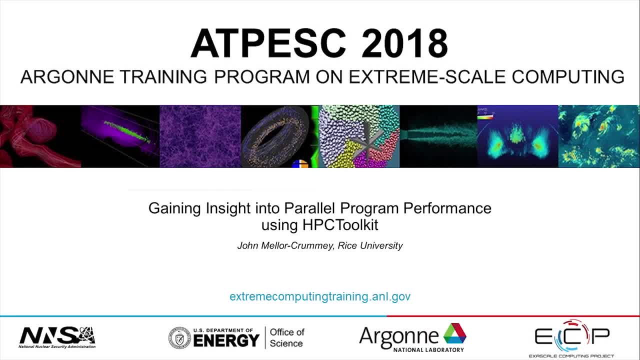 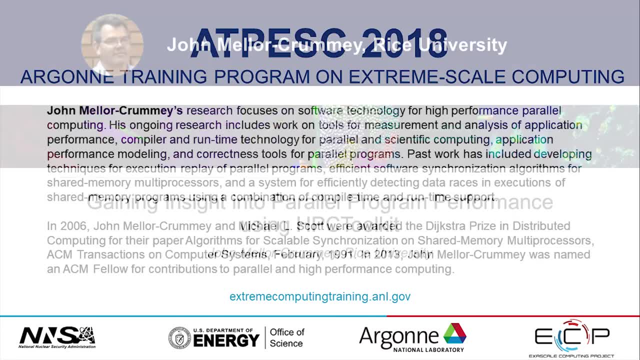 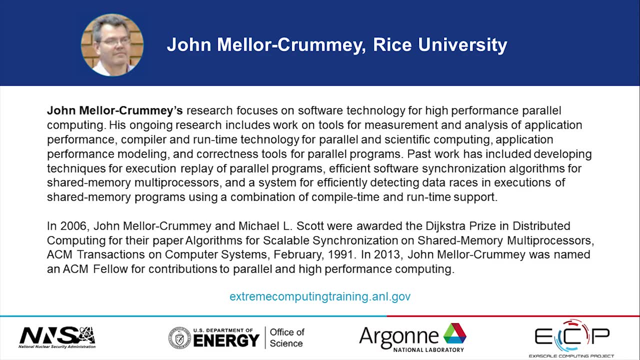 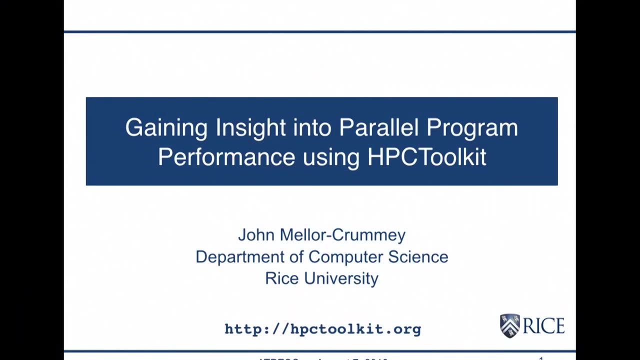 Hi, John Miller-Grummey. I'm a professor at Rice University in the computer science department. My focus area is high performance computing, and the thing that my group is working on mostly these days is actually building this tool that I'm going to talk about- HBC Toolkit. 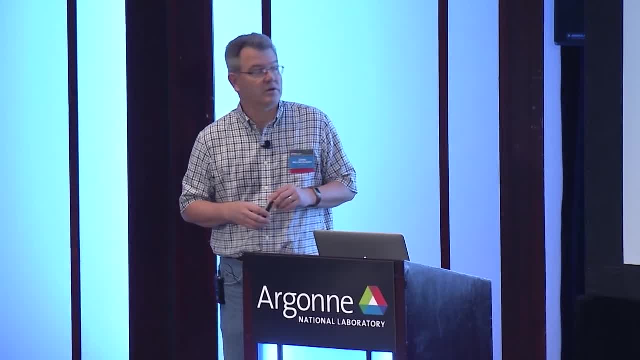 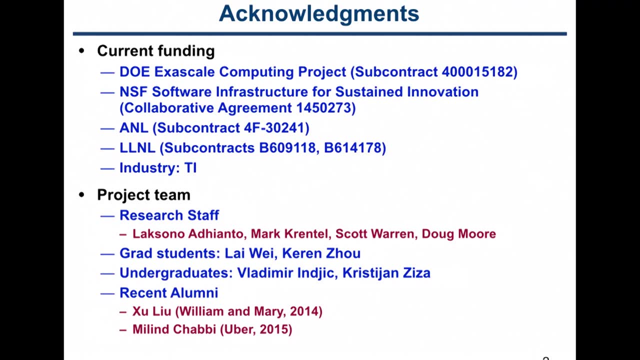 So I'll begin with an obligatory funding announcement. We're supported mostly by the DOE Exascale Computing Project. We also have some funding from the National Science Foundation, a subcontract from Argonne and one from Livermore, And this is not just my work. This is the work. 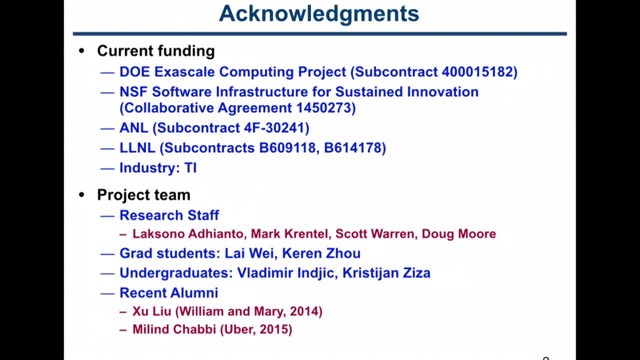 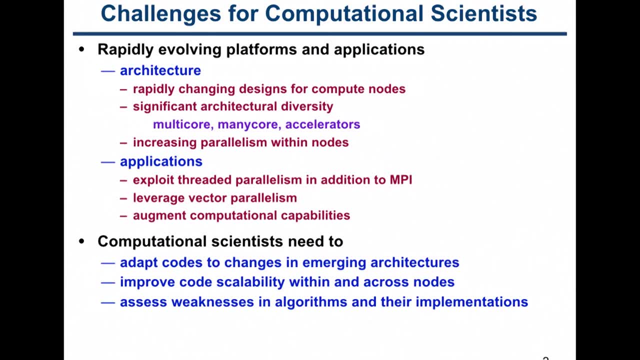 of my research group, which includes four PhD research staff and a number of students. So for computational scientists like yourselves, one of the biggest challenges is that these platforms that you're starting to use are rapidly evolving, that there's been a shift from multi-core to many-core, and also there's a big push to move to systems with accelerators. and so the machines that you're starting to compute on will not be the ones that you finish computing on, And there's also increasing parallelism within, And then you're also going to be working to improve the scalability both within and across nodes, in order to get the most out of these. systems, And to do so, you'll have to assess weaknesses in your algorithms and their implementations as impediments to scalability, And so I would argue that performance tools can play an important role as a guide in this process. So some of the challenges that you have for performance analysis are that these architectures have very complex nodes. You have multiple levels of parallelism in that you have multiple cores. Each core has instruction-level parallelism inside it. The cores typically have short vector units, SIMD parallelism And then on some of the systems like on Titan or the, 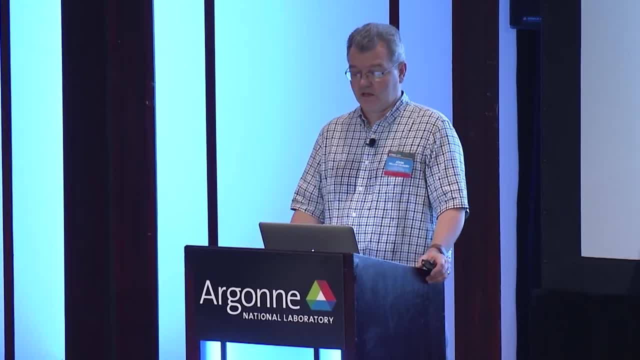 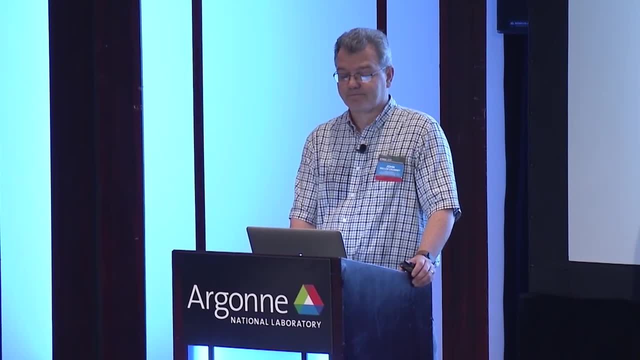 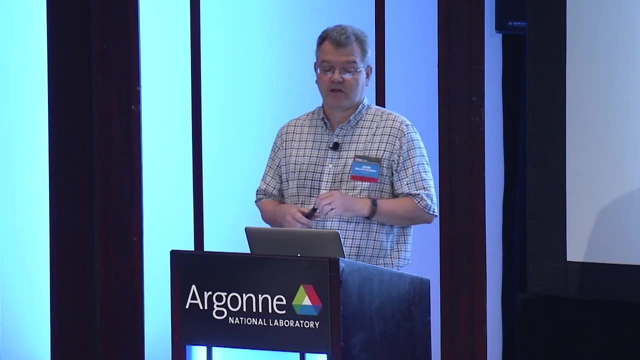 emerging systems. at Oak Ridge, the Summit system, or at Livermore, the Sierra system. you have accelerators on them. There's a multilevel memory hierarchy. I don't know. I think in the architecture session you probably talked about cache and memory. As it turns out, memory is about 300 cycles. 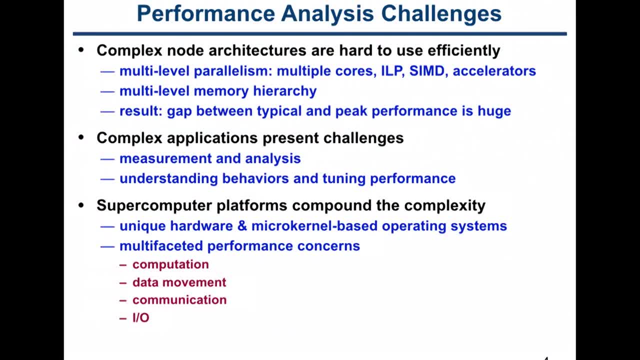 away, and cache is just a few cycles away, And if you're not making the most of the memory hierarchy, then you're running at the speed of main memory, which is much slower than the processors, And so, as a result, the typical gap between the peak performance and what 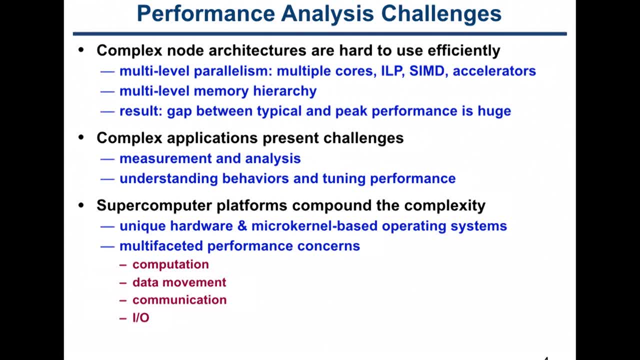 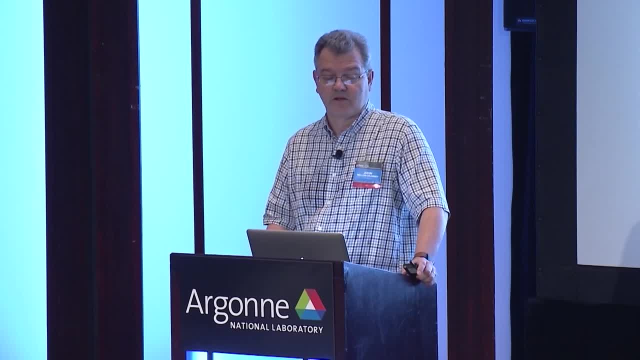 you achieve is huge, And so, if you want to try and get the most out of this system, you have to invest a little bit of effort into figuring out what's the mismatch between what your application is doing and what the architecture is capable of, and then doing a little adjustment. 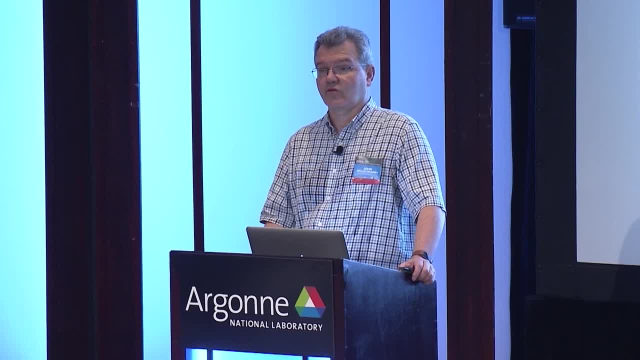 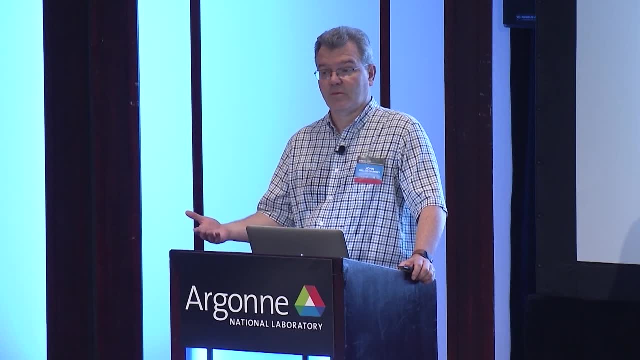 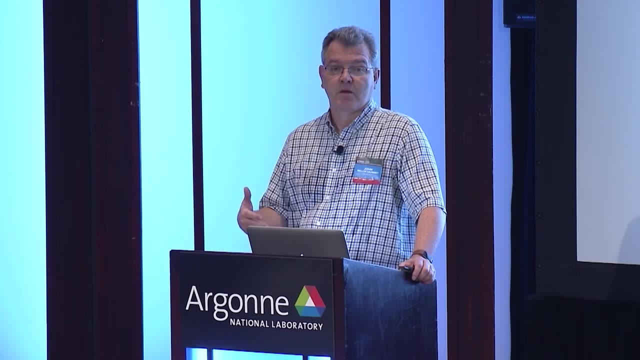 And so for us, from the tools perspective, complex applications present challenges. There are challenges for measurement and analysis, also for understanding the behaviors of your applications and tuning the performance. And on these supercomputers that you're starting with there's additional complexity. So on the BlueGene system, there's unique microkernel-based 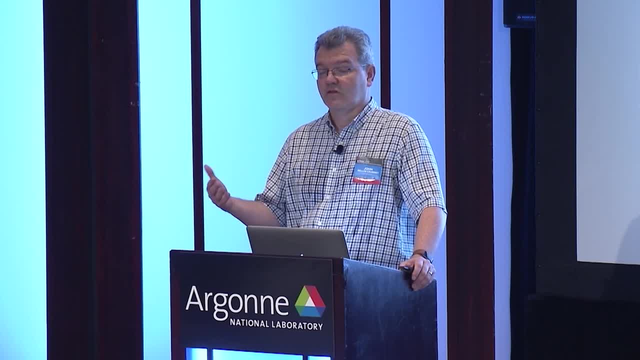 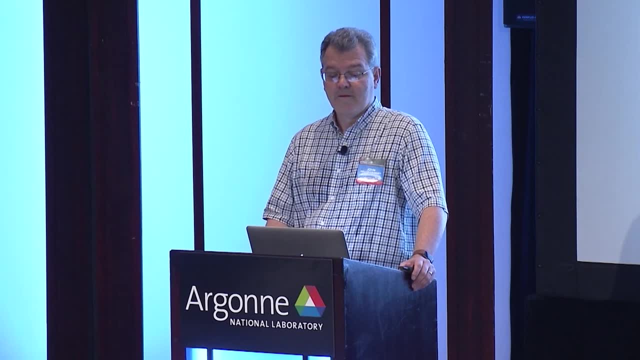 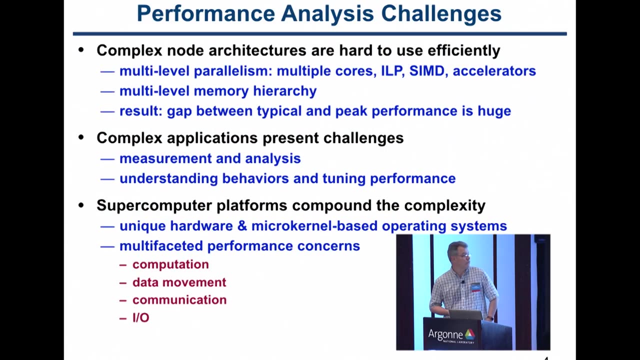 operating system, not just stock Linux, And your performance concerns are beyond just computation. You're interested in optimizing data movement and communication and IO. if you're trying to get the most out of these systems, So what? I would argue that you want. 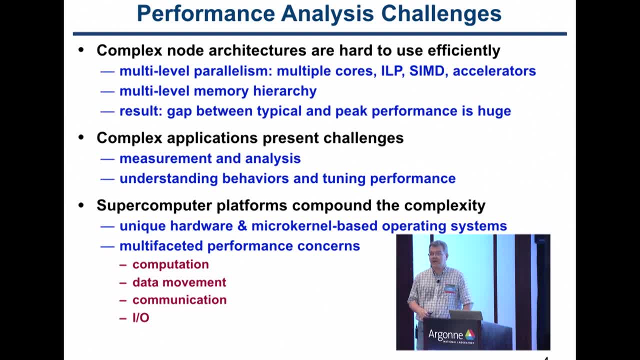 is. you'd like a multiplatform programming model, independent tools, whether you're computing using MPI or whether you're computing using partition global address space model. that makes the system look like a giant shared memory machine. to the first order, You'd like to be able to use the same set of tools and you'd like to use this, whether you're computing. 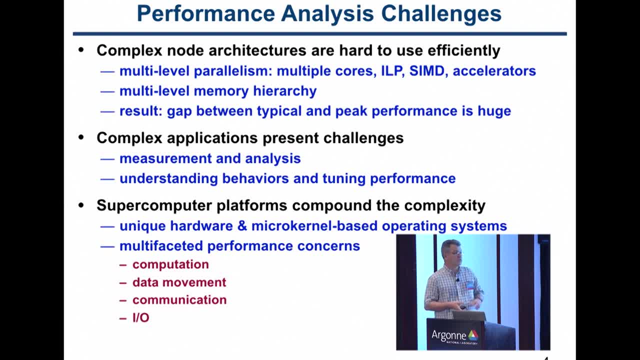 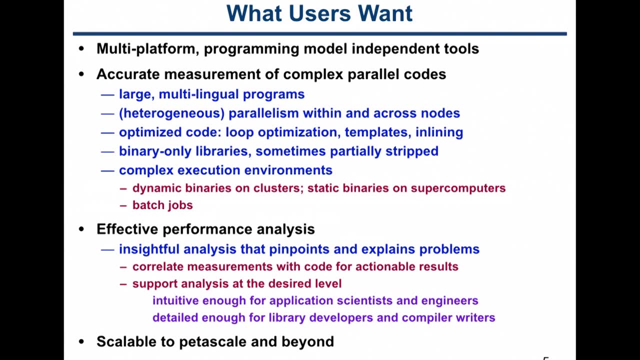 on something with an Intel-based architecture or something with IBM processors in it, And you want to do accurate measurement of complex, parallel codes. So your programs are often large and multilingual. What we see in codes from the National Labs is that sometimes they have a C++ framework but they've got computational kernels in Fortran. There's parallelism both. 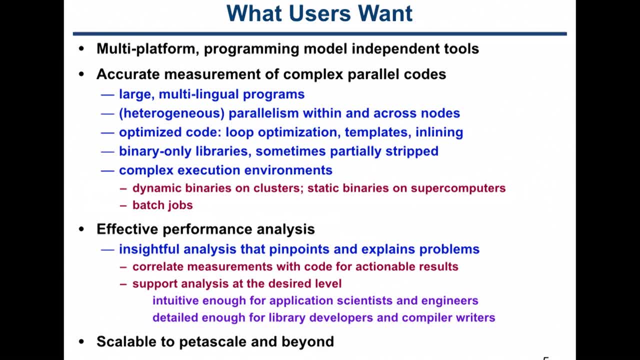 within and across nodes, So perhaps OpenMP within the nodes and MPI across the nodes, And sometimes the parallelism within the node is heterogeneous. You've got accelerators, You've got optimized code loop, optimization done by the compiler, inline templates, inline. 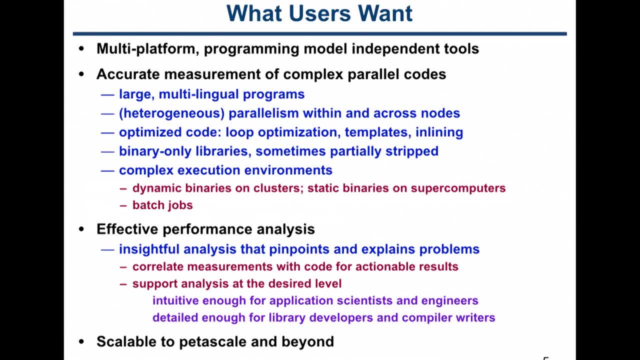 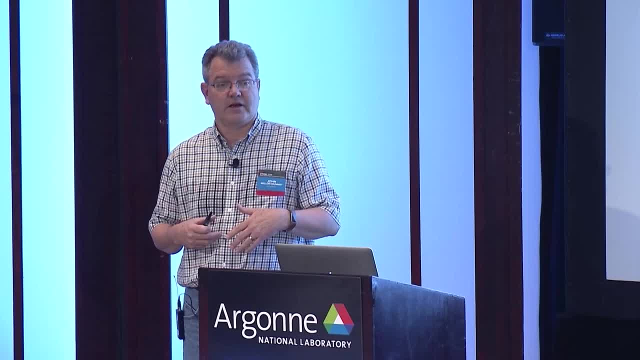 functions, And then something that we have to live with is that often, many pieces of your environment are available only in binary form, And so this might be the vendor's OpenMP library or libcuda from NVIDIA, if you're using accelerators, And on these systems we also. 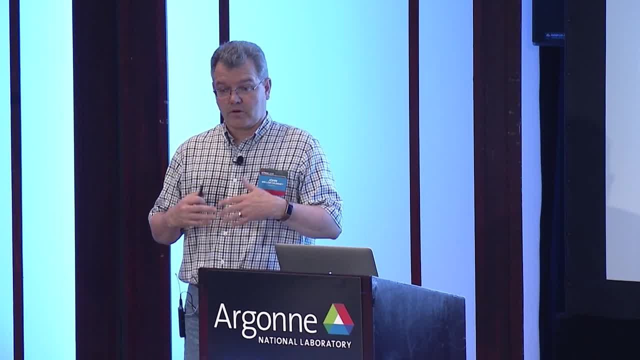 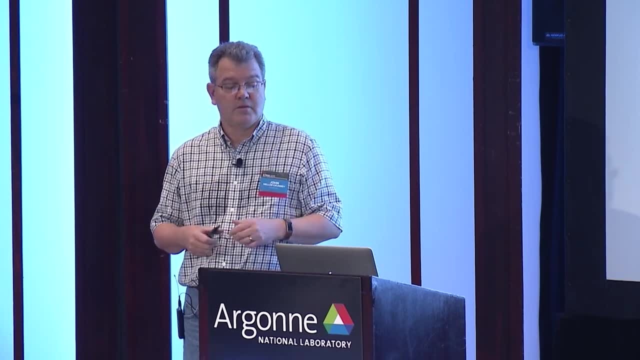 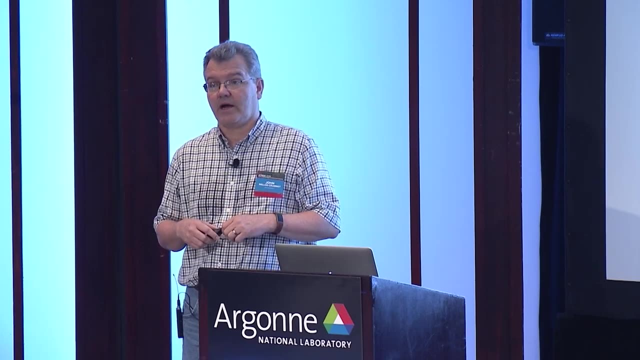 have some complex execution environments And sometimes binaries are dynamically loaded, which means that when you compile them, there's external references to things like the C library and the math library. When you compile things on Theta and Mira at Argon, typically you're. 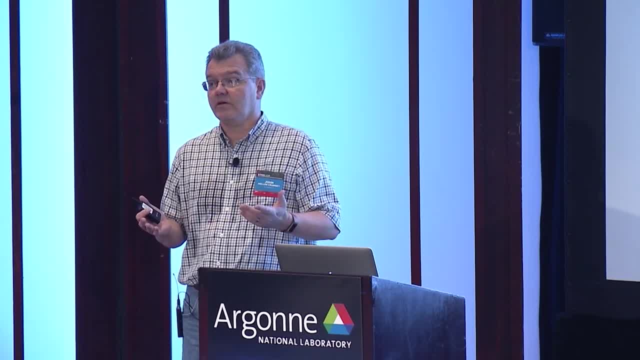 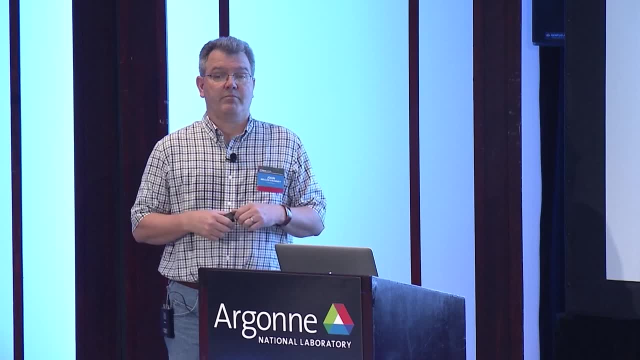 producing static binaries which contain everything that your application needs. But our tools are built to use on either dynamic binaries or on static binaries, And so if you're using it on your cluster at your institution, then you would probably use it on dynamic binaries. 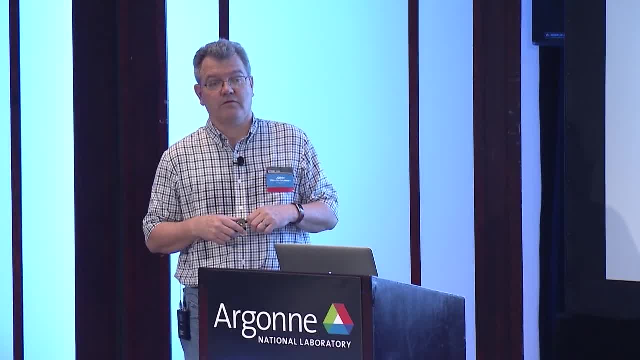 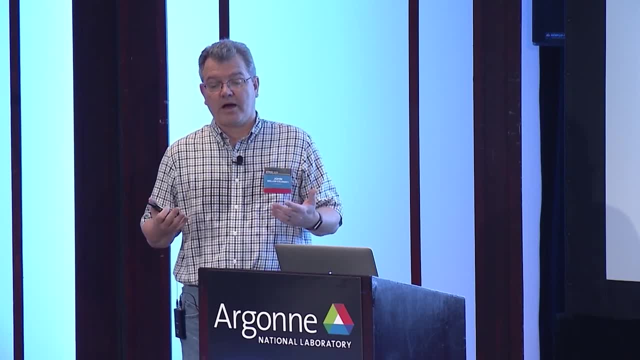 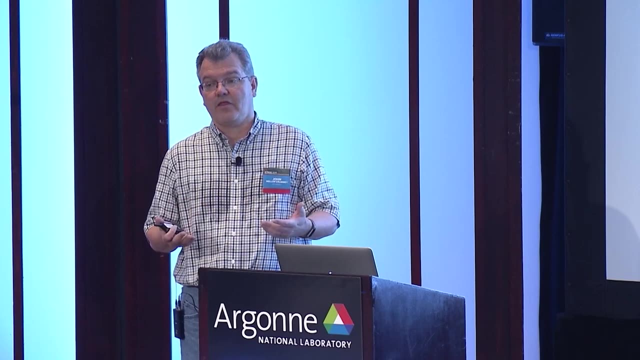 So what we've built are some tools for effective performance analysis, And the goal is to provide insightful analysis that explains what the problems are And correlates the measurements with the code, Rather than just having a picture that says your performance is terrible. what we want to be able to say is, on line seven of 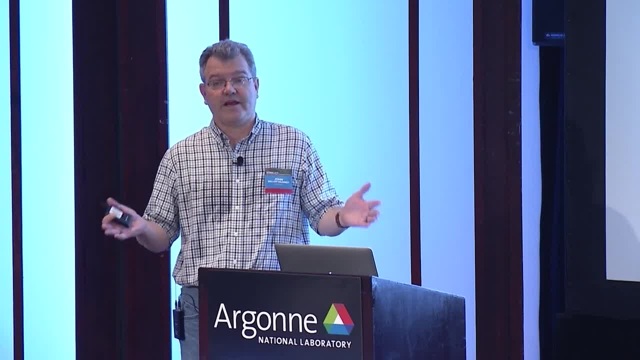 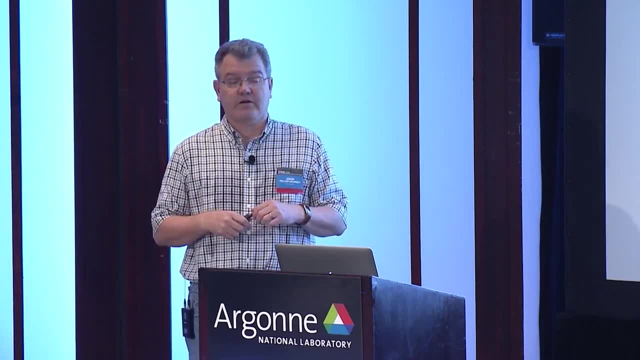 the following file, you have a problem, And that's costing you a 25% scalability loss, And so associating the performance losses with the code is actually an important part of the tool, And so, then, our goal is scalable to petascale and beyond, And I think there's. 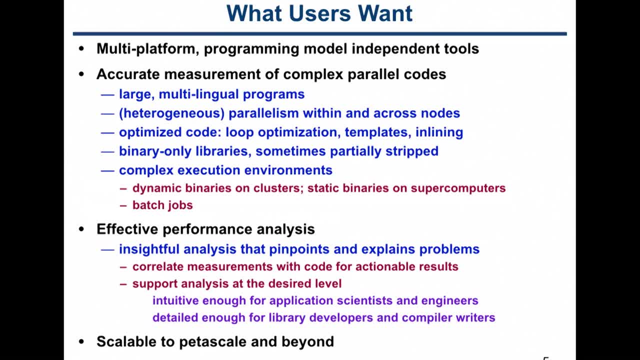 still some challenges in scaling our tools, And that's what we're working on right now. We're working on the exascale project. So I'll start with an overview of HPCToolkit And then I'll show you some demonstrations on how we use it to pinpoint scalability, bottlenecks, understand behavior, applications over time. 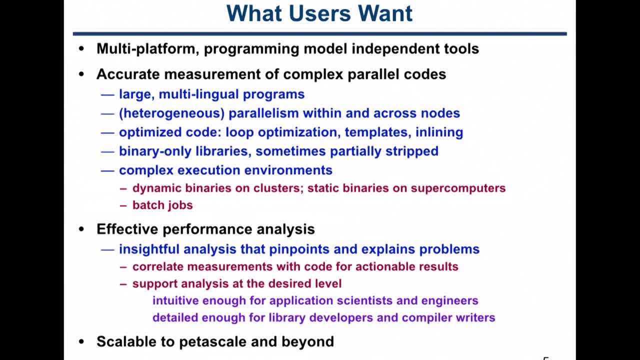 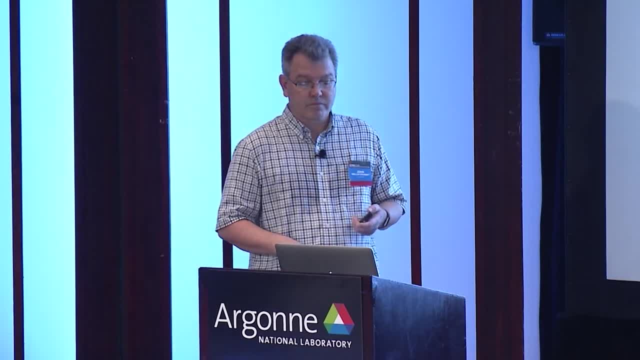 how we can use it to understand process variability or thread variability, understand OpenMP performance and then a few final remarks. I'll see if I can fit all that in in the remaining 32 minutes. So HPCToolkit employs binary levels. 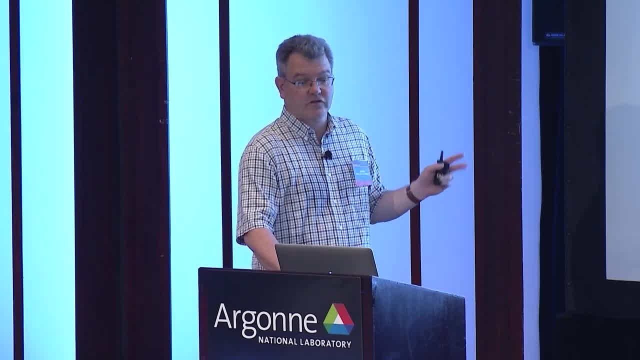 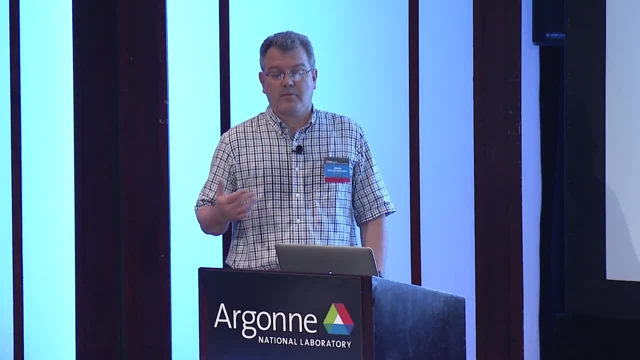 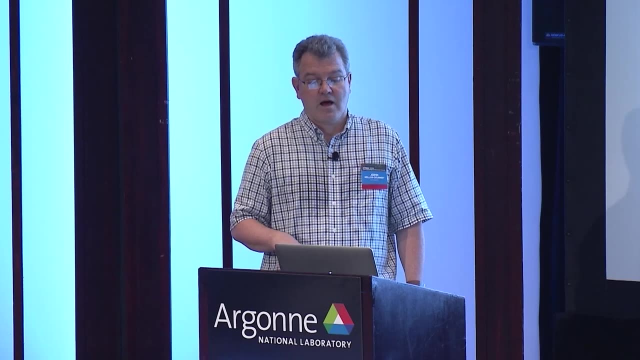 Binary level measurement analysis, So we're observing fully optimized binaries, which might be dynamically linked or statically linked. We're supporting multilingual codes with libraries that are potentially available only in binary form. HPCToolkit uses sampling-based measurement, And so what that means is that the overhead is controllable. You can set the sampling. 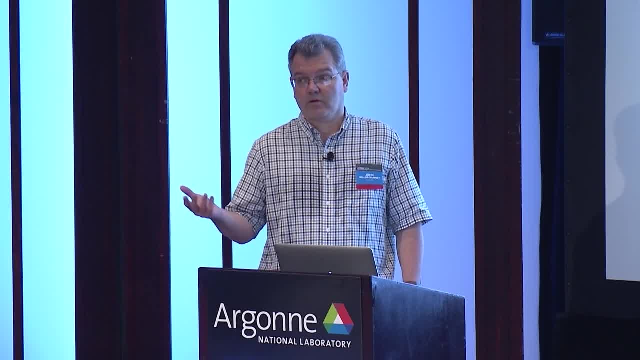 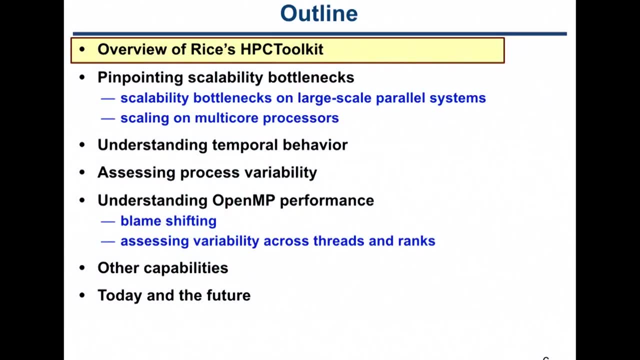 frequency and that determines how often our tool is making measurements in your application And what sampling does is. it minimizes the number of times that a tool is using a binary level measurement And that's because it optimizes the blind spots in your application. So if you're rewriting, 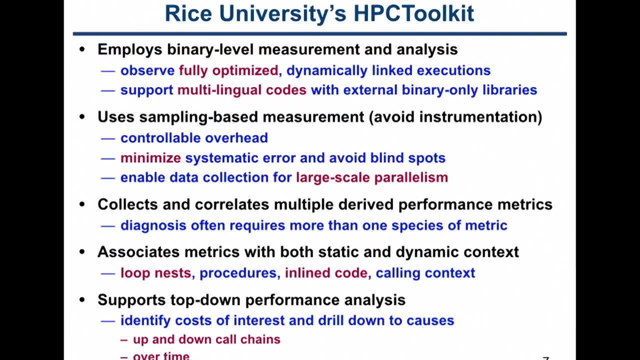 your code and adding instrumentation at function entry and exit, and you do this for all of your user code, but then you link against a whole pile of libraries. you might miss all the performance information in the libraries, And so our tool just says: you link your application the normal way and we'll make some measurements. 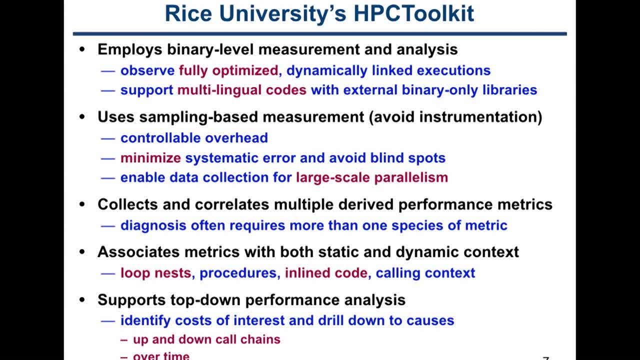 as it runs, and we'll measure the code wherever it came from, whether it's in libraries or whether it's linked directly into your application. So what's this? It's called the HMI. So with our tool, you can collect a number of applications. 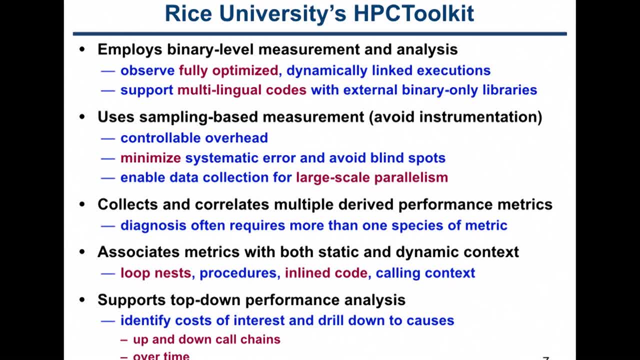 and correlate multiple derived performance metrics, So sometimes one metric is enough. If I told you you had a billion cache misses, that's kind of meaningless. What you need to know is: well, how many accesses to the cache did I have? Or if I told you you executed for a billion cycles. 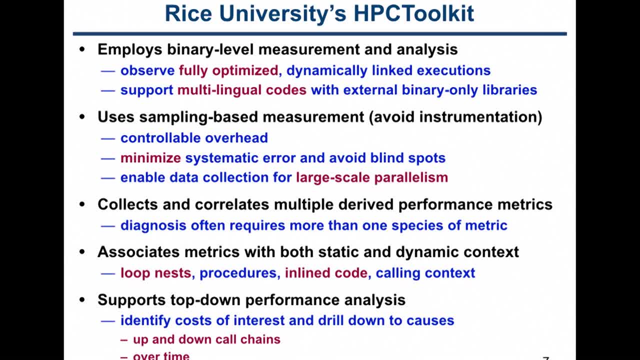 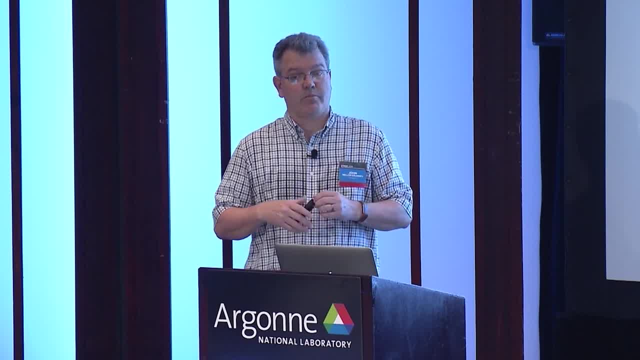 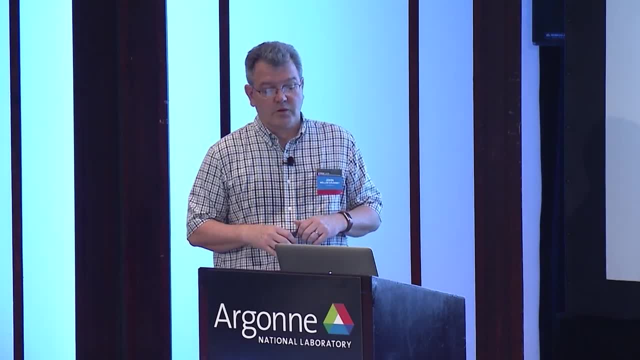 then you might wanna know: well, how many instructions did I complete, Did I waste my time or did I compute productively? And so often that requires having measurements with multiple metrics and then you can compute, derive metrics using the metrics that you measure. 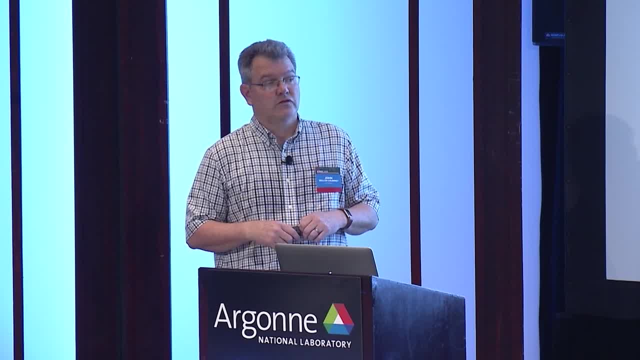 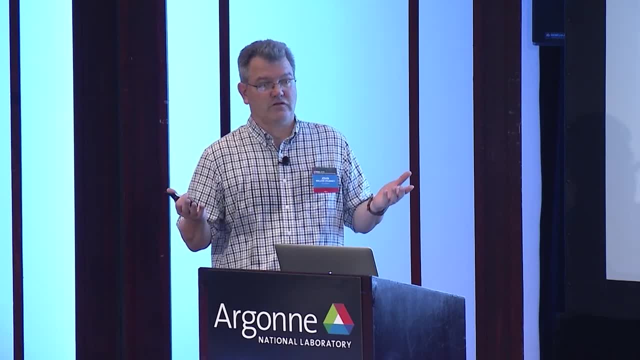 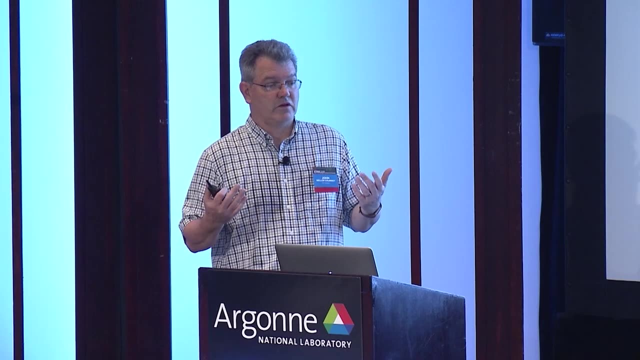 We associate metrics with both static and dynamic context. By static context I mean with procedures and with loop nests and with inline code, And then dynamic context, I mean call chains, okay, And so if we see that time is spent in MPI weight. 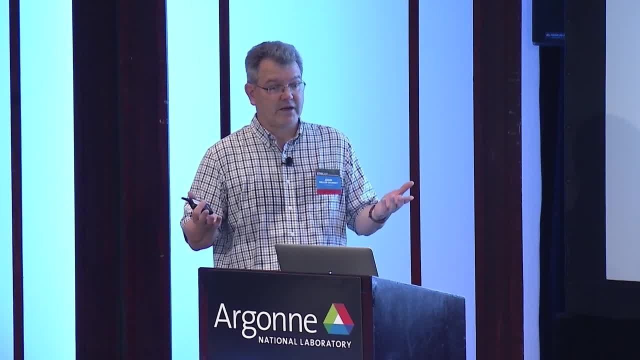 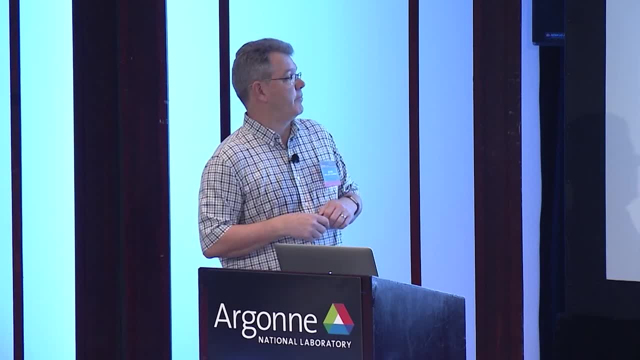 in something like a coupled climate code. then you need to know whether it's whether you're in MPI- weight in the atmosphere portion of the code, or the ocean part of the code, or something like that. And then, finally, our tool supports top-down performance analysis. 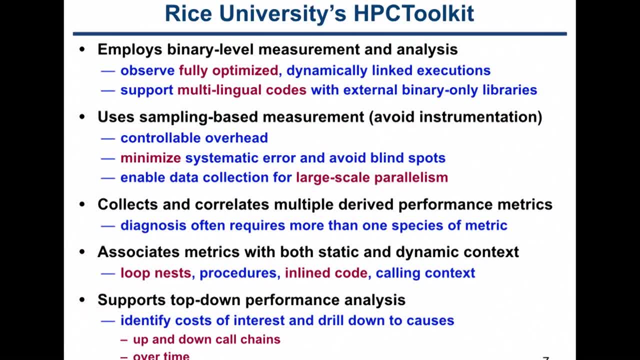 So you can identify what you're interested in and then drill down and focus on the causes. So here's a little schematic for the workflow for using our tools. So in the first step you compile and link And for dynamically linked executables on Linux clusters. 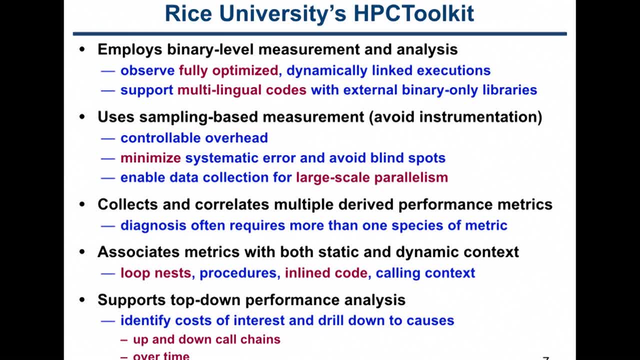 you don't do anything, You just use your makefile- Makefile's exactly the way they are On Cray and BlueJeans systems that are statically linked. then what that means is you actually have to add our HPC link command as a prefix to your link line. 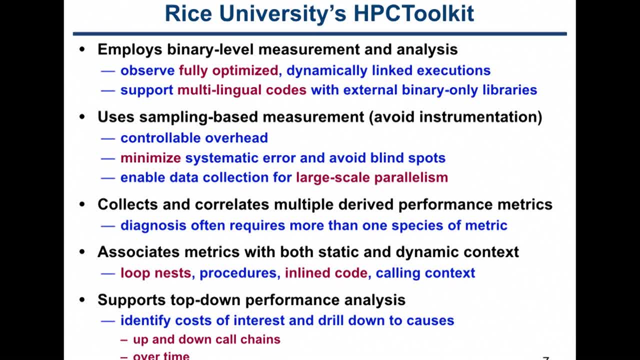 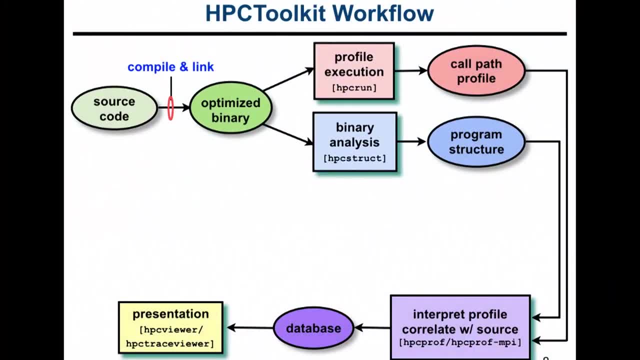 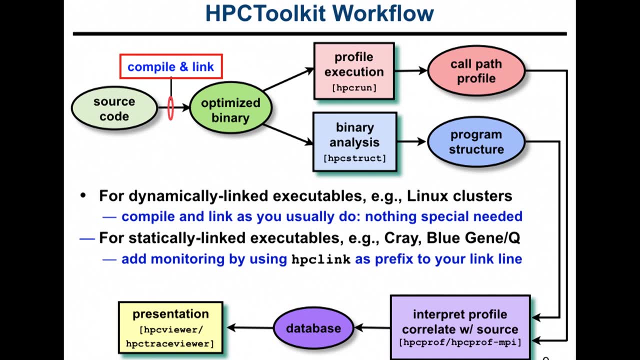 So if you have an entire command that performs your linking, you just say HPC link in front of it, And what that will do is it'll inject our monitoring library into your statically linked execution, And the second step is profiling the execution, And so you launch your optimized application binaries. 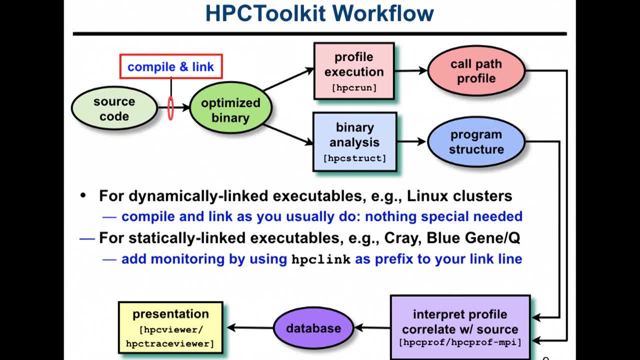 For dynamically linked binaries. you launch them with our launching script, HPC run. So you would say, HPC run my application, or MPI run, HPC run my application. Or however you launch MPI. whether it's with Slurm or with Cobalt, there's a way for launching. 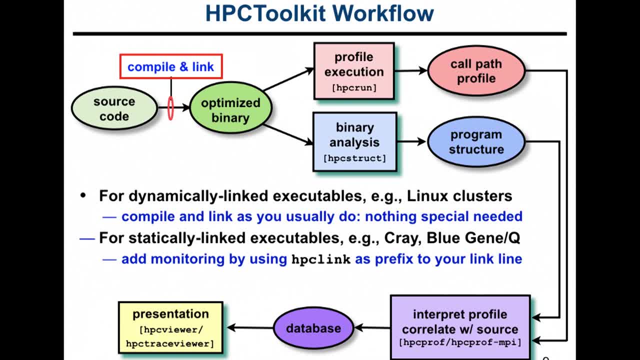 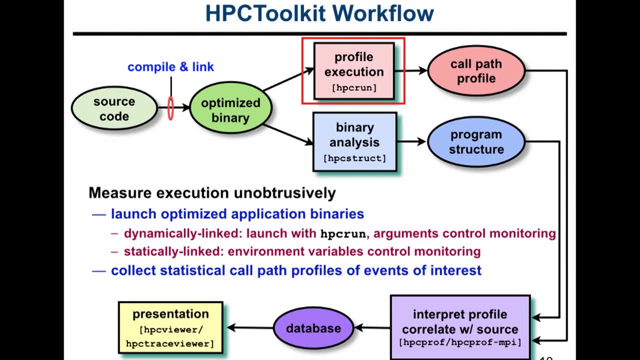 your MPI applications And instead of just launching the application itself, you say: HPC, run my application. HPC, run the application For statically linked binaries. so on Mira and on Theta, you actually use statically linked binaries and so you don't use our launcher script. 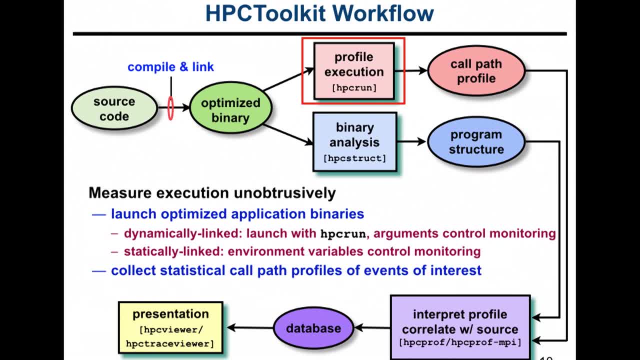 And what that means, then, is that all of the settings that you wanna pass into to control the monitoring, you pass in as environment variables And then, when the application is running, we're collecting what we call statistical call path profiles, And what that means is that, when the application is running, 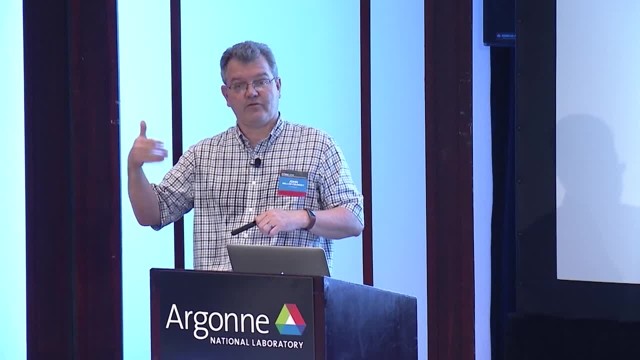 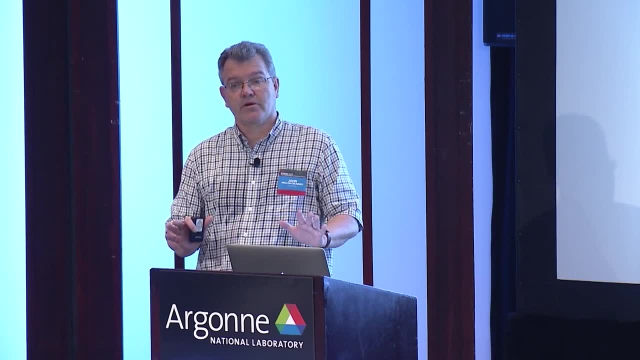 it's going to be able to measure and attribute costs in context and of the events of interest. So what I mean by that is we're going to measure and attribute costs in context, And so you can use either a timer to interrupt the program. 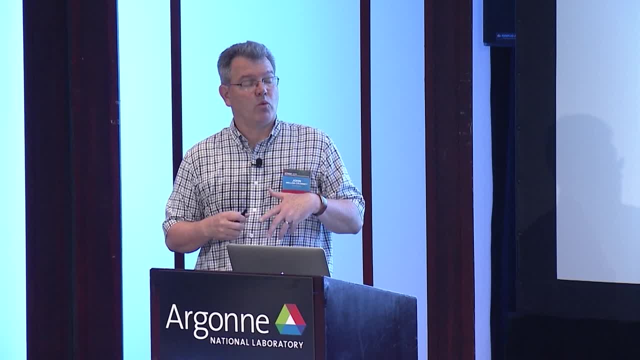 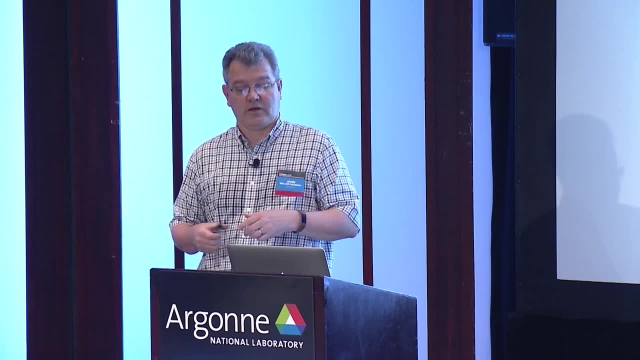 periodically. or you can use a hardware counter and say: I want to know where I spend my cycles, or I want to know where I execute instructions, And so I can say: I want to have a counter based on cycles and I want it to periodically interrupt my program to find out. 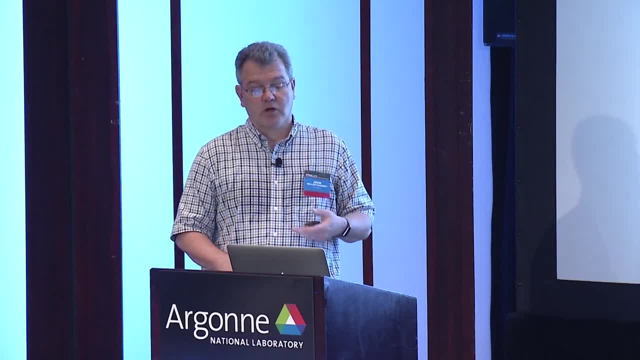 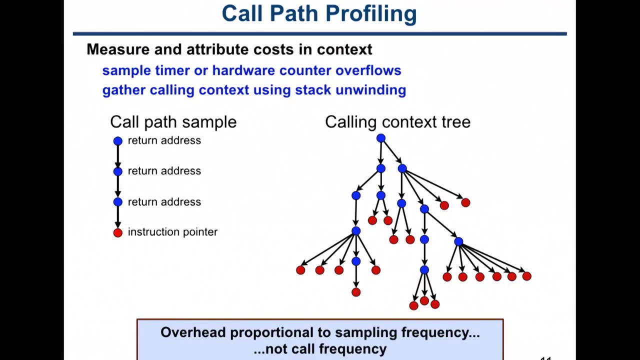 where I'm executing. And then every time you run your application, every time this timer goes off, you'll be at a particular instruction. You'll be at an instruction pointer. And so let's say I'm in a routine C when called from B. 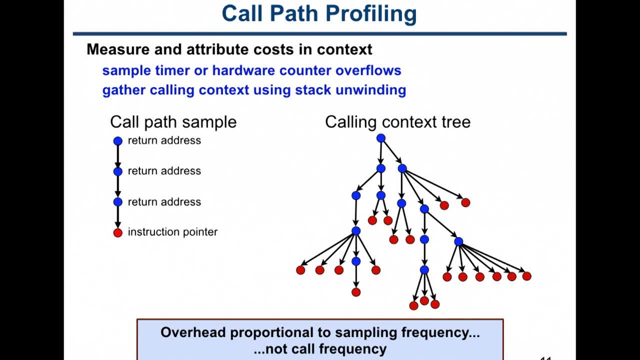 when called from A, when called from main, And so what we will do at runtime is we will unwind the call stack and find out where you were and how you got there. Okay, so if I'm in MPI, wait, I know how I got there. 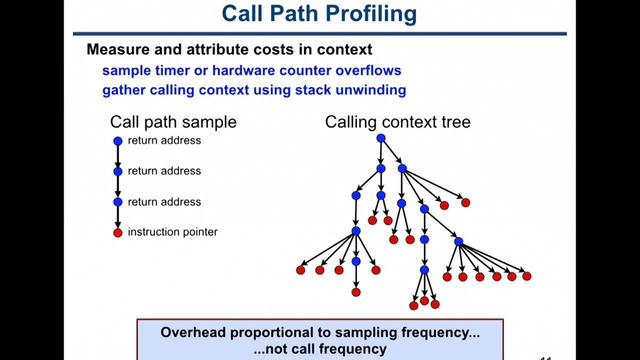 And this is just for one interrupt where the sample timer or the hardware counter overflows. So what we're going to do is we're going to unwind the call chain And then, as the program executes over time, we're going to keep unwinding the call chain. 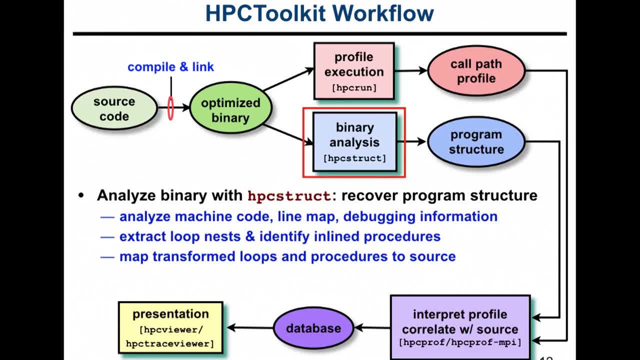 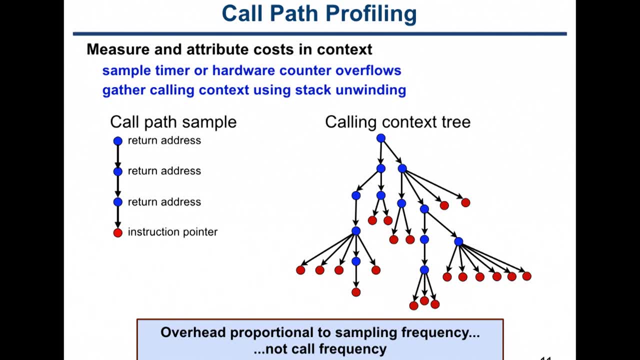 and we're going to fit all of these things together into a tree, And so, conceptually, at the top there's something like main, And then a subtree over here might represent the solver, And then there might be an initialization phase and some sort of post-processing. 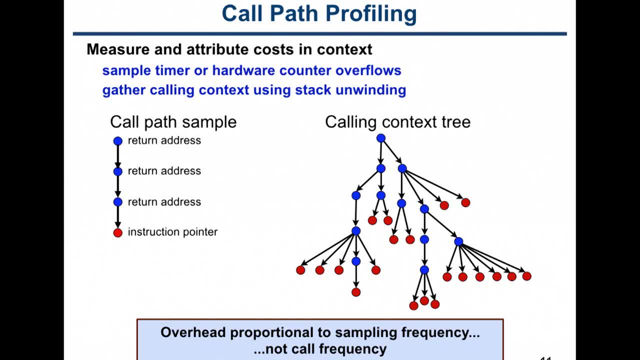 phase, and they each have kind of their own context within the tree, And so the result of our monitoring is actually this tree with weights at the various nodes, And the weights indicate how much metric was measured at that point, And so the metric might be cache misses, or it might be cycles or time. 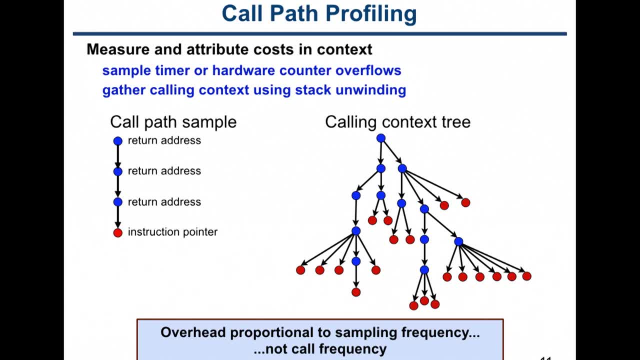 And so the important point about this measurement technique is that the overhead is proportional to the sampling frequency, not the calling frequency. Okay, you get to say so right now. if you're using this on theta and you're using the Linux perf measurement subsystem, then you just say: 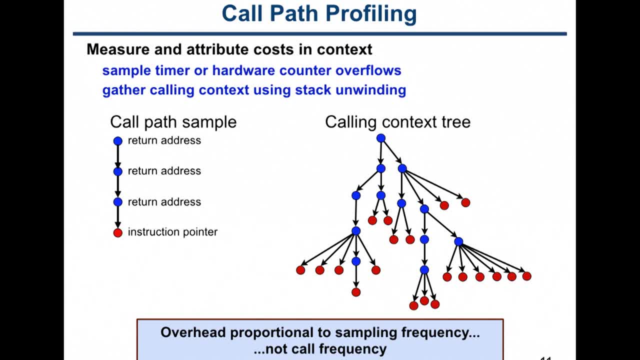 I want to measure with cycles, And then perf will figure out exactly how often it should be interrupting your application, And so it's aiming for about 300 samples per second, per thread. Okay, so now we've launched the program, we've measured it. 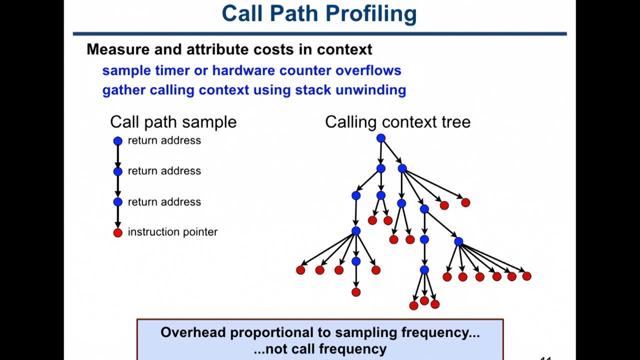 we've collected these calling context trees. The next step is now. we want to interpret our data. So what we have is a binary analyzer called HPC struct, And what this does is it recovers program structure and associates it with addresses- machine code addresses in your application. 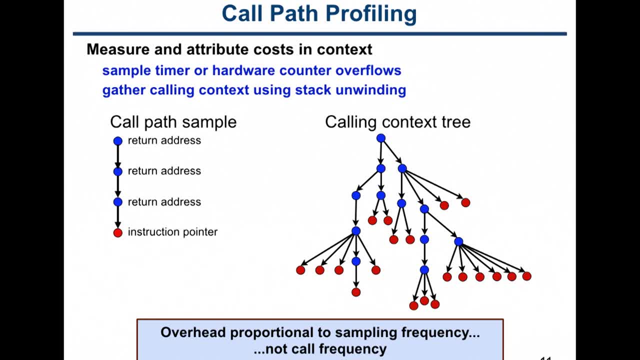 So when we're measuring your application, we're measuring everything in terms of instruction addresses and return addresses inside your application. And now what this HPC struct utility does is: it analyzes the machine code, it parses the machine code, it identifies branches. 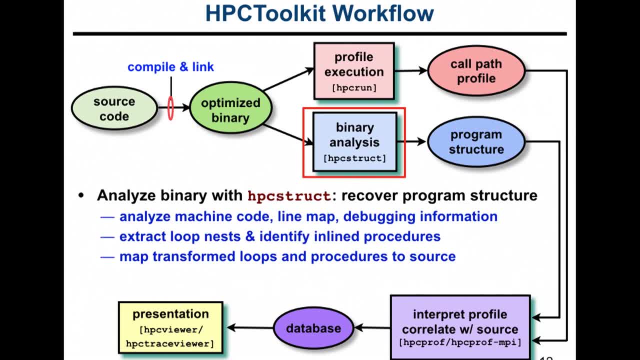 it identifies the branch targets, It reconstructs the control flow, builds a control flow graph, analyzes the control flow graph to find out where loops are. And then we take this information about loops and we combine it with a line map and with whatever information we got from the compiler. 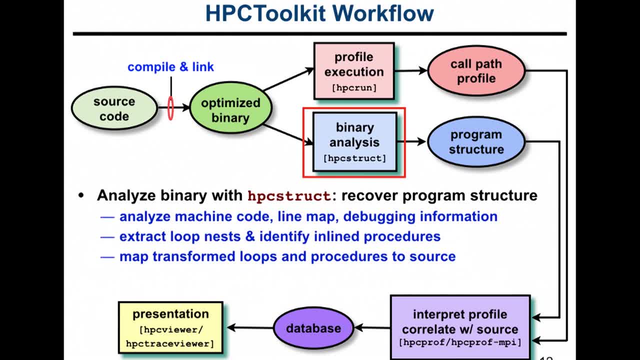 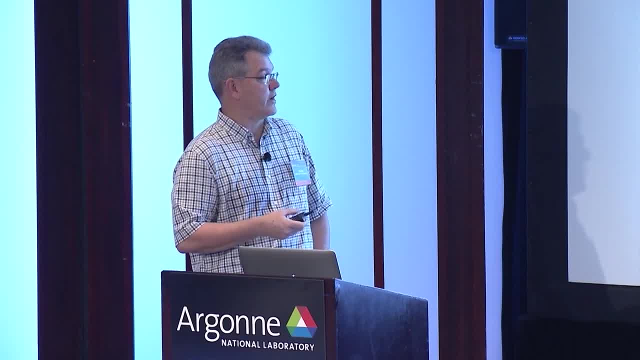 about inlining and we assemble loop nests and information about inline procedures And then we map everything in your optimized binary. we map it back to the loops and procedures that were in your source code. So if your loop has been torn into several pieces, 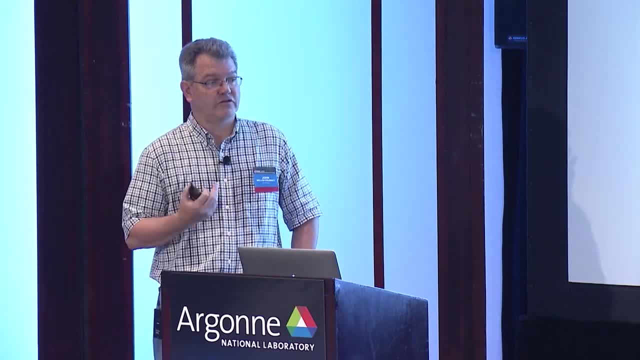 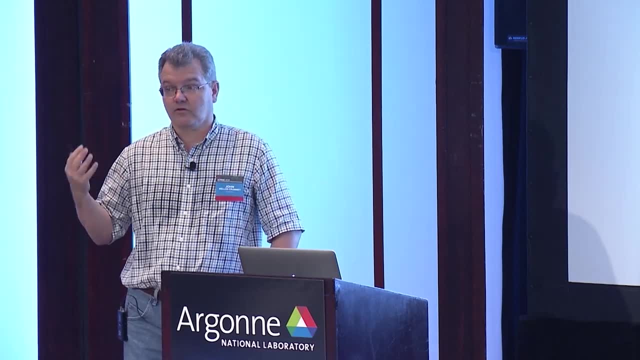 when we're reporting the performance information, we're just reporting it all back to the same source lines that you had present in your application, And so this is pretty unobtrusive. You just say: analyze my binary, and you don't really have to know. 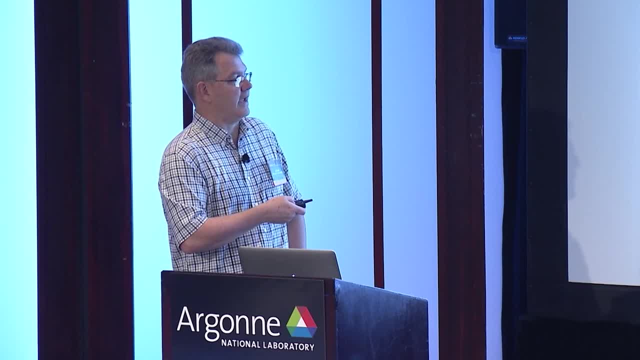 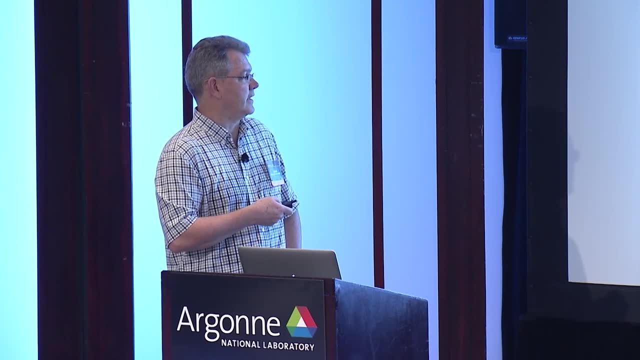 You don't have to worry too much about what happens inside here. Then the next step is: once we've collected our call path profile, our dynamic measurements, and we've analyzed the binary, then we use a tool that combines these two sets of information. 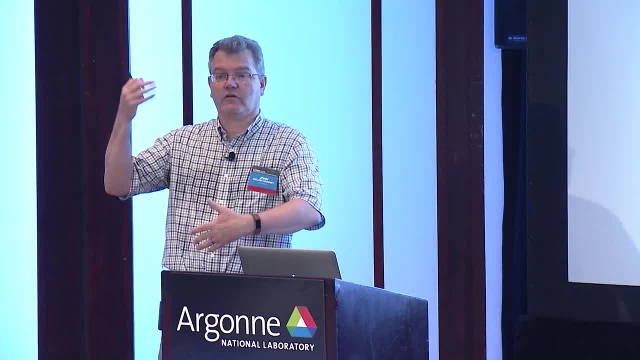 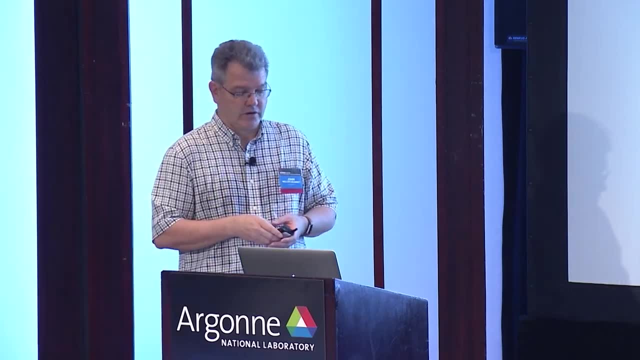 So there's HPC prof, which is a tool that can be used on the head node of these clusters to analyze small amounts of information, say from a few threads or a few processes. If you want to analyze information about a large execution, then you use HPC prof- MPI. 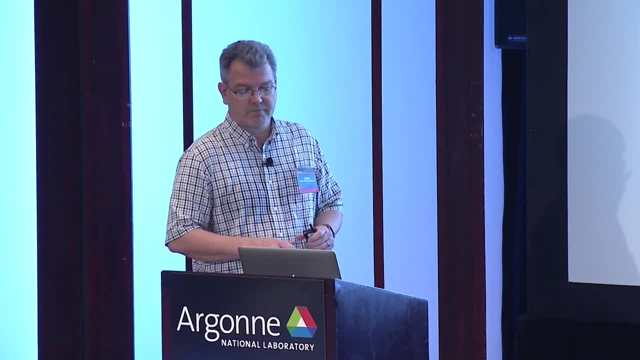 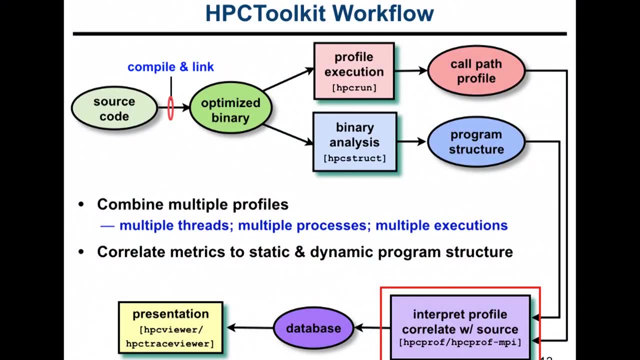 And this in itself is an MPI program. And so if we have profiles from hundreds or thousands of threads and ranks, then you use HPC, prof, MPI to say: scoop up bales of these things, analyze all the performance data and assemble it all into a unified view. 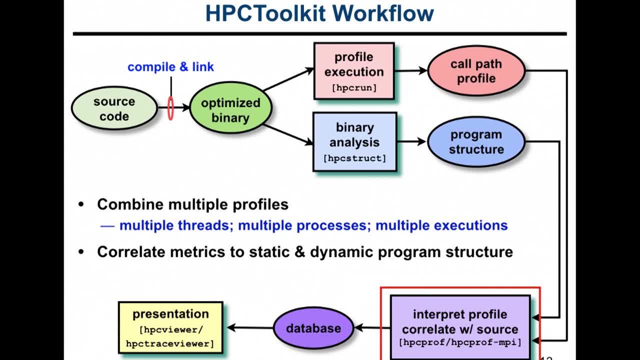 And then what the interpretation tool does is it produces what we call a database. It's really just a directory with different kinds of files in it. And then the presentation tools. well, there are two. So one is a source code-oriented view and the other is a time-centric view. 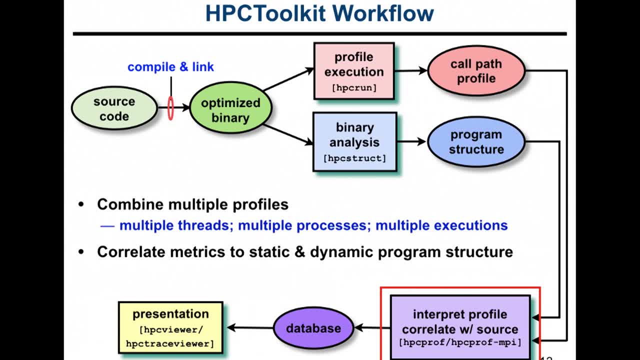 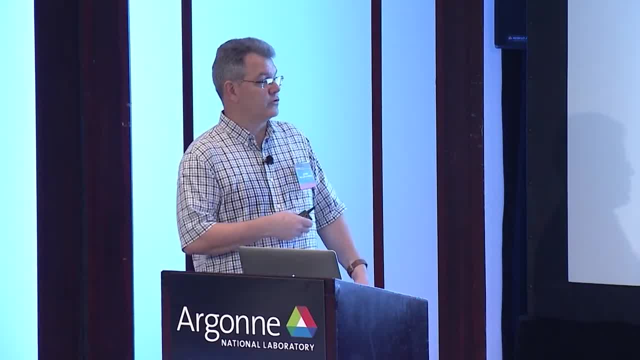 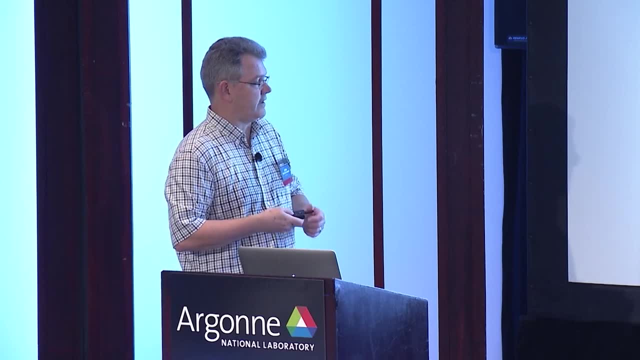 And so these tools enable you to explore the performance from multiple perspectives, to rank, order the metric that you think is important and then compute derived metrics to help you gain insight, like scalability, loss, graph the thread metrics over the context and then explore the evolution of behavior over time. 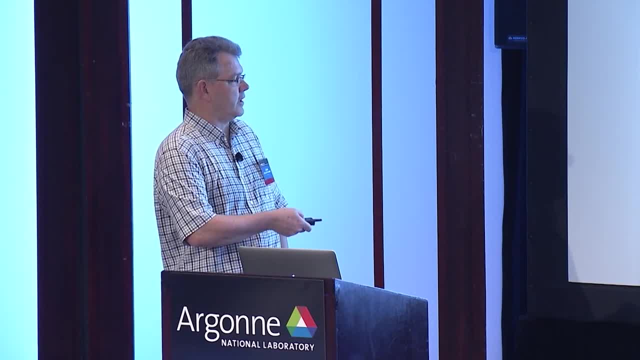 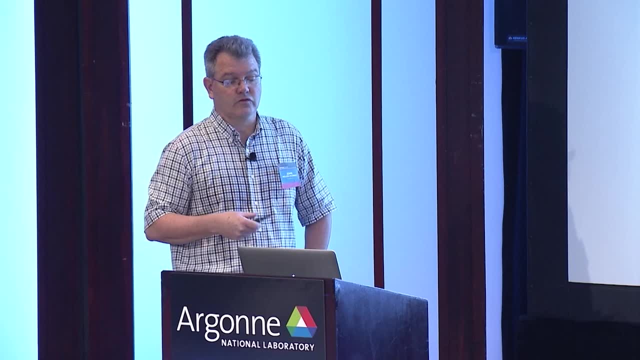 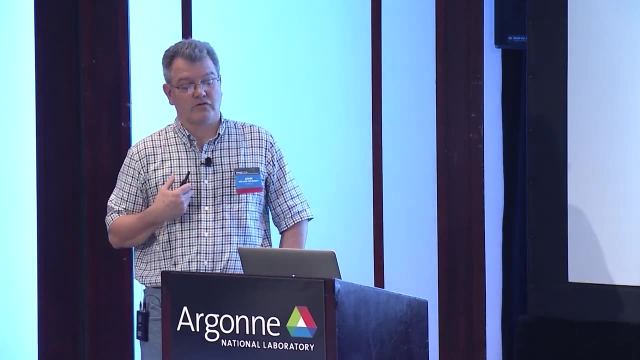 So here is our code-centric view, And it looks rather simple, but it turns out that it's simple by design and you can use it to analyze measurements on a large number of threads and ranks, And so what we have here is: there's the metric pane. 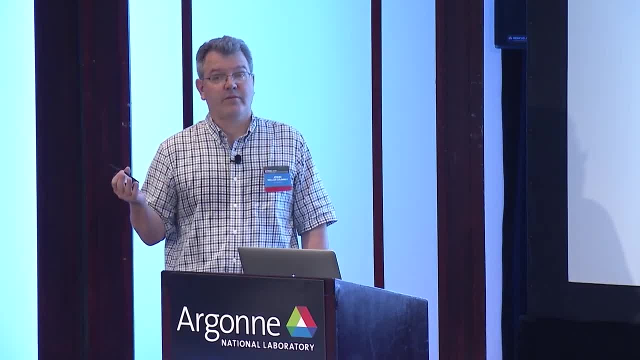 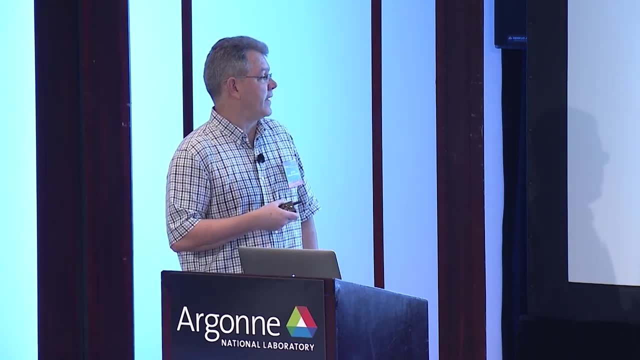 which is whatever we measured. So in this case we're measuring time, And there's inclusive time and exclusive time. So exclusive time is the amount of time I spent in a function, And then inclusive time is the amount of time I spent in a function or things that it calls. 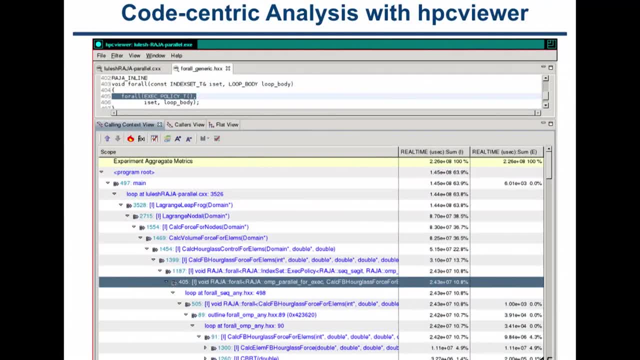 And so you can think of the inclusive time as being like a top-down view, And then the exclusive time is: what did I do here? And then we have this navigation pane, And so over here you can click on various places in the navigation pane. 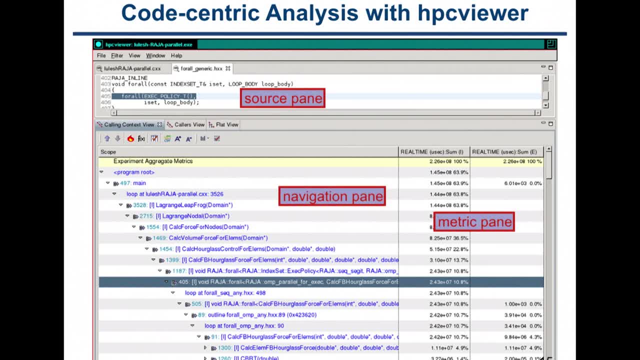 So if I clicked on this function, then it'll bring up the source code up at the top. Here it's showing for the highlighted line. it's showing the source code in the top view, And what's interesting about this is that there's a couple of different ways. 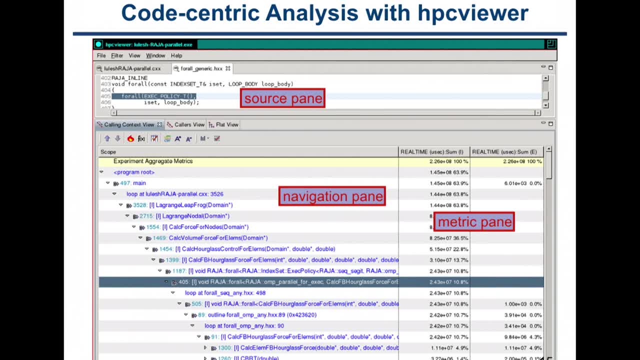 that you can look at your application performance. You can look at it in this top-down view, what we call the calling context view, where you're looking down complete call chains, The caller view where you're looking at your performance. to say, 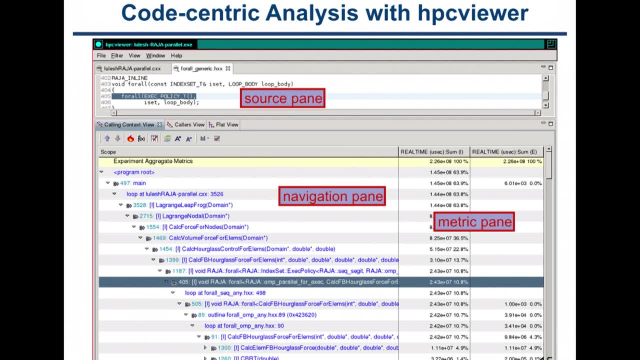 okay, I spent my time in some function like memcopy. How did I get here? So I can look up call chains to find out how I got to memcopy And if I spent 50% of my time in memcopy I can trace down to each call site where I came from. 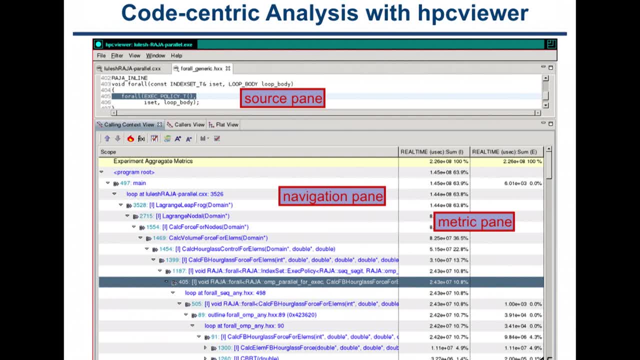 how I ended up spending that much time in here. Then there's the flat view, which you can use to just say: well, I want to look at a particular piece of code and I don't care how I got here. I just want to know how much time or how much cost was incurred here. 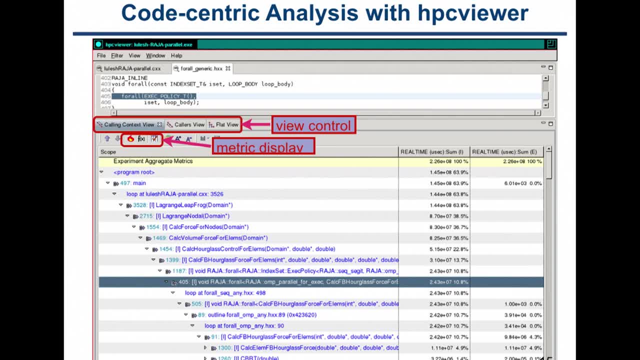 And I can look at the loop nests inside my procedure and decide which ones are important or not. And then there's a couple of metric display options. So the flame button is one of my favorites. You just point at something here and then you hit the flame button. 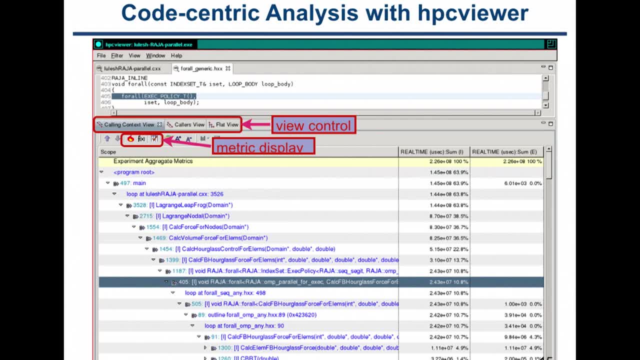 and it will open up call chains and show you like what the most important thing is, And so the rule is: if I open up something and there's some child that accounts for 50% or more of the parent's cost, then you keep on going. 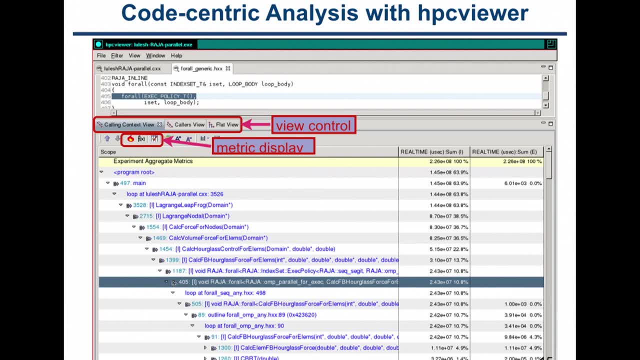 And I can point at anything along the way, Anything in here. I might click close with a triangle and then point to some sibling and then hit the flame button again to explore some alternate path. And there's a button here. F of X for computing derived metrics. 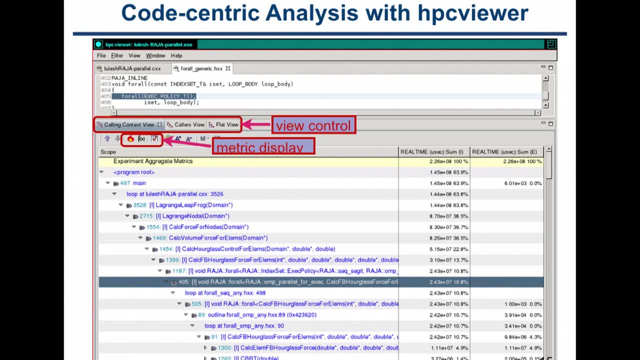 So it will bring up a little pane where you can key in spreadsheet-like formula and I'll show you how to do that. And then there's a column chooser. So if you collected actually multiple metrics, you might decide that for now I only want to look at one or two. 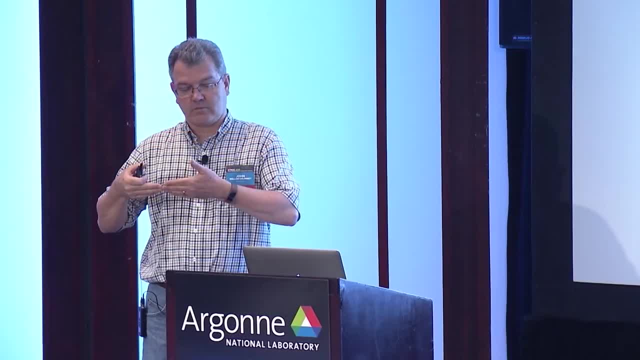 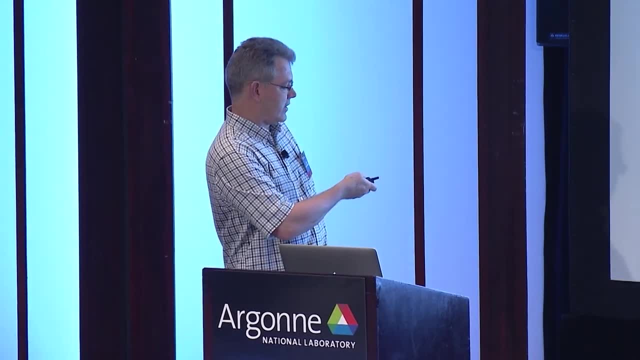 and just sort of hide the rest. so I'm not horizontally scrolling a lot, And so that's convenient as well. So an interesting thing about this pane is that while this looks like a call chain, in fact only the things marked in blue are actual calls. 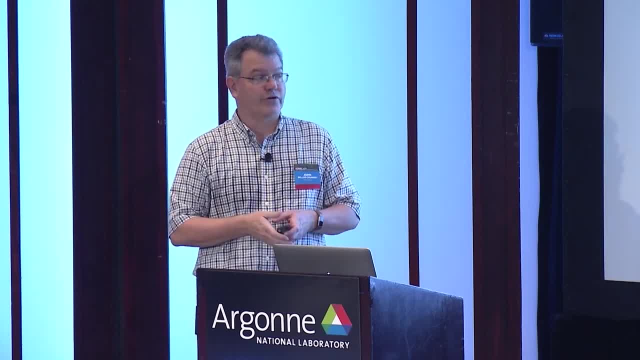 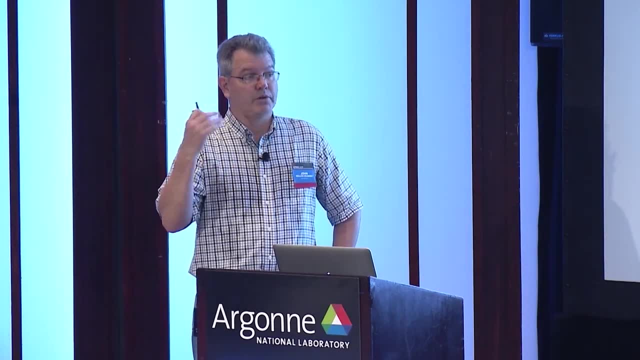 And so inside here there's information about a loop. This information about a loop we're not getting from the source code. We're getting this from looking at the application binary and looking at analyzing the machine code and looking at the mappings back to source code. 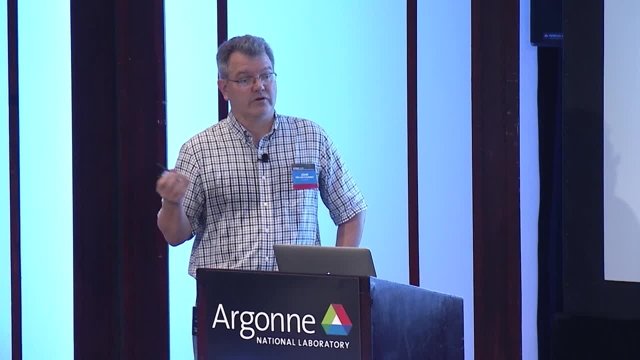 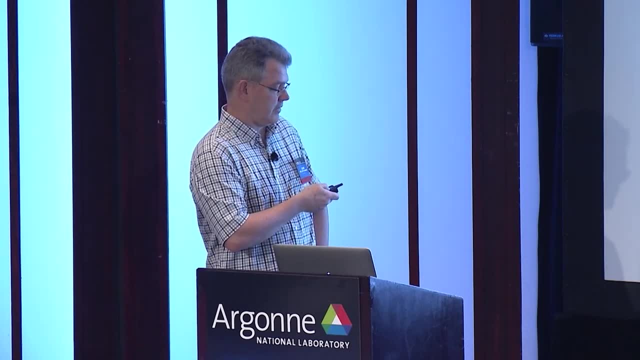 And then here it shows calls to inline functions and so this bracket I bracket designator indicates that this is inline and this says: at line 3528 there's a call to an inline function And then inside that inline function, at this line number, 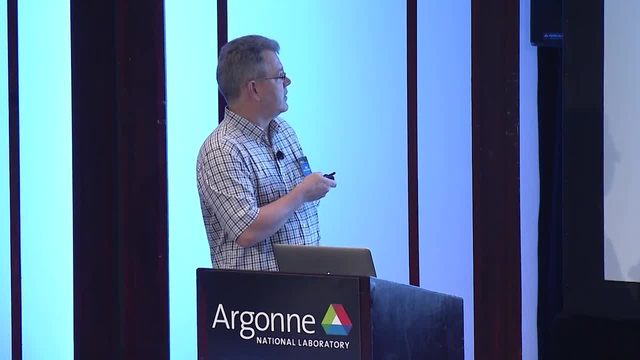 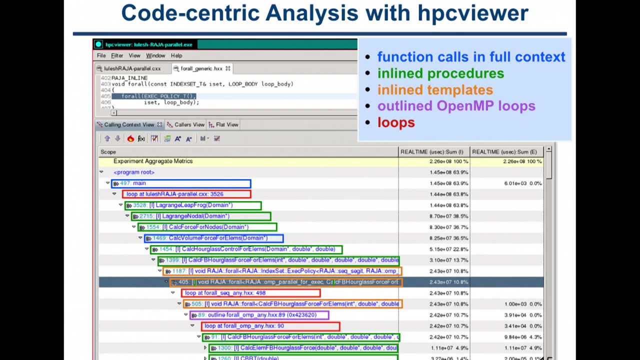 there's a call to an inline function, And I know that you talked about Raja and you talked about Cocos the other day. In fact, here is Raja templates: a Raja for all template. We can see how the template expands. 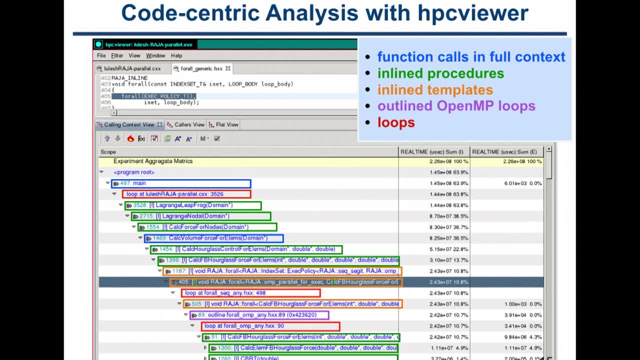 Inside the template. there's a loop Inside that. there's another inline template- Raja for all outlined- a call to an outlined OpenMP function, a loop inside that and some calls inside that, And so what you really get to see is the full context. 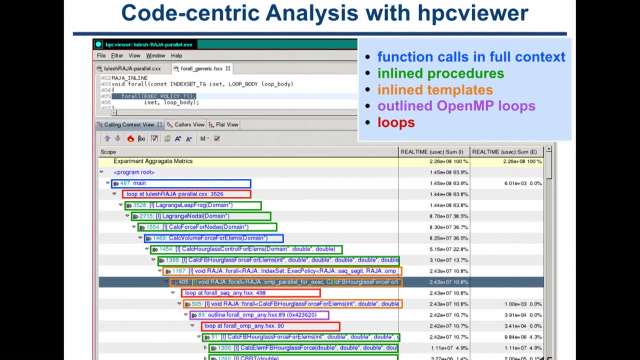 in which your performance measurements were incurred, And so this works for C++, it works for Fortran, it works for C or any mix thereof, And so for C++, where you're using inline functions and templates, it's really crucial to be able to see these additional layers of context. 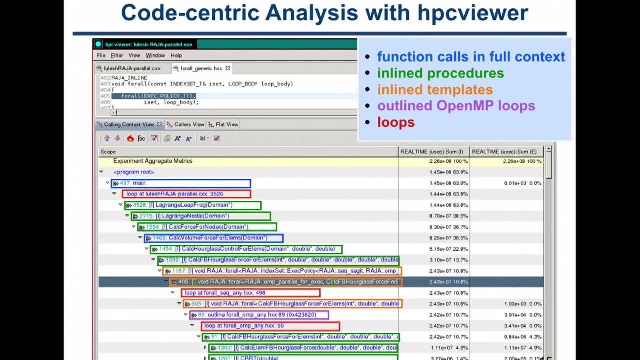 because if I was just told I had a call to this function from inside main and that's the way the compiler left it, I'd have no idea how it got there. Okay, so why are we here? We're here for large-scale computing. 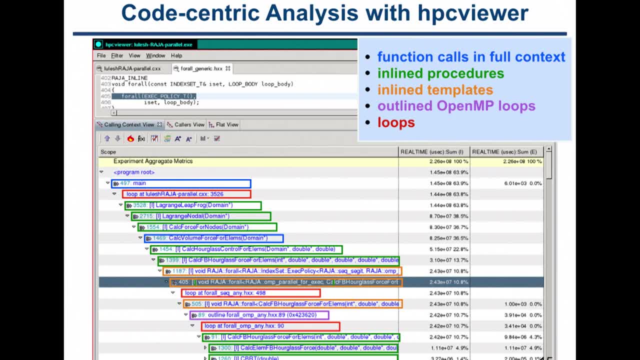 And so on these large-scale systems. as you run on larger numbers of processors, what happens is, instead of getting the full benefit of all the processors or a parallel efficiency of one, your efficiency drops off, And so that when you get out to a large number of processors or cores. 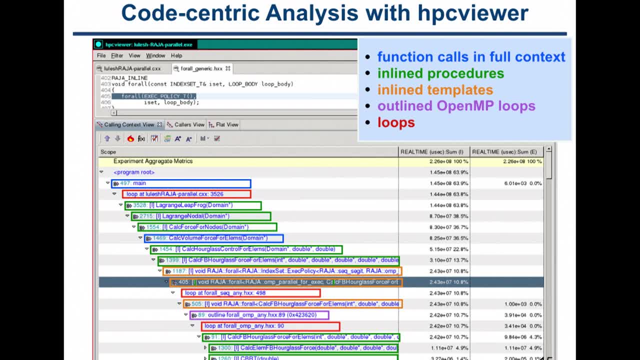 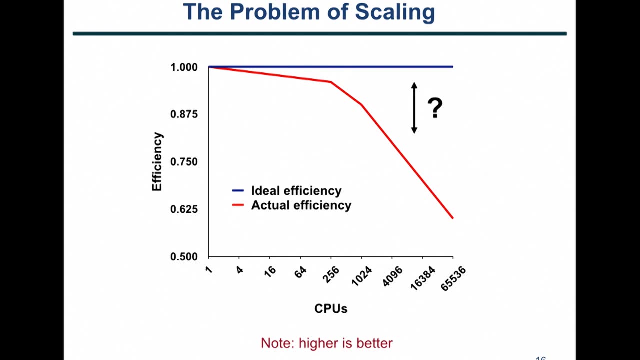 instead, you're only getting about 50% efficiency or 15% efficiency on the machine, And what you really want to know is what caused this efficiency to drop off? That's the question we're setting out to answer. So the goal here is that you have some sort of automatic scalability analysis. 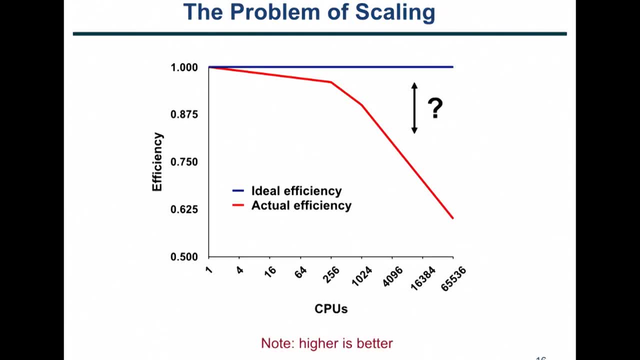 You want to pinpoint your scalability bottlenecks, guide the users to problems and quantify the magnitude of each problem. Ideally, we'd also like to diagnose the nature of the problem. Well, I can say that we have. the first three are under control. 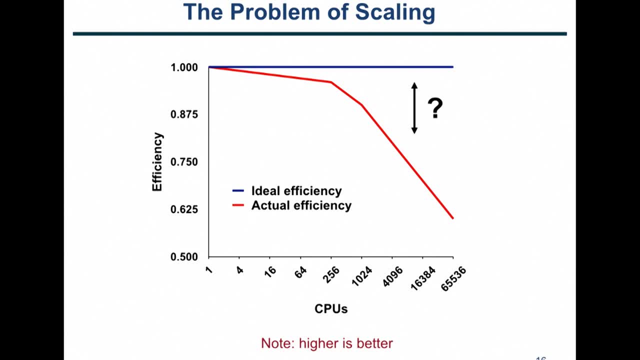 The last one is up to you, Because the nature of the problem, it might be your data structures, it might be your algorithm, and so we can tell you the problem is here, but then you have to figure out what to do about that. 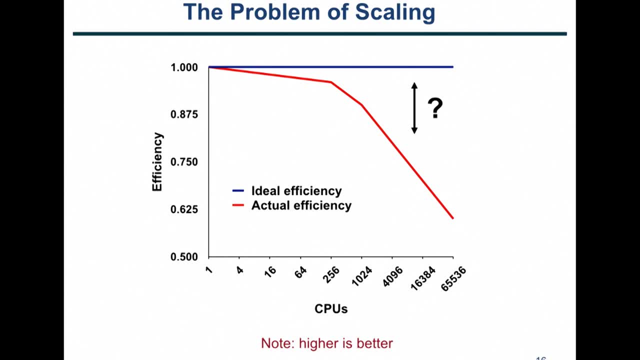 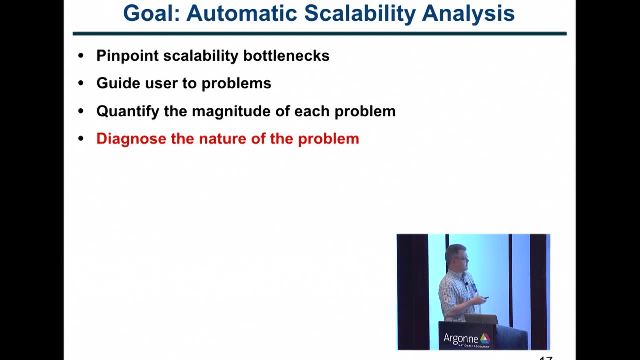 And I can show you an example in just a moment, and it'll be clear why we can't tell you exactly what the problem is. All we can do is say the problem is here and it costs this much. So as an example, let's use 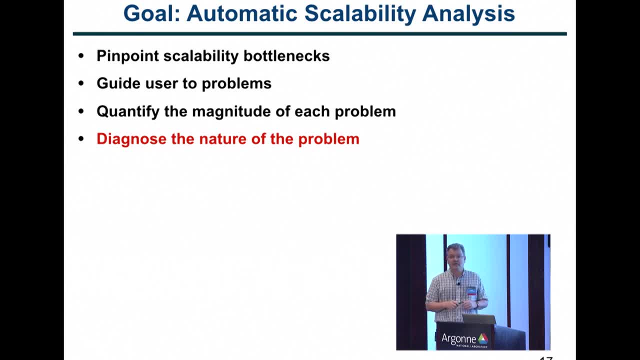 a climate code, And so modern software has many layers of libraries You might have. your application is using the Petsy library, is using the MPI library- underneath The MPI library, is using the C library to perform memory copies and things like that. Your performance is often context dependent. 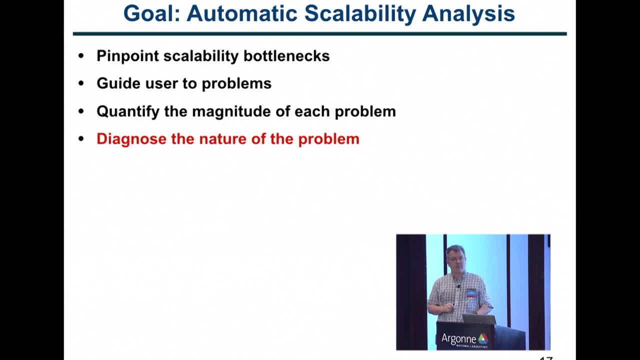 And so earlier I mentioned that you might have a climate code and you might have calls to MPI weight in one of the phases, And so, rather than knowing that I just spent time in MPI weight, I want to know that the MPI weight in the ocean. 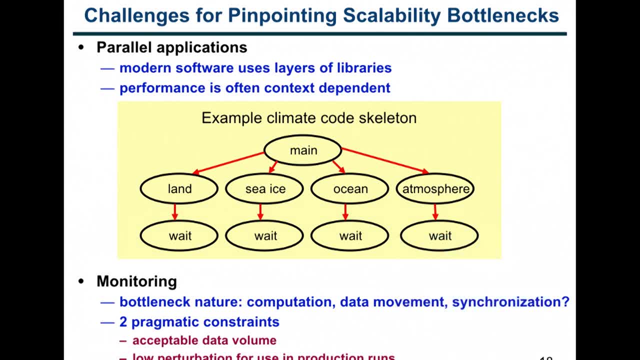 I'm spending a lot of time waiting in the ocean model, And so that may indicate that I've got some sort of problem with my load balance or whatnot inside the ocean phase. So when we're monitoring your application, the bottlenecks might be anything. 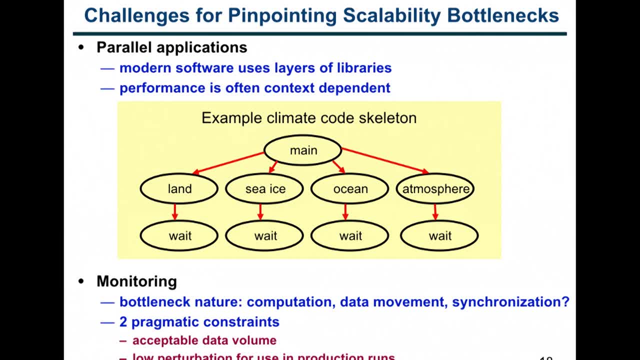 It could be computation, data movement synchronization, And so, for our measurement tool, we have two pragmatic constraints: One is that we can't record too much data, And the second is we don't want to spend too much time recording data. 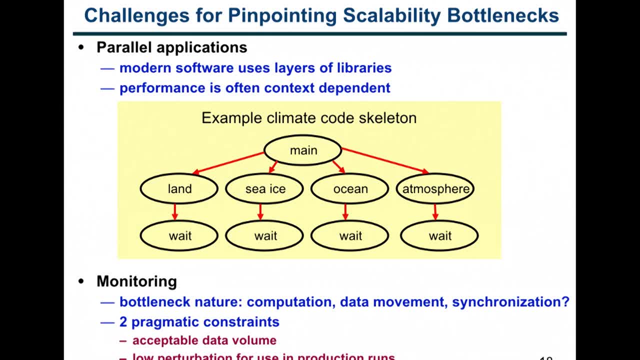 We want to perturb your execution as little as possible. Otherwise whatever we're measuring might not be sort of a faithful measurement of the performance of your application. So when you run your application, you have strong expectations for what it's going to do. 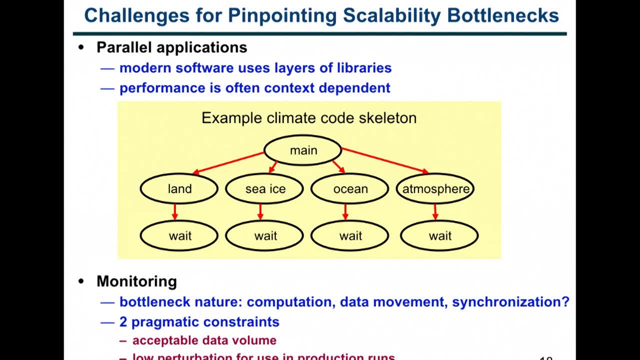 You might be performing a strong scaling experiment, where you take the same problem and you run it on twice as many processors and you expect it to be twice as fast. Or you might be doing weak scaling, where when you double the number of processors, you double the problem size to get higher resolution. 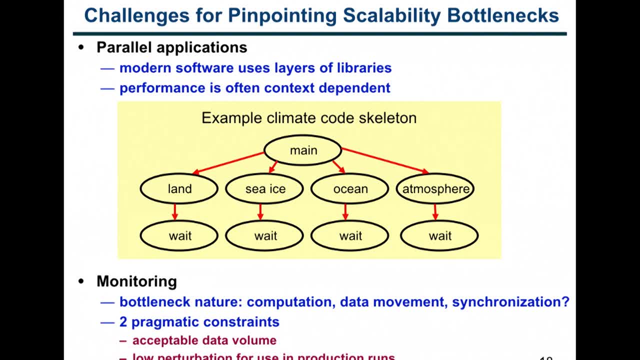 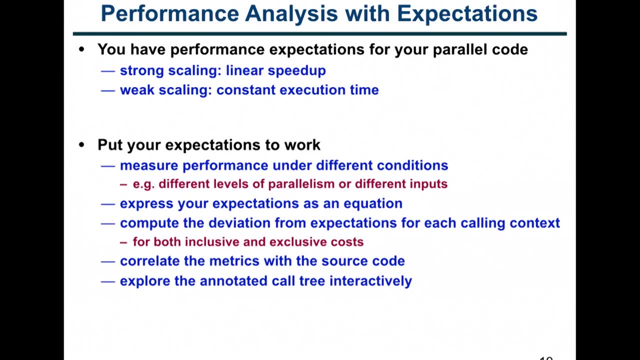 So the idea here is that you can put your expectations to work. You can measure the performance under different conditions, for example at different levels of parallelism or on the different input sizes, And then you can express your expectations as an equation and compute the deviation of your expectations. 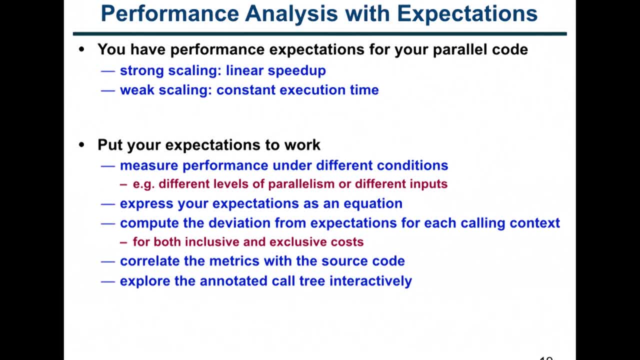 for every calling context. That's something that our tool will do: Correlate the metrics with the source code and then you can explore the whole thing interactively, So at a high level, when we're measuring your performance, let's say, on P processors. 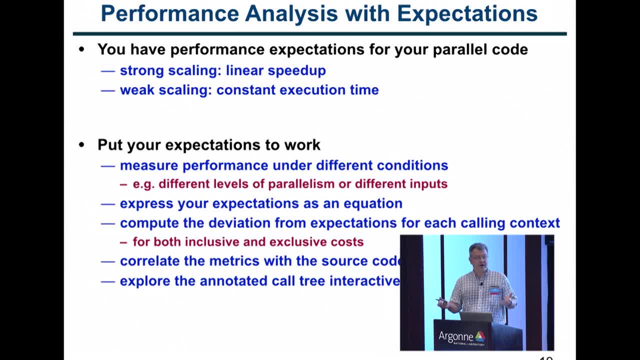 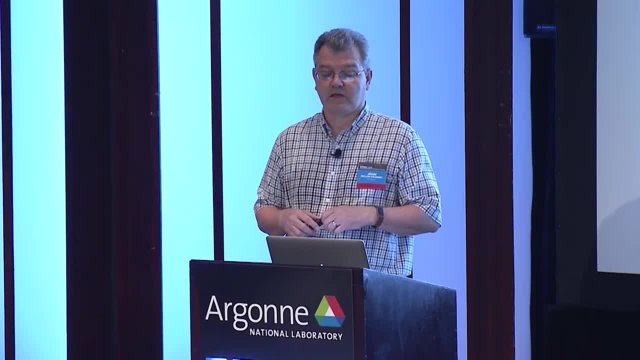 and so here's our calling context tree, and I've colored these at different levels of intensity to indicate sort of maybe how much metric accumulated it at any node in the tree. And so I measure it on, say, 256 cores and then I measure it on 8k cores. 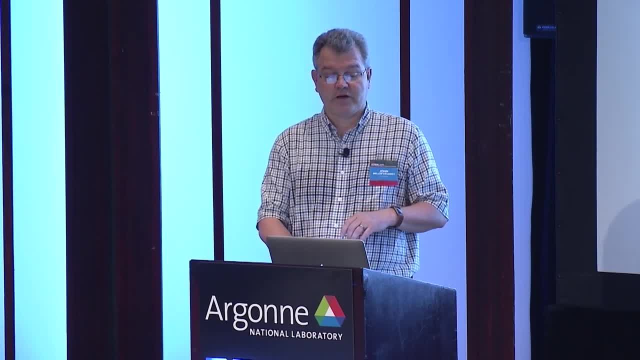 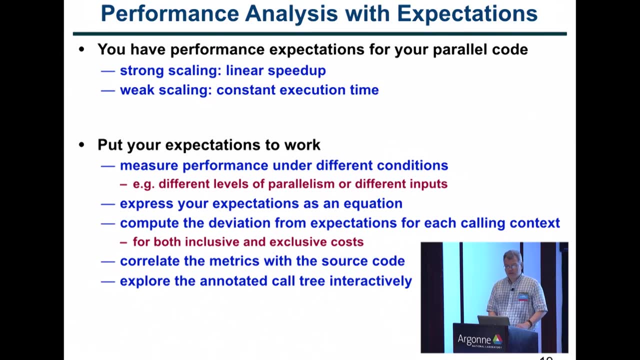 and I get a different distribution of where I spent my time. And so, for instance, if I spent 400k units of time in the solver, when I did this on 256 cores and then I took the same problem and I ran it on 8 cores, 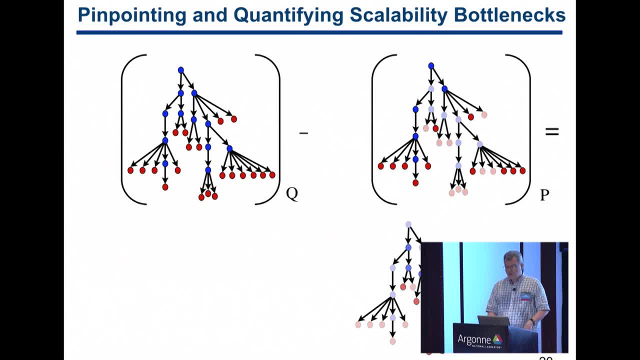 and then I spent 600k units of time in the solver, then what that would mean is that I have a wasted effort of 200k units of time. I've spent more time in the solver instead of when I took the problem and I split it up on a larger number of processors. 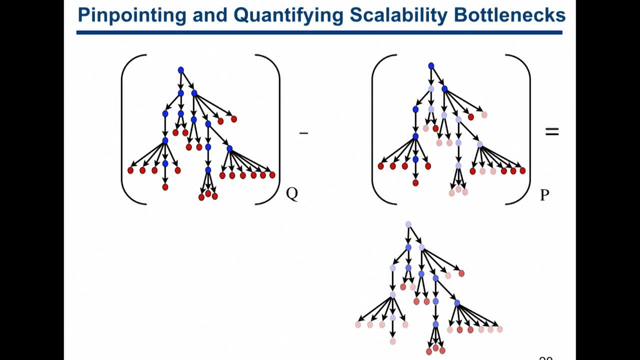 I invested more total effort in there, And so this represents wasted effort. and if I divide it through by the total time that I spent on Q processors, then I have the fraction of wasted effort. If I multiply by 100, that's percent wasted effort. 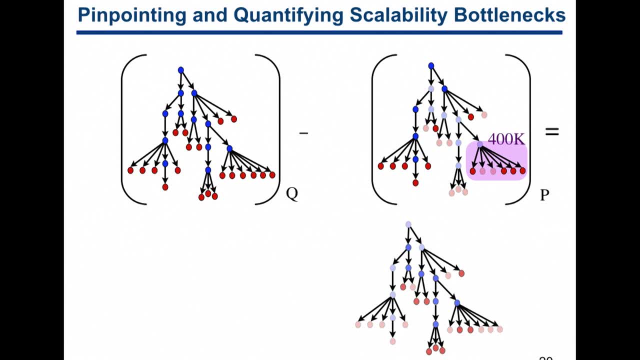 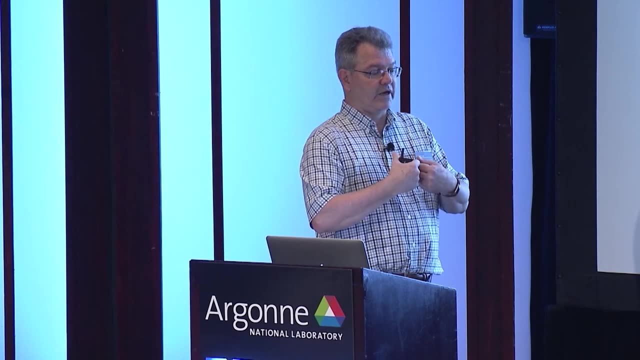 which is exactly the same as percent scalability loss. Okay, So let's. And then if you're doing weak scaling, then you can just multiply through some coefficients, because you're actually doing more work, All right. So let me demonstrate this with a canned example. 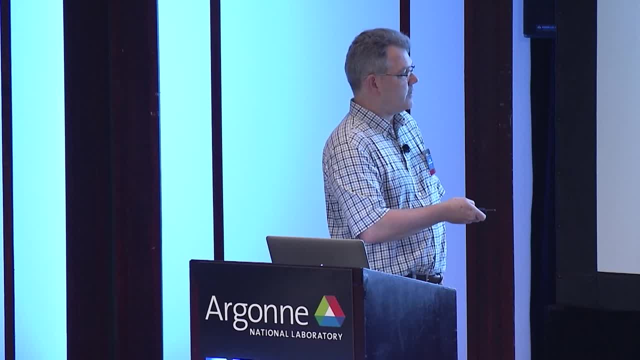 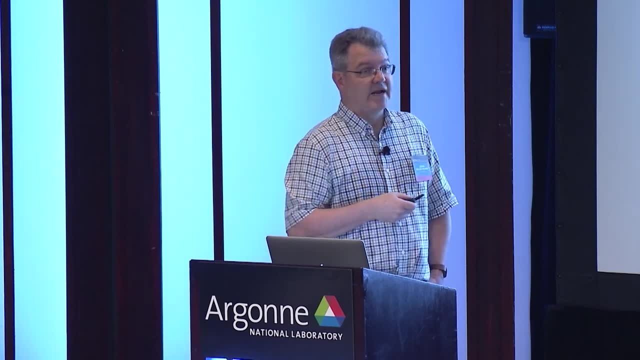 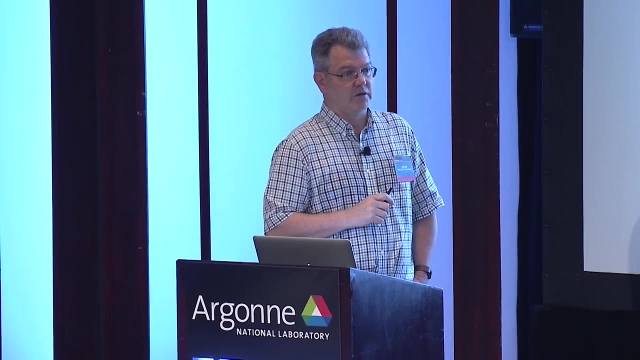 that I have on my laptop. So this is applying this scalability analysis idea to an adaptive mesh refinement code that does block-structured adaptive mesh refinement. It's designed for compressible reactive flows. It simulates things like helium burning on neutron stars, And here I'm going to use it to analyze. 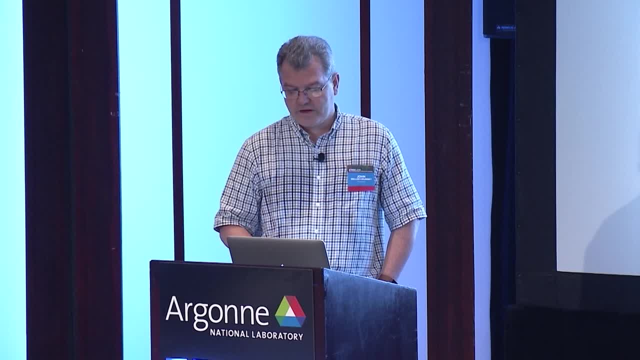 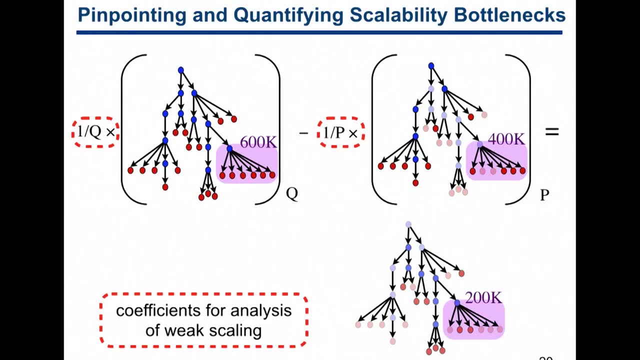 two executions of a white dwarf detonation, And so this is a classic piece of data that we measured on R2 from the Paragon's Blue Gene P system that was before the Blue Gene Q, And I use it because it's just such a nice example. 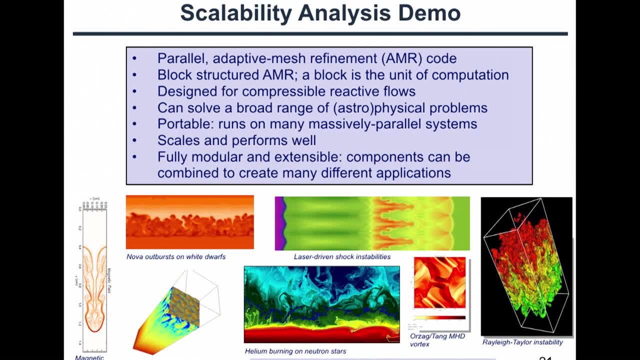 Okay. So what I'm going to do is I'm going to take the source code-oriented interface, So I'll open the tool and then I'll go look in my demos directory. So what this shows me is: I've got a couple of columns here. 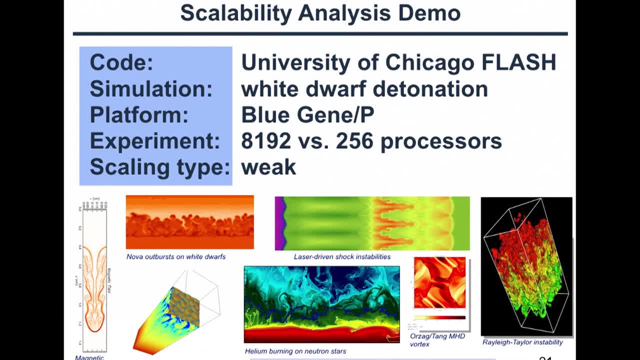 So there's one column that says 256 cores. wall clock time: inclusive and exclusive time with 256 cores and inclusive and exclusive time with 8K cores. Now, what I did here is I just took measurements from one core of each of these executions. 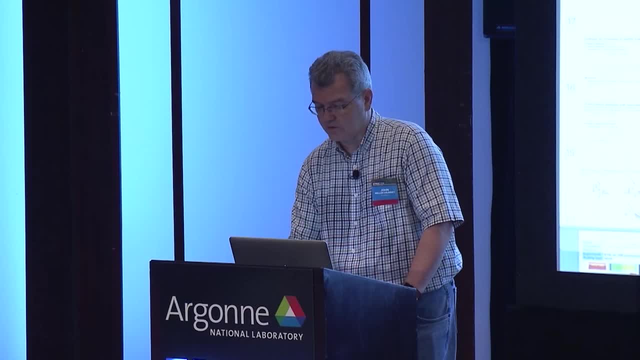 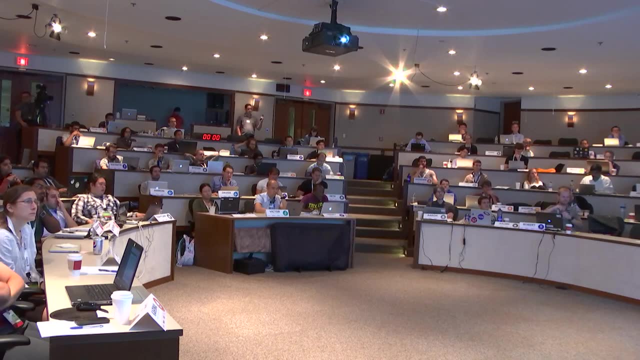 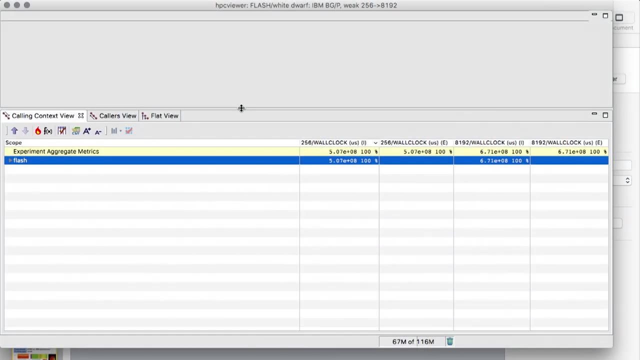 And so it was a weak-scaling experiment, And so what I would expect is that the time spent in each of these executions would be exactly the same. As I increased the number of processors, I increased the problem size, Now using this interface. 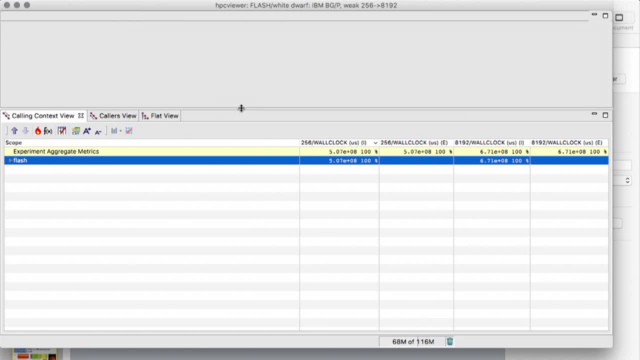 I can just go and sort of hunt around and say, okay, so 100% of the time was spent in this code, Flash or things that were called from Flash, which is the main program, So that's like a Fortran main. It says that 88% of the time was in Driver Evolved Flash. 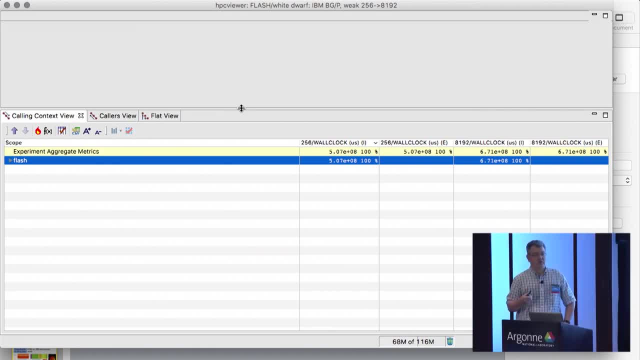 And so I can click on the function here and see the function, or I can click on the call site and it will show me where that function was called. This is all for highly optimized code. And then I can go in, click the flame button. 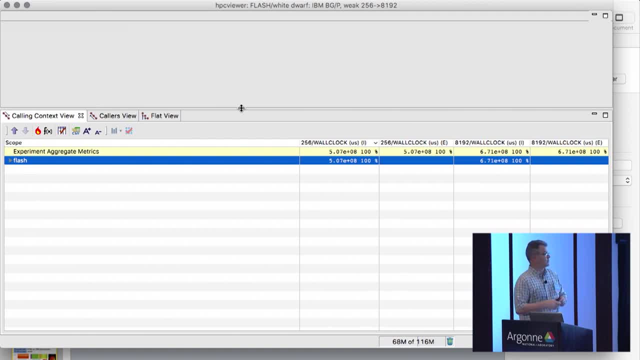 and it will show me, inside Driver, Evolved Flash, that time was spent inside a loop. Now, when I clicked on the loop, it didn't actually show me a loop header. In fact, the loop header is a couple of lines above and the reason is that we're mapping back to loops. 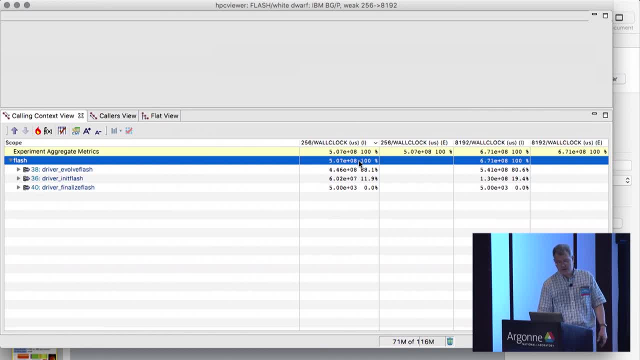 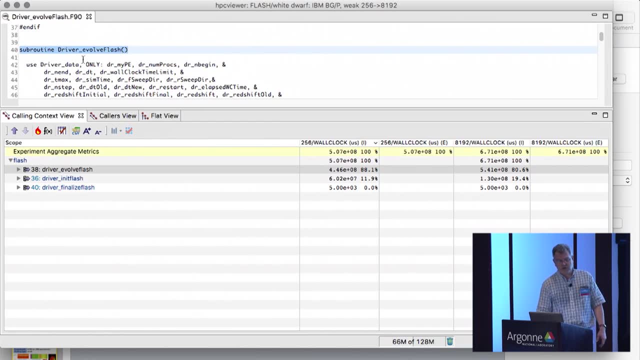 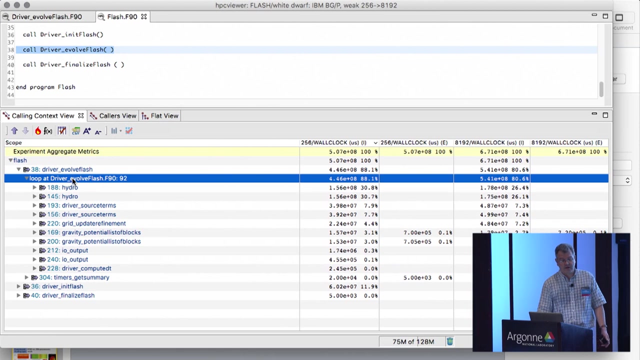 using source line mappings that we got out of the machine code, And sometimes the machine code only shows the first source line in the loop where executable code appeared from. Okay, So I can do this for both the columns for the 256 processor execution or the columns based on the 8K processor execution. 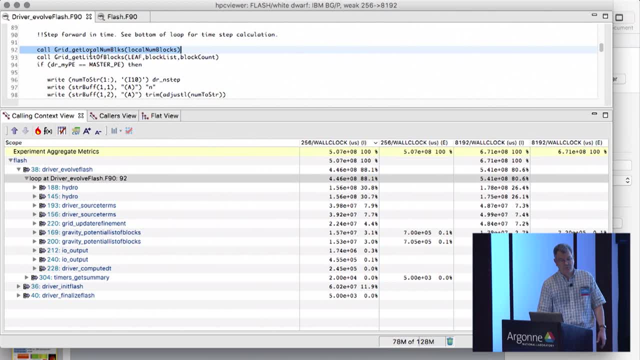 I can look at the bottom-up views. So, for instance, if I want to know where I spent the most of my time in my 8K execution, I can scroll up to the top and it says I spent 16% of my time. 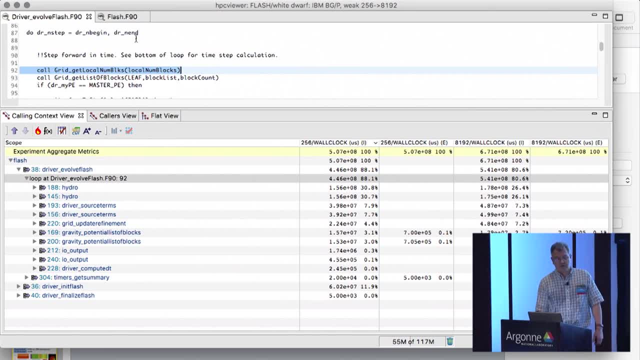 in DCMF protocol. multisend tree reduction. Multisend tree reduce. short post: receive message advance. That doesn't mean anything to you, Okay So, but the cool thing is I can just hit my little flame button and say: how did I get here? 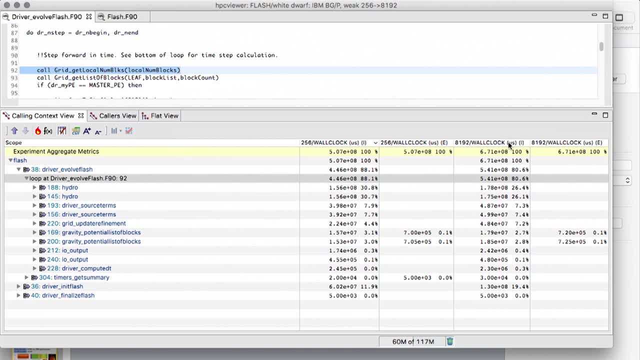 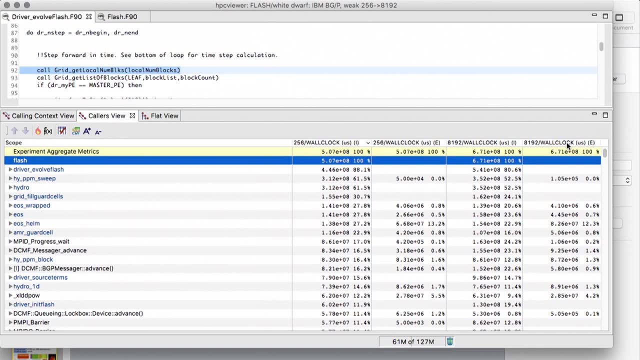 And then I start looking up the call chain and all of a sudden I see things I recognize like PMPI: all reduce. Okay, so this is an all reduce, and the all reduces in the program that are important are from the following locations: 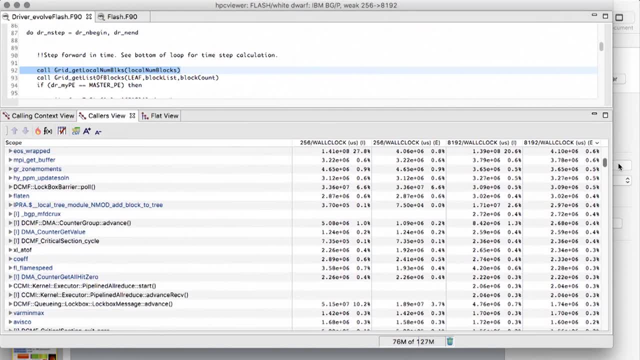 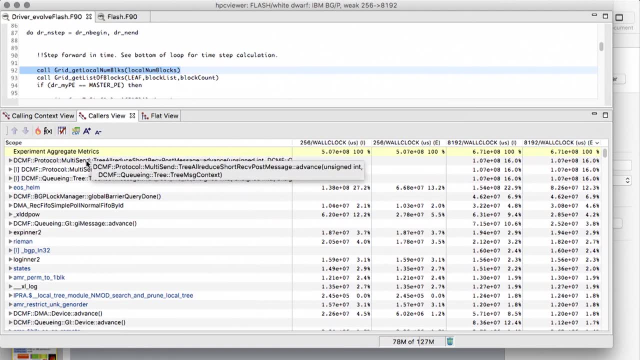 I can see different places in the program where all reduce is called the 16% of the time that was spent in all reduce, 14.2% of it was spent in MPI, AMR comp setup. Okay, So that's just sort of general using the bottom-up view. 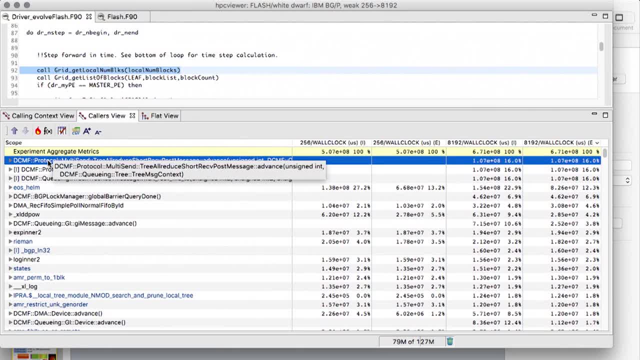 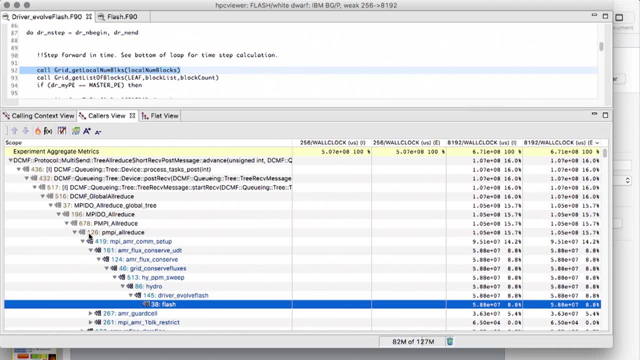 to find out where you incurred your costs. So now let's go back to the top-down view, and now we're going to compute the scalability loss. So I'm going to be doing exactly what I showed you here, where I'm differencing these trees. 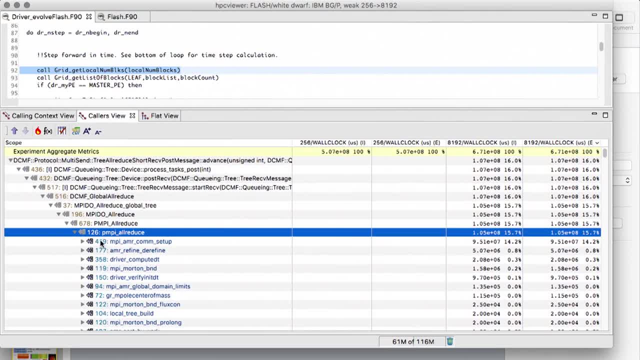 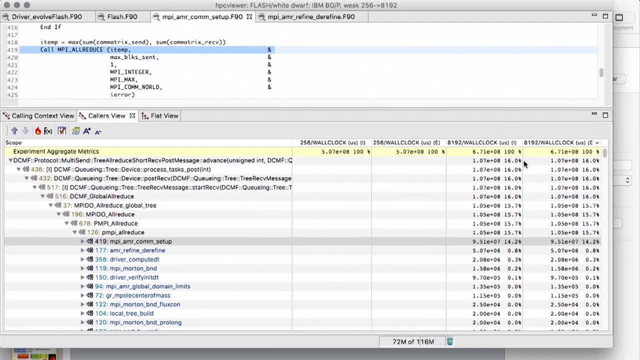 and finding my scalability losses. So I'll take the time on 8k cores, and then I'm going to subtract, and so what I'm doing is I'm just selecting a metric out of the menu, So each of these has a number that's associated with it. 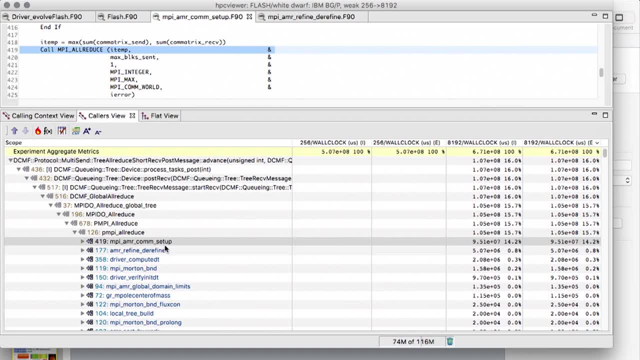 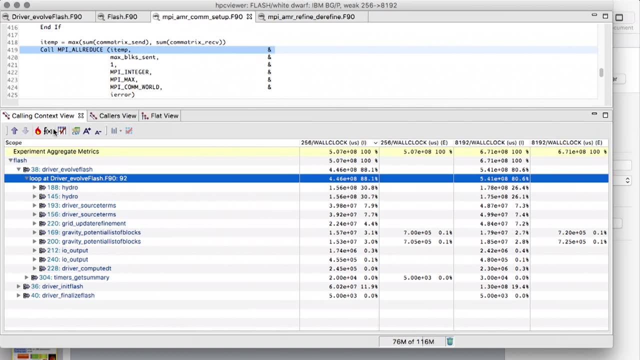 Think of it as like the column in a spreadsheet. okay, So then I'm subtracting off the time that was spent on 256k cores, and so the difference between the 8k cores and the 256 cores is wasted effort, and I divide through by the total time on 8k cores. 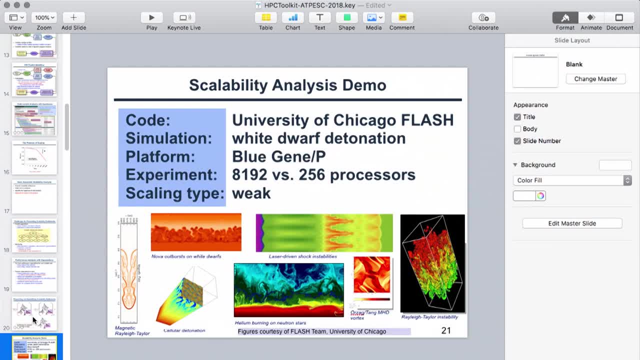 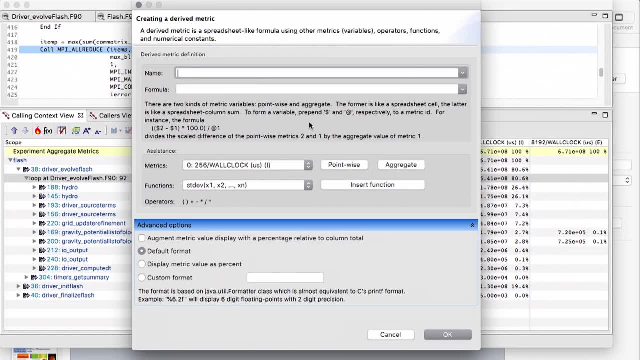 and that uses this at sign. So think of it as the dollar applies to every node in the tree and the at sign only applies to the root, And then I multiply by 100, so instead of having the fraction of wasted effort, 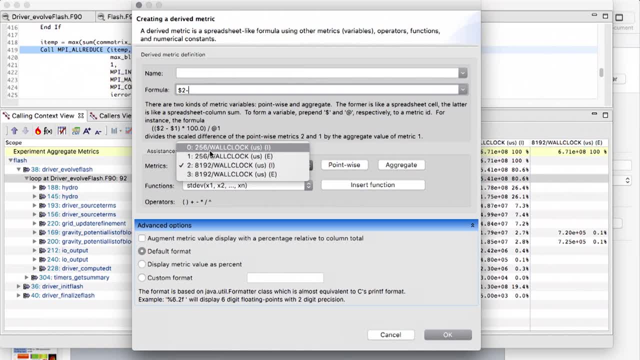 I have the percent wasted effort, which I said is the same as percent scalability loss, And I'll display this as a percent, and it says I have a 24% scalability loss. Now, if I were to look at this, it says that most of the scaling loss 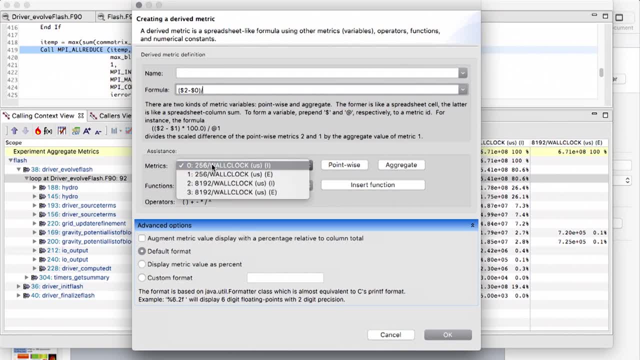 is in driver-evolved flash. There's 14% loss in driver-evolved flash, 10% in driver-init flash. So why don't we just take a look at the losses in driver-init flash first, since that's the first thing that the program does? 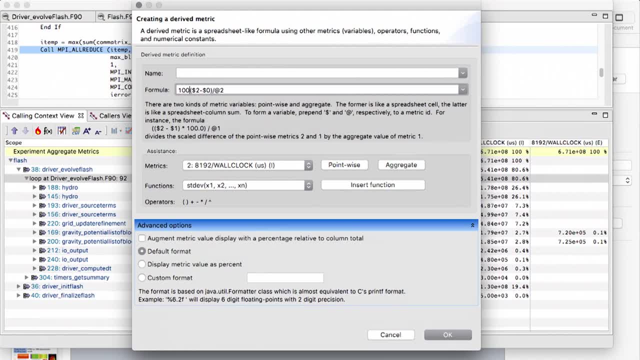 So if I click my flame button it drills me down into the code and brings me to a spot and I look at this and just a couple of lines above it says: do iproc equal 0 to nprox minus 1.. 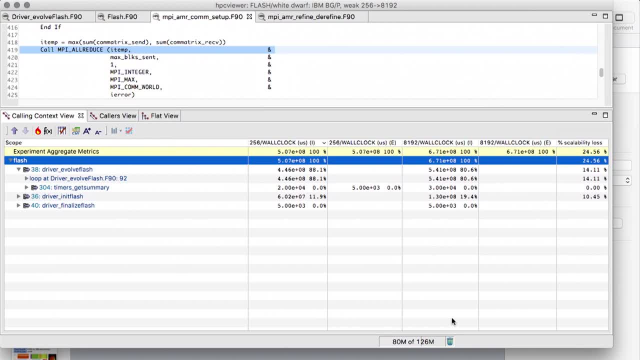 So what this is is it's a loop over the number of processors. As I increase the number of processors from 256 to 8K now, it's more trips around the loop. What's going on here? Well, inside this loop, 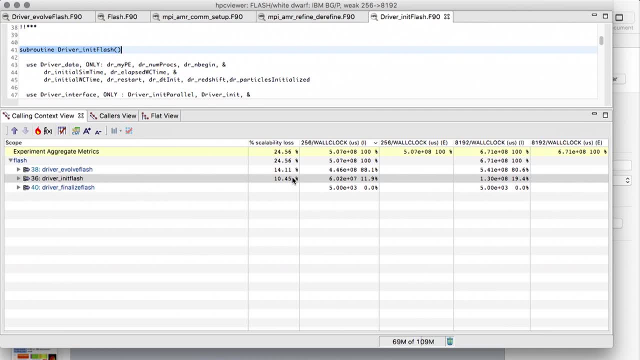 there's all of these calls to mpi send, receive, replace. So actually what's happening here is this is in the middle of adaptive mesh refinement: AMR refine, derefine Morton processes using space-filling curves to balance the load across the processors. 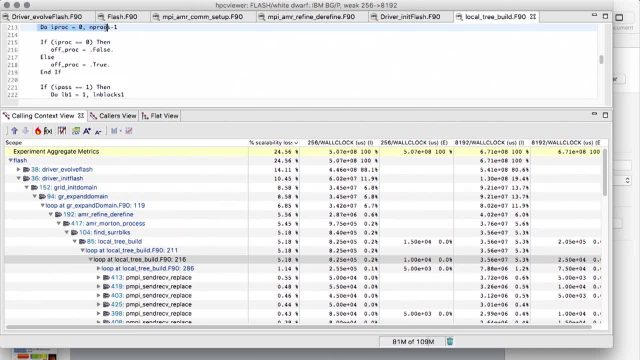 Find surrounding blocks. When I have a block of data that I'm supposed to be computing on, I need to know who my neighbors are, And so what it does is it says these are the blocks that I have, and it passes it to the right. 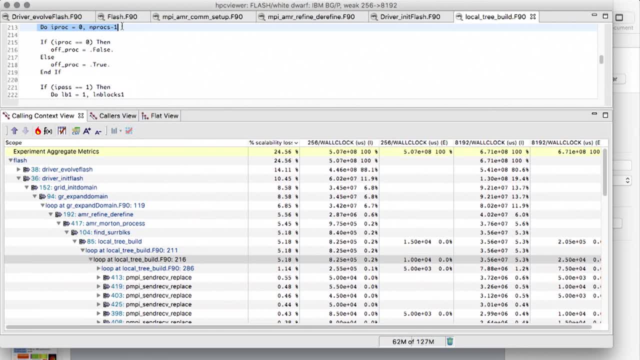 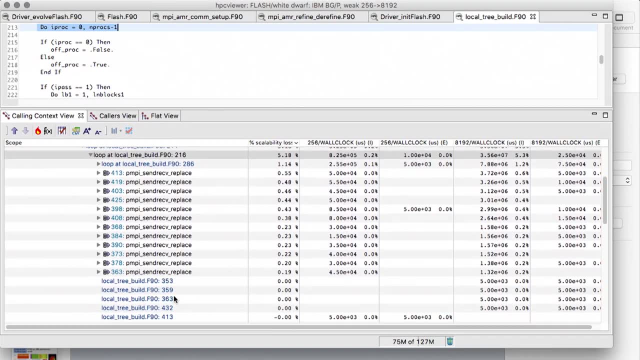 This passes all the way around a ring. I get to see what everybody has, and by the time it's cycled all the way around, I find out who has the things that I need, And so as I add more processors, the ring gets bigger. 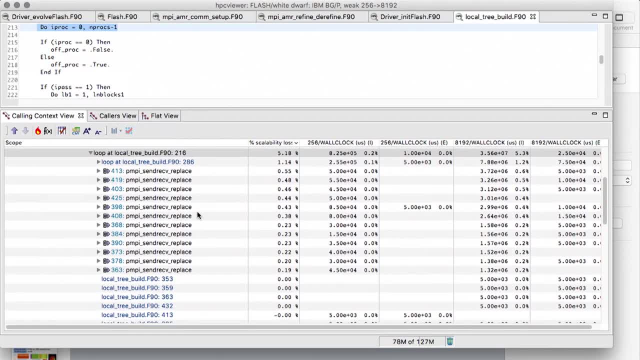 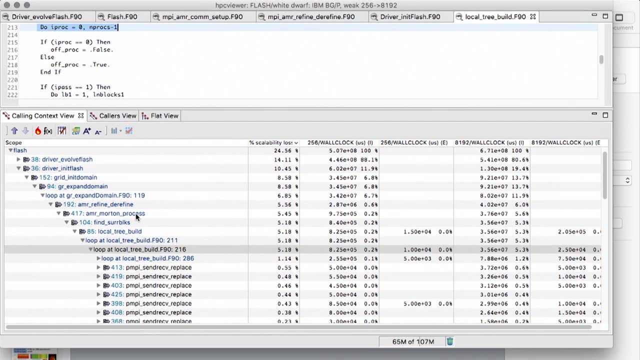 So what this is doing is it's doing an all-to-all, really, but it's doing it in a way where you don't end up with all of the data at once, Okay. So that's one example here That was in grid init domain. 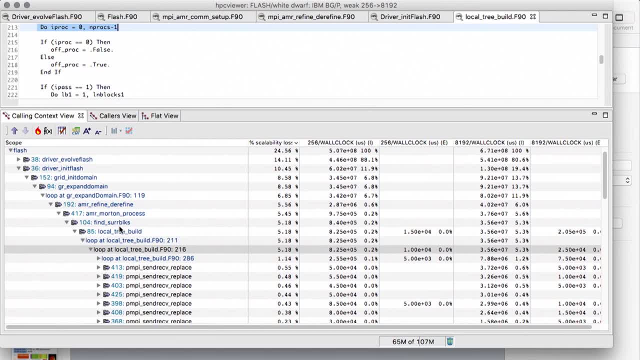 Now if I look at grid init and say let's look at where this 1.97% came from, Well, that takes me down into some other place where there's a call to MPI barrier. I see something that looks like: do IPROC equals? 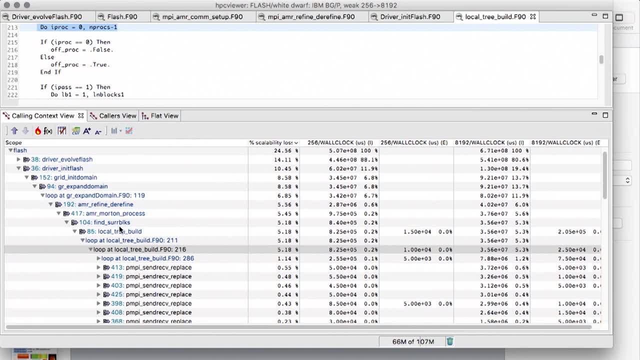 There's reads looking up for the top of the loop, And now we find another loop: IPROC equals one to NPEs minus one. If it's my turn, then I open the input file. Another scaling bottleneck. Okay, Somebody ran it on something like 20,000 cores. 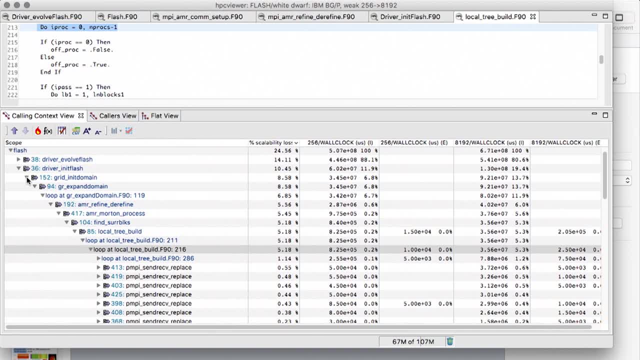 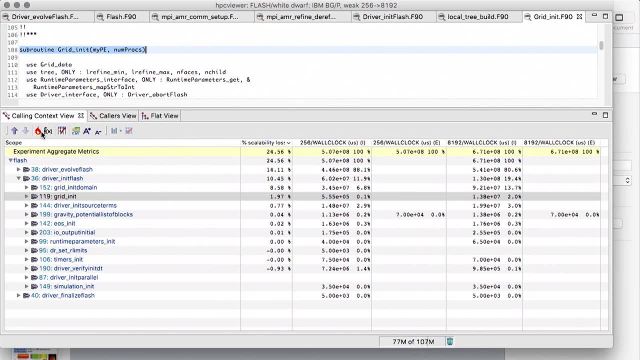 Everybody tried to open the same input file crashed the system. They said let's not do that again. So they said let's take turns, and then forgot about it, Left it there in their application. Okay, Well, that was in the init flash. 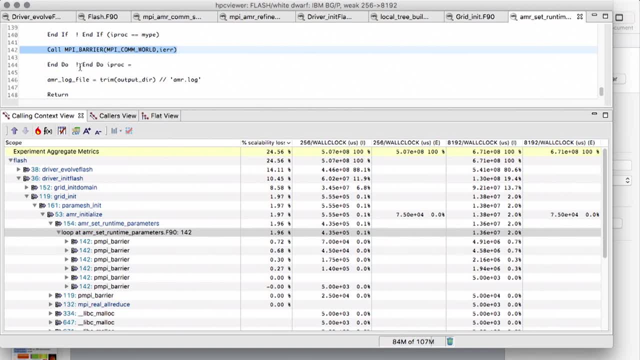 One more time in the evolve flash. I opened it up and then there wasn't anything that was dominant. It came down to the loop. So then I picked the top thing that's in here and used the flame button again, And it takes me back to exactly the same place. 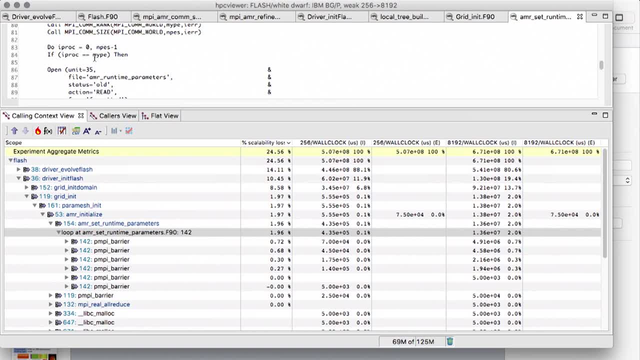 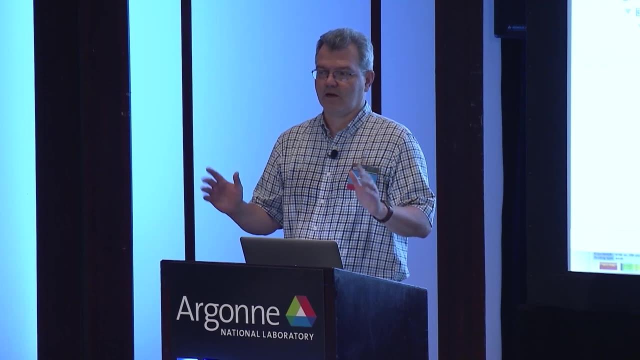 So the same oops, the same: refine, derefine, morton process, find surrounding blocks. I'm back in the same place. Okay, So that's our. that's the way you use this top-down interface. And so when Anshul Dube from University of Chicago. 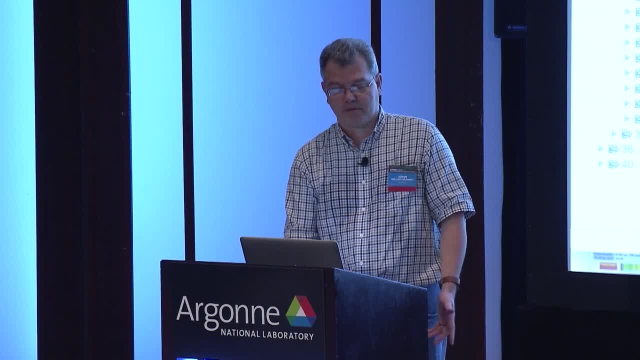 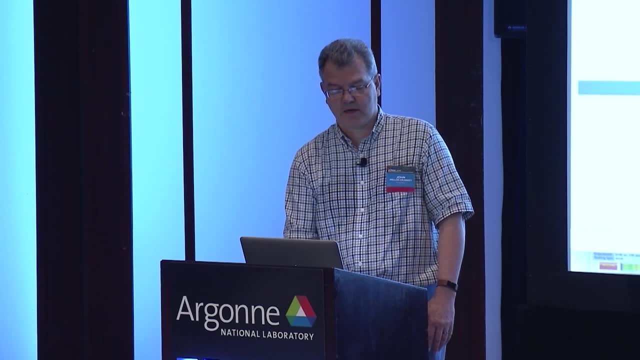 was informed about this, they said: well, first thing they said is: that's not my code, We got that piece of code from NASA. And then they said, well, actually we could do a little bit better. So instead of like circulating it all the way around a ring. 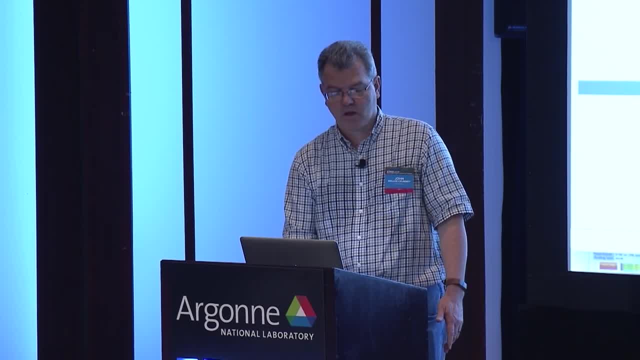 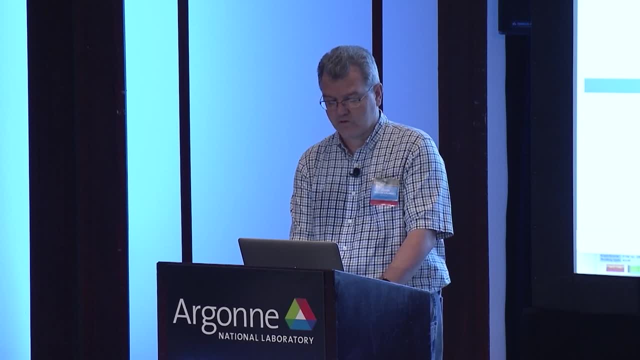 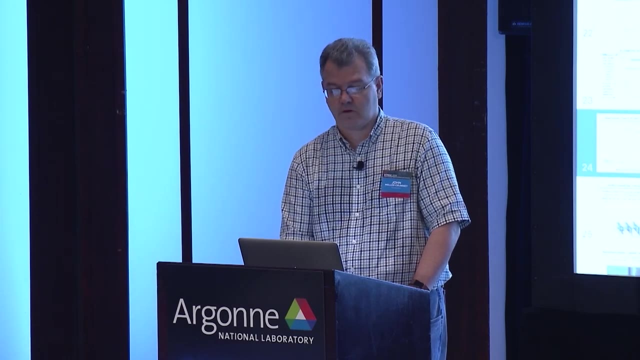 we can actually just query our neighbors, And so, instead of having the time grow as we increase the number of processors, it stayed flat and was scalable. Okay. So sometimes, though, knowing the profile isn't enough. You actually, you want to see the 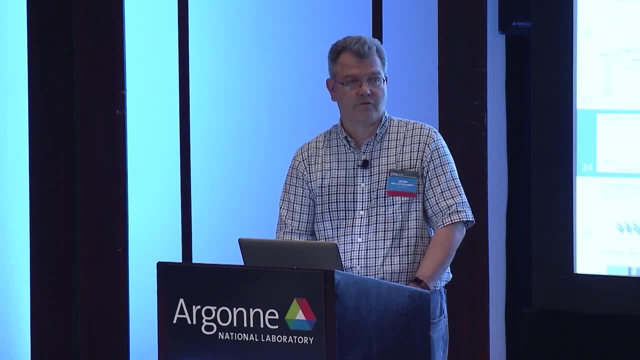 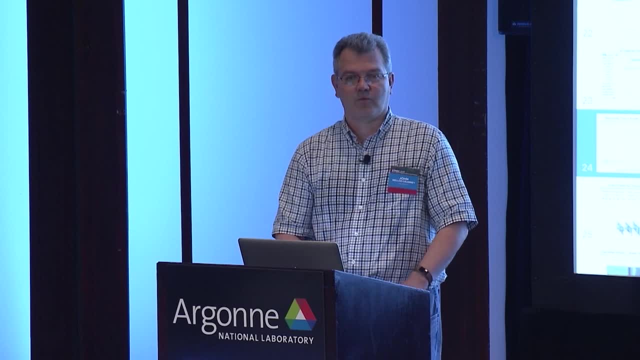 the temporal dimension. And so what can we do? We can trace call path samples. So at any point in time we unwind the call stack and we get some call stack And then. so at time t we unwind the call stack on thread one. 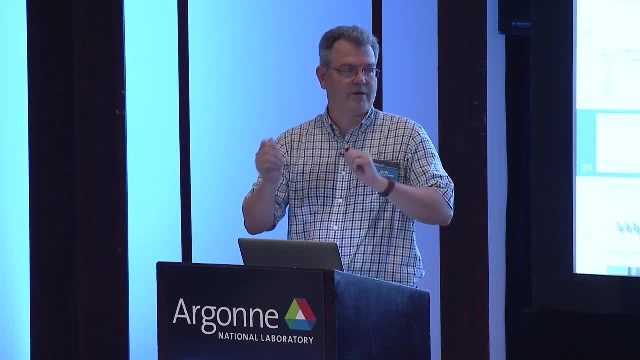 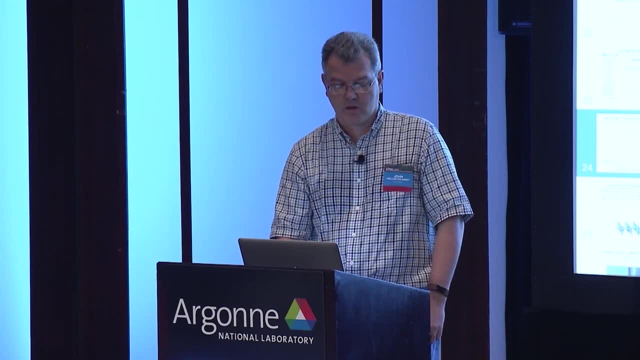 And then, at time t plus delta, we unwind the call stack on thread one And two delta and so on, And so we get a series of call stacks for thread one and for every other thread and every other MPI rank in the application. The idea here is that you have a visibility plane. 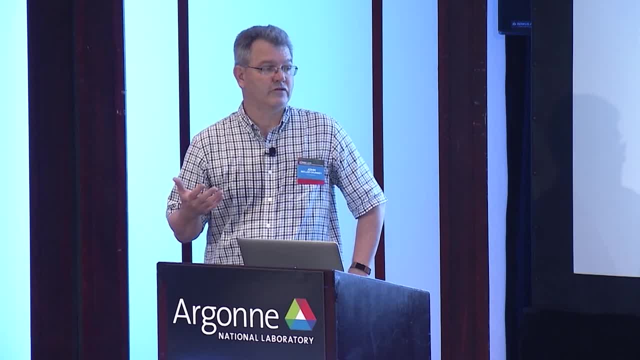 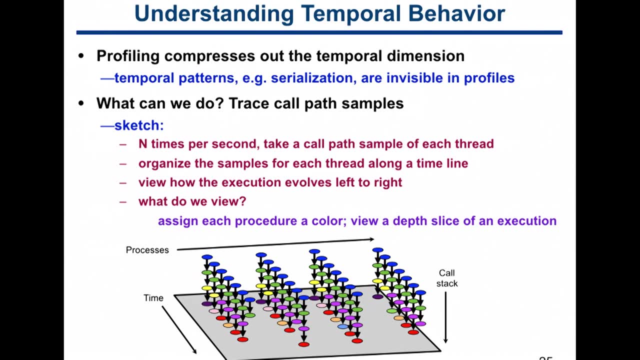 If you lift it all the way up to the top, you would see that everybody is in main or things. main calls for the entire execution, And as we move down a little bit we'll start to see differences between them. So let me just pull up an example here. 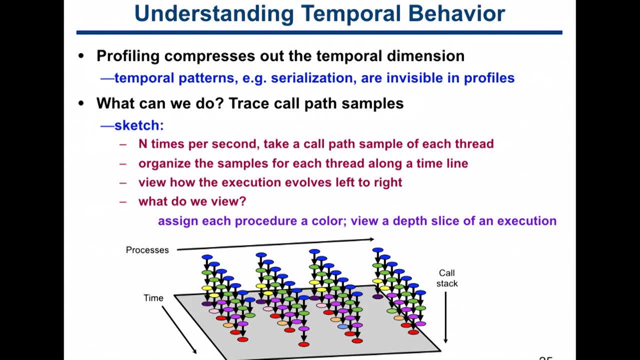 So this is a code called QMC pack, which is a materials code, And we were working on this with Nick Romero at Argon. So they had one implementation of QMC pack and then they were changing it to to add open MP to it. 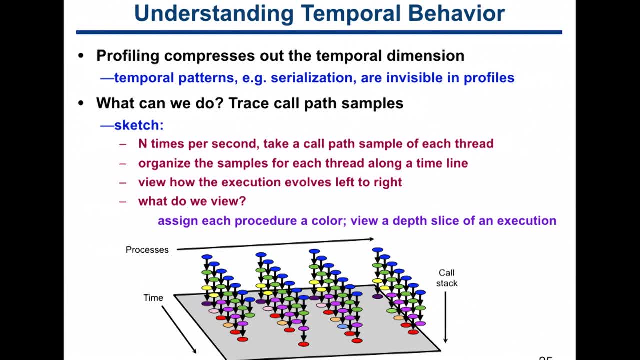 So at the top level it shows you mostly uniform color Over here. so this is like this represents program root, or moving down one level, it says main And you find that there's a different color over here and that's because we have this tools interface for open MP. 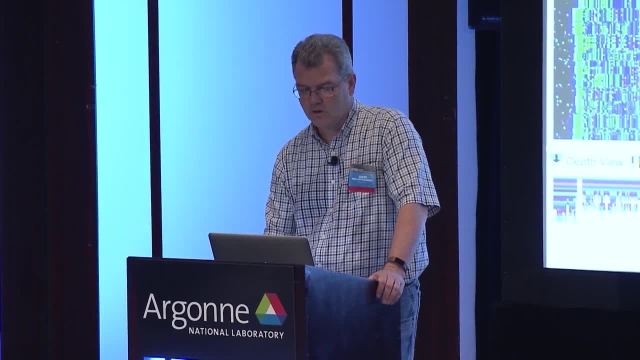 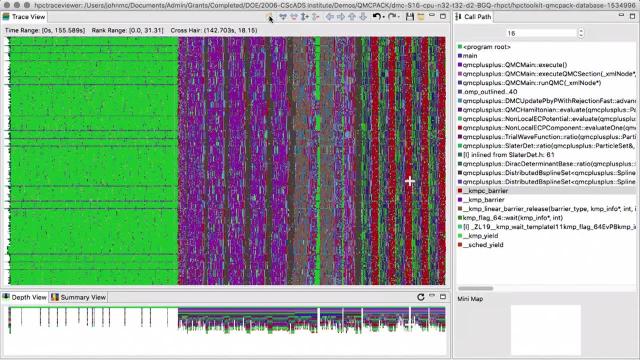 And so this just says indicates that open MP threads are idle. So you can't relate idle threads back to a call path, So the color is a little bit different. So then what we have is on the vertical axis, it's ranks and threads. 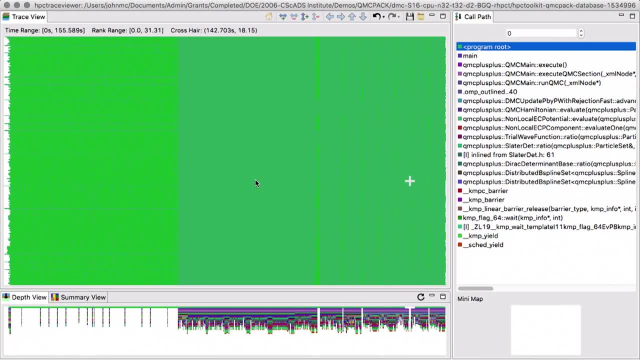 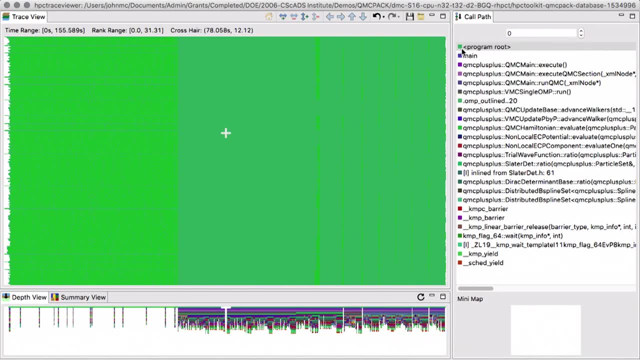 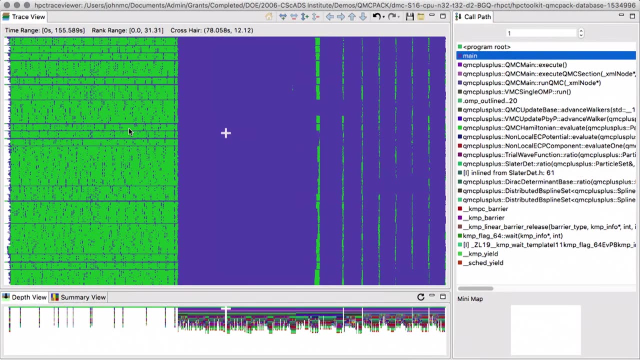 And then the horizontal axis represents time, The bottom window represents the call stack over time, And so this is showing 43 seconds into an execution that's 155 seconds long. There's 31 processes with 31 MPI ranks, with 31 threads inside each. 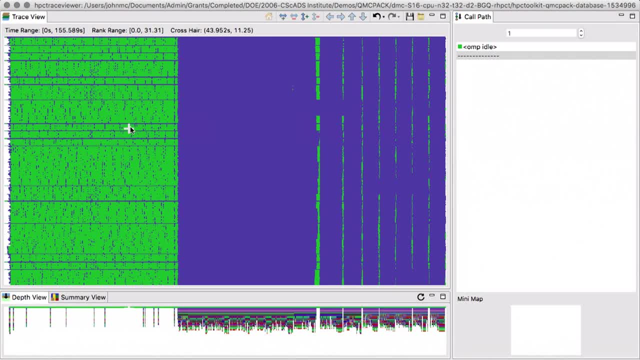 And so then I can just point it at a place in the execution And this will tell me the complete call stack at that point in time, And then, by moving down at different levels of the call stack, I'm getting to see my execution at different levels of abstraction. 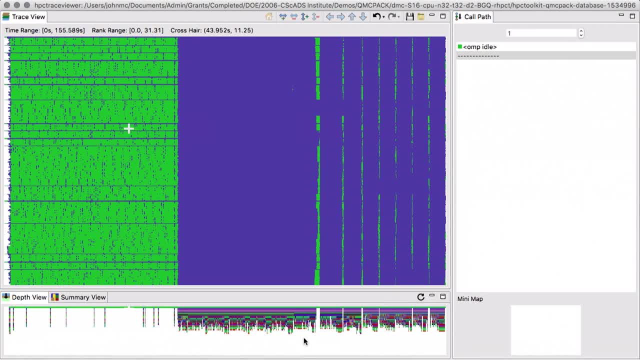 And so once I reach an interesting level of abstraction, then I can see that there are differences Here. this is doing something like QMC update base, advanced walker. So this is doing a quantum Monte Carlo code. And then in this second phase, 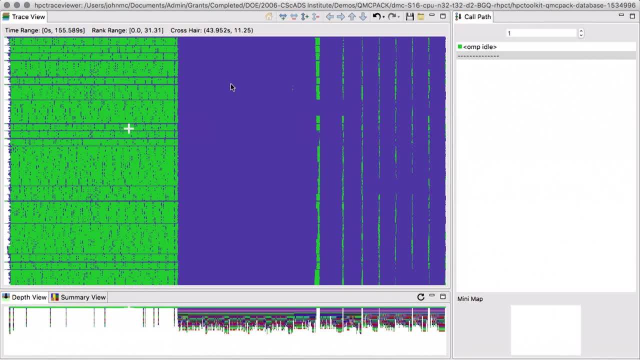 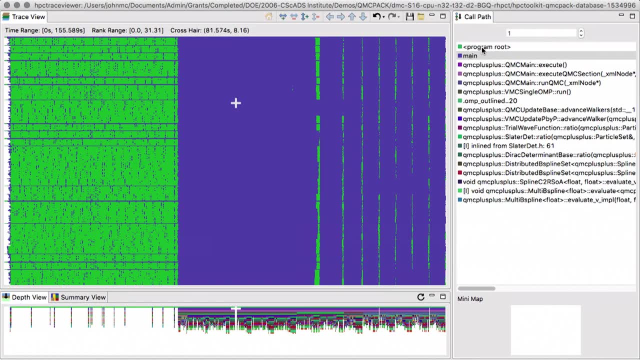 this is evaluating Hamiltonians, And so I don't have much time to go through this interface, but it turns out that by looking at this and looking all the way down at the bottom and finding out what you're spending your time doing, it turns out that red down here, 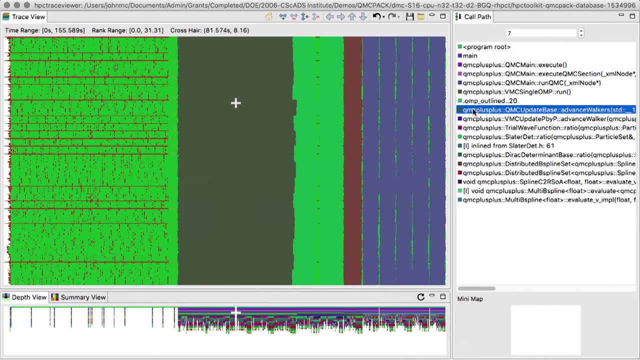 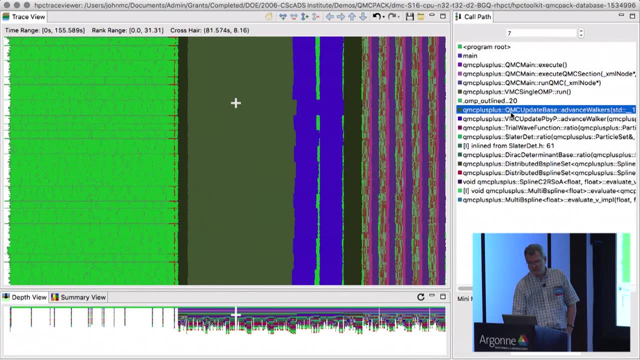 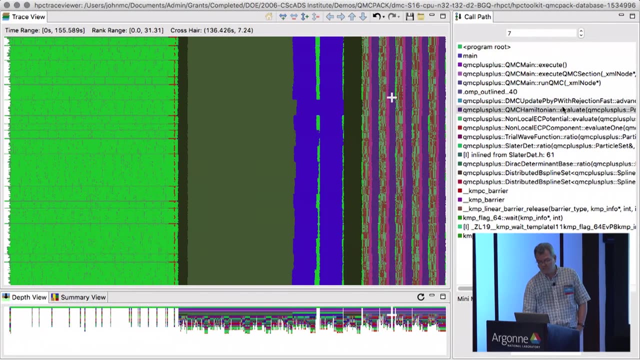 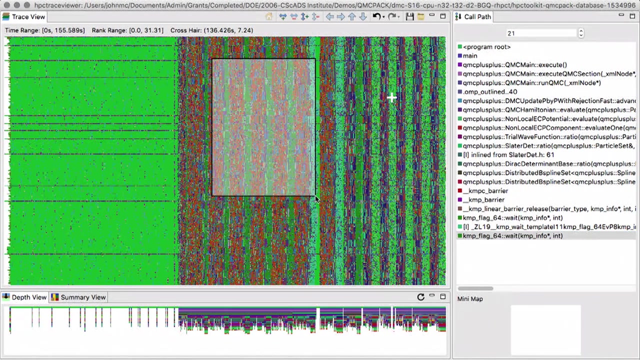 represents time spent in. If I add something here, it will So say: look for time that's spent inside the Intel runtime system and let's color it bright red. And, And as we look, we find that some fraction of our 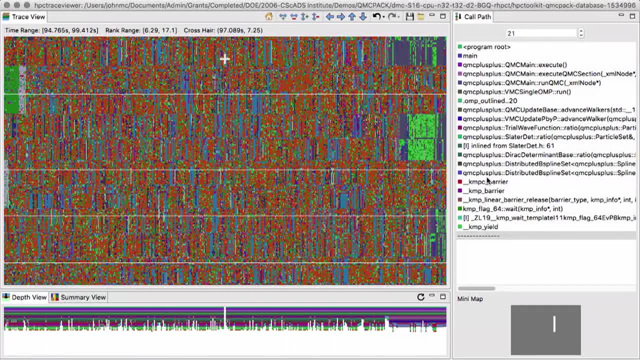 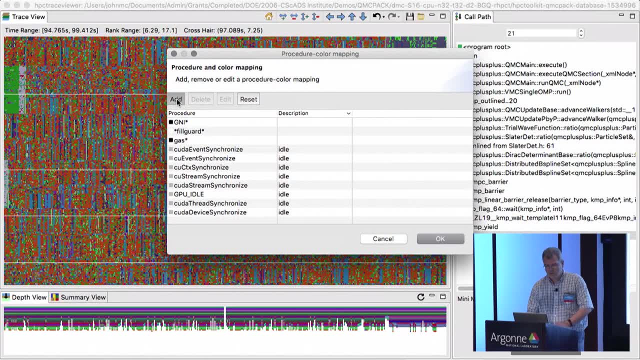 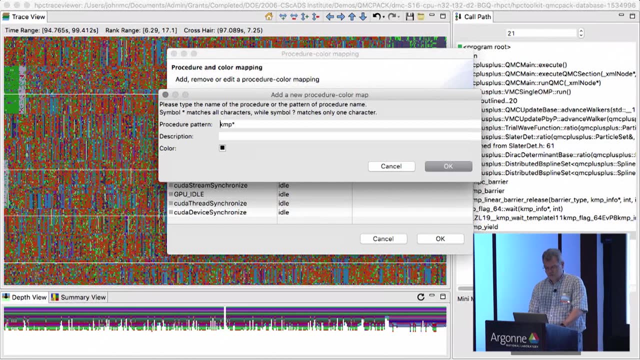 Oh, and then this green is schedule yield, so I should color that red as well. So that's saying that I'm giving up the processor, I'm just coloring it sort of red for convenience. And so what this is showing me here. 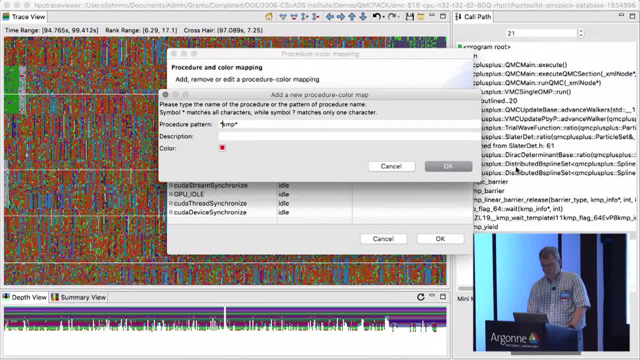 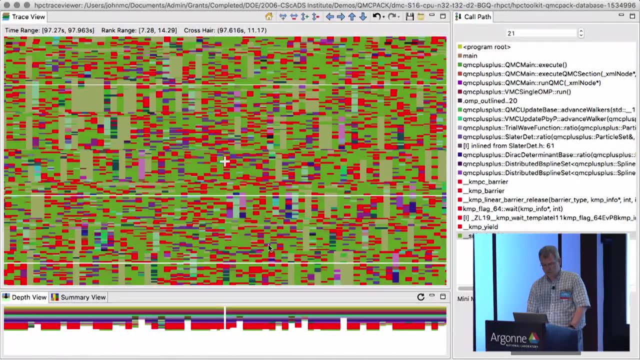 is everything that is now colored red represents bad stuff. This represents basically wasting my time, And now what we find is that we're wasting 50% of the time. okay, This is what you can find out from this interface, And that is we look at the execution over time. 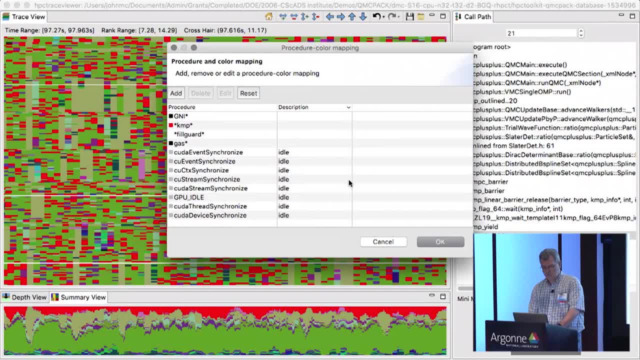 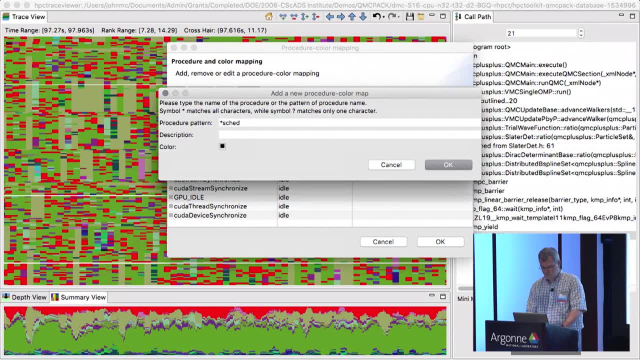 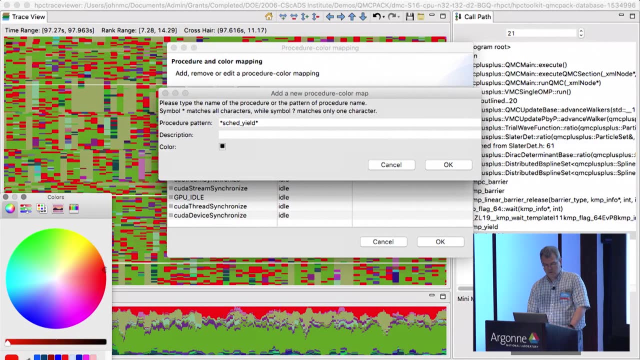 In fact, we see, well, there's this setup phase and then for the rest of the execution, we just waste our time. You can find this out by your code too. You'll be surprised. So one of the things that we've spent a lot of time doing. 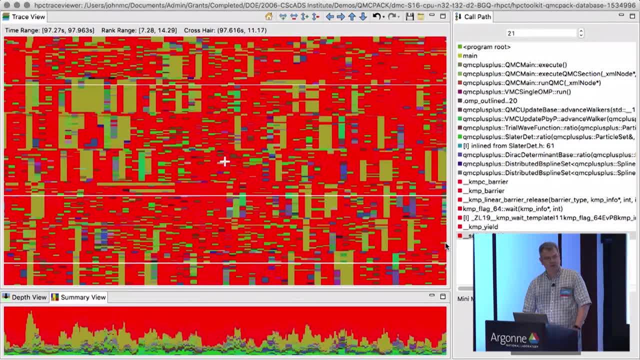 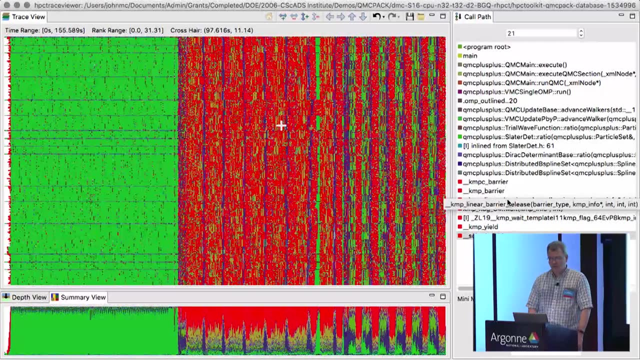 over the last couple of years is that for OpenMP, if you don't use a special interface inside the OpenMP runtime you'll see a view that represents an implementation-level view. So the OpenMP compiler will tear loop nests out of your program and put them in separate functions. 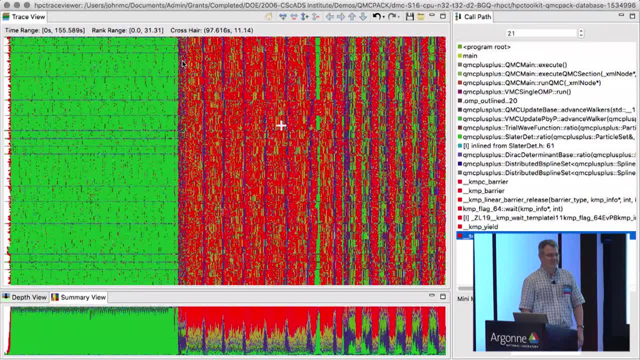 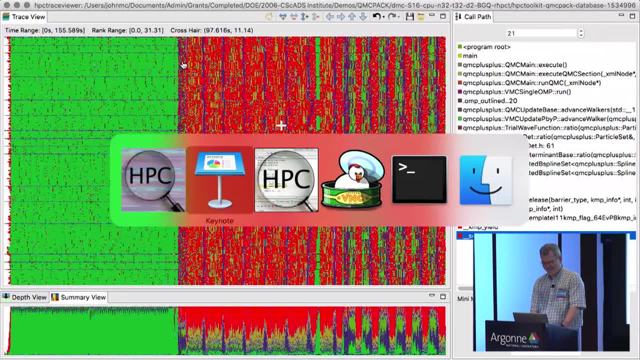 and you'll see something here where this looks like: KMP launch worker is calling launch thread is calling invoke task and then these are some things that you never wrote in your program. They've been like they're machine-generated, They're compiler-generated routines. 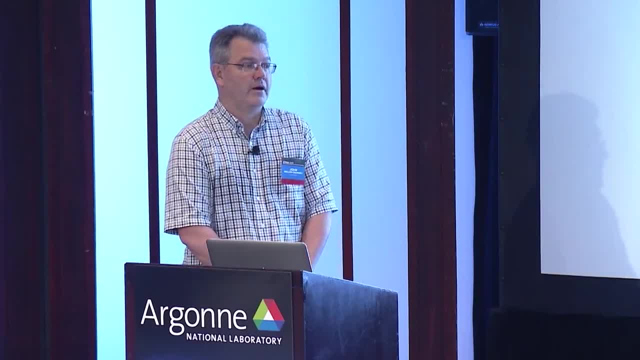 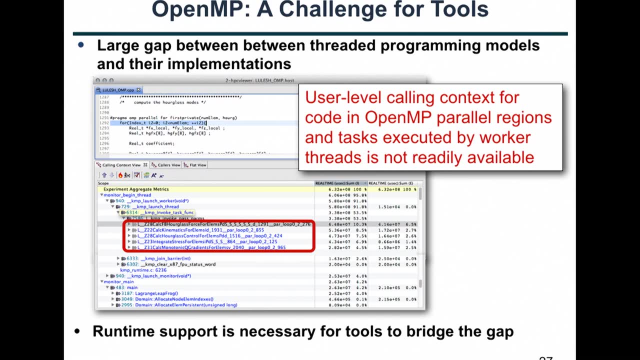 And so what you really want to know is like: how did I get here And how did I? And I want to understand these routines in context, And so we built this OpenMP tools interface. We started on this process in a collaboration with IBM. 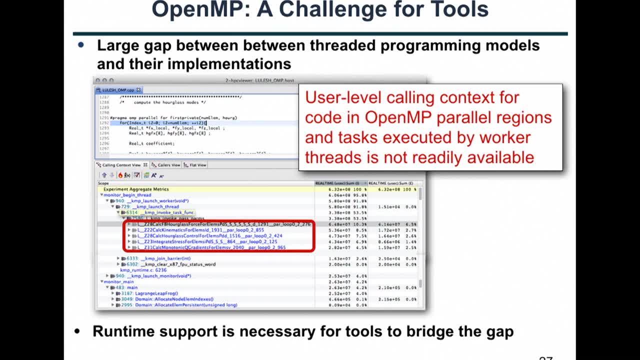 when Mirror was originally purchased, and we've been working on this since 2012 and making it part of the OpenMP standard And so, as part of OpenMP 5, when it's released in November, it will have a tools interface. 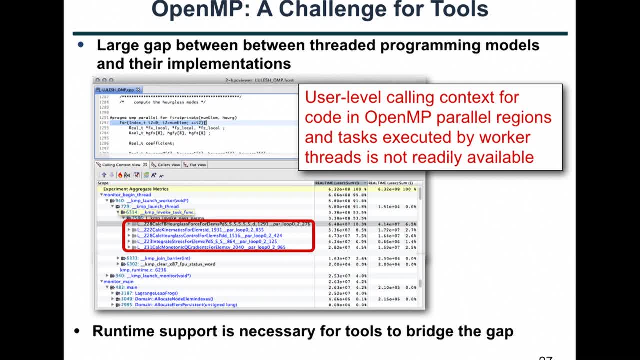 And what the tools interface will enable us to do is to paper over the differences between the master threads and the worker threads and show you a source code-oriented view of your application. So we've designed this standardized tools interface and some of the tools around the room. 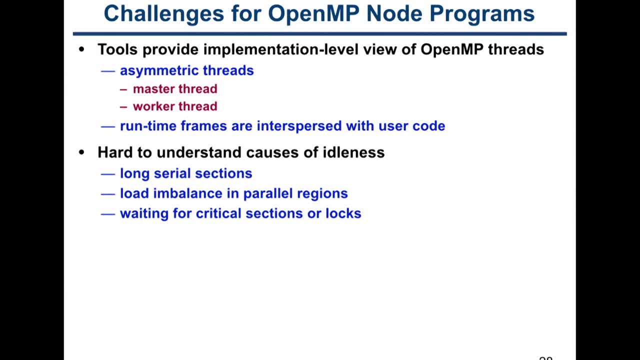 that you'll hear about today are starting to use this, And so in our HPC toolkit, this is the source code-oriented view, and now what we're seeing is that the OpenMP routines that were torn out of the application are shown sort of in the full calling context. 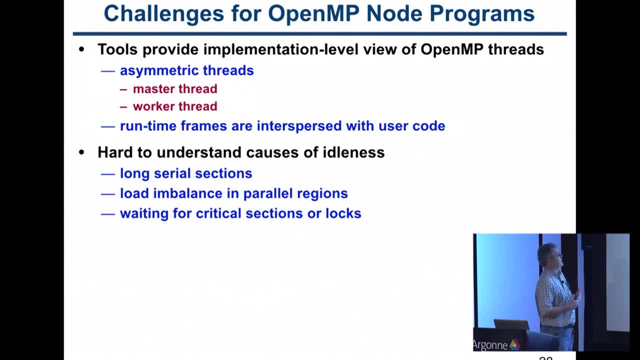 that we see that the time is incurred in this OpenMP routine And then we're also able to graph, like thread and process views to see this: the variability of the amounts of time that are spent in. Some of the threads are spending a lot of time. 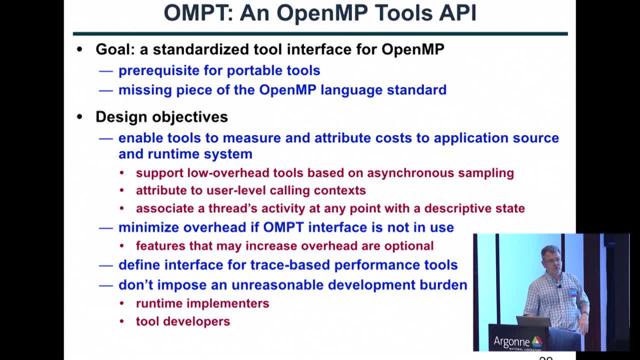 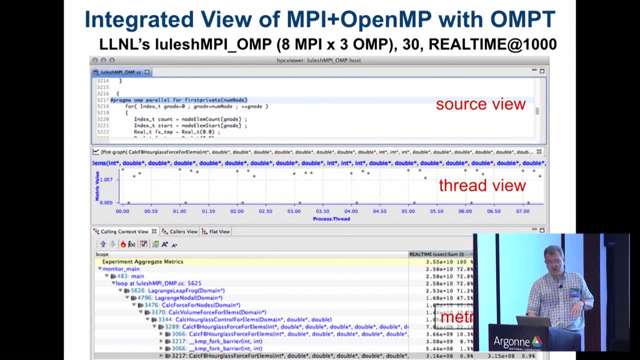 and other threads are doing nothing. Okay, And so there's a knob for this thread-level view as well, and so it's not shown in this version of the interface, but there's a knob there in the version that you could use, And so then this is showing. 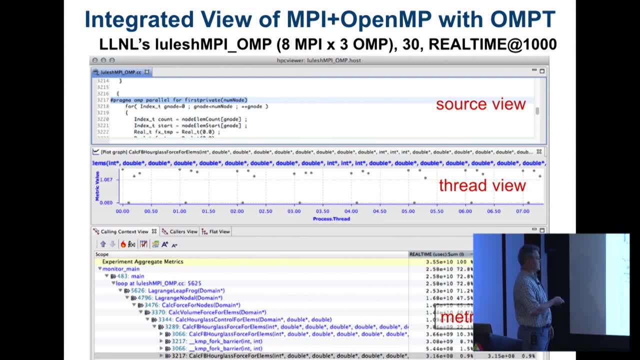 a trace-level view for an OpenMP code. This is an algebraic multigrid code, And so, things of note, here we're inside some phase in, So these are like MPI ranks, and then there's a set of OpenMP threads. 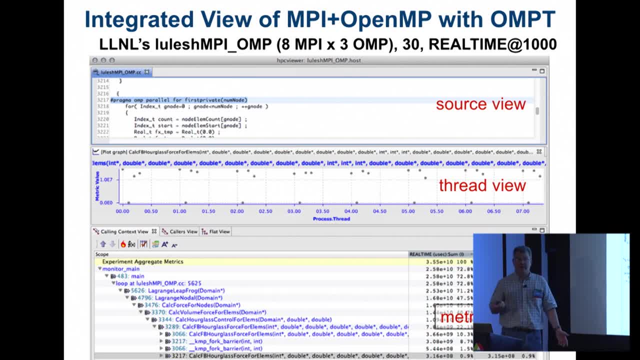 So there's four MPI ranks and eight OpenMP threads, And so for these regions where all of the threads are colored the same, then that means that everybody's working together, executing OpenMP Where it's gray. here, that means the OpenMP threads are idle. 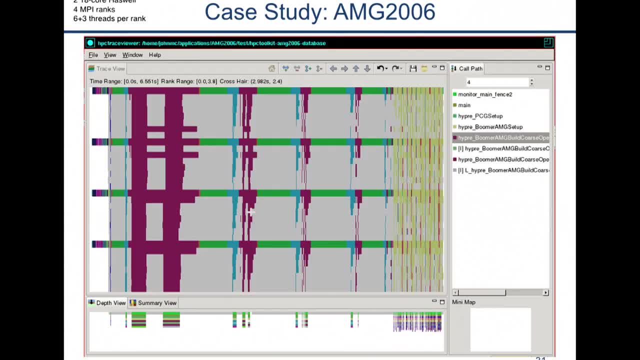 So that means this is a piece of serial code. Okay, So from this level, From this view, you can find out that you've got serial code. but also we have something that we call blame shifting. that's integrated into our tool where, when a thread is waiting for work, 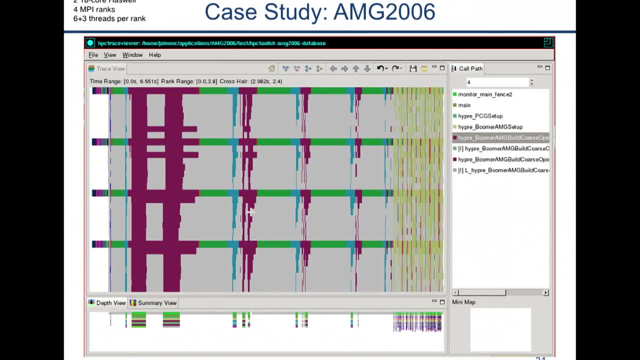 we blame the thread, that's, We blame the code that's executing in serial for not shedding enough parallelism to keep us busy. And so you can. You can measure OpenMP idleness and say: I want to measure in cycles and I also want to measure OpenMP idleness. 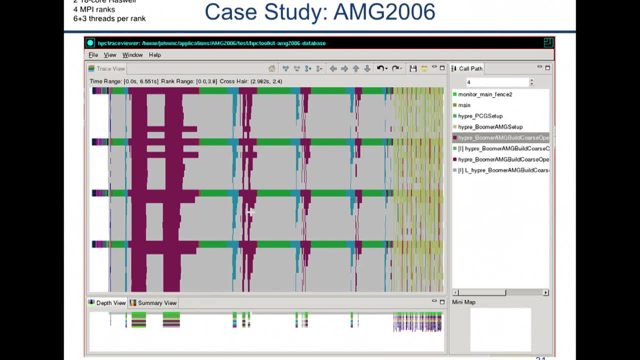 And then if we measure OpenMP idleness, then we can find that routine. where it was green. It says that 50% of the idleness in the program is attributed to this function. What that means is that threads were idle when I was spending my time here. 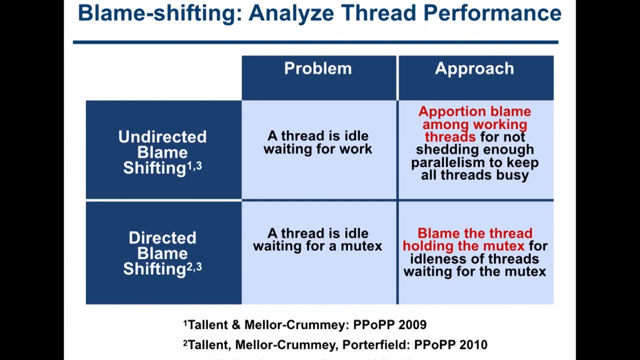 Okay, I'm pretty much out of time, So we're working on integrating this with the OpenMP tools interface, which is going to be released in in the upcoming version of OpenMP in November. Right now, we have a prototype of the interface. 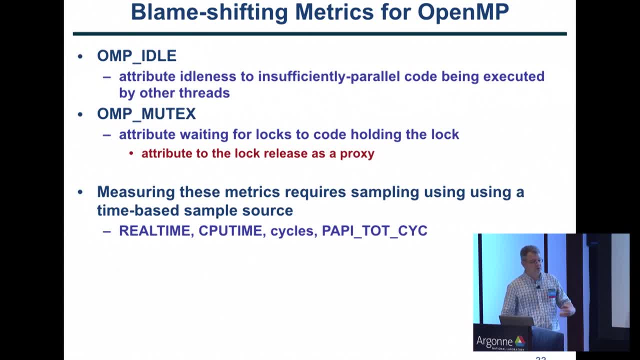 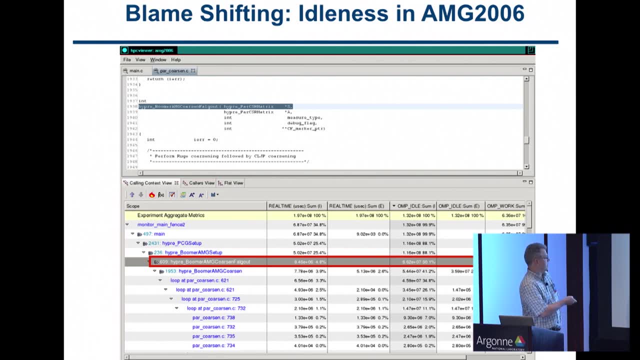 that you can try today, and there's some more directions in here on how to do that. We can measure hardware counters using Linux perf events on Theta with frequency-based sampling and hardware event multiplexing, so you can measure lots of metrics all at once. 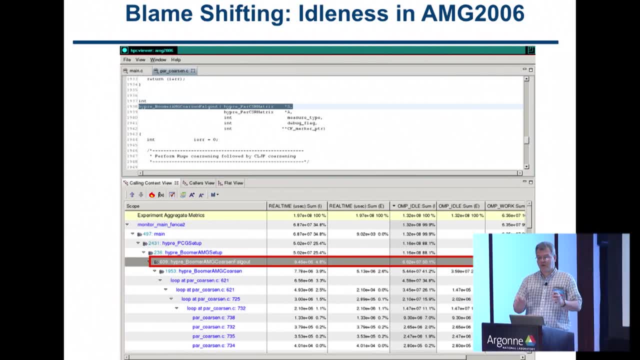 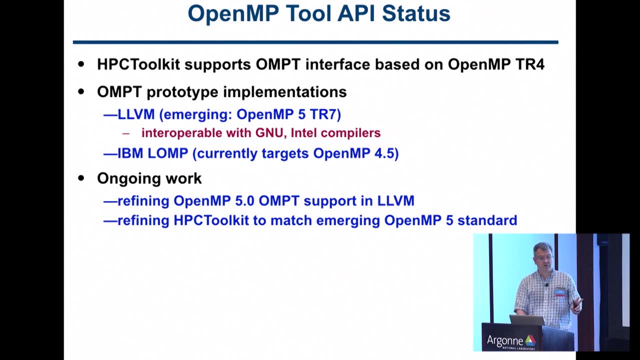 And in fact we can also sample activity in the kernel on the platforms. at Argonne that's not so easy, but on other platforms you can, And so some of the ongoing work we have are improving support for measuring GPU-accelerated nodes. 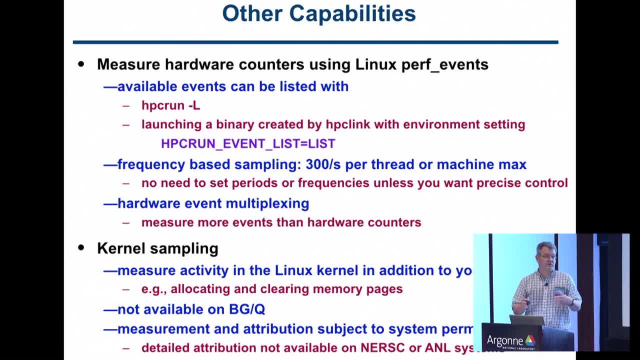 We can attribute costs for code executing on the GPU back to full calling contexts, associating costs with data and some more automation of analysis to deliver performance insights. I'd be happy to answer a couple of questions. Yes, How do we generate the HBC tree? 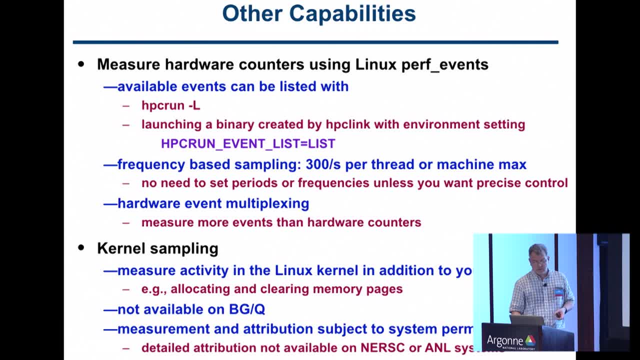 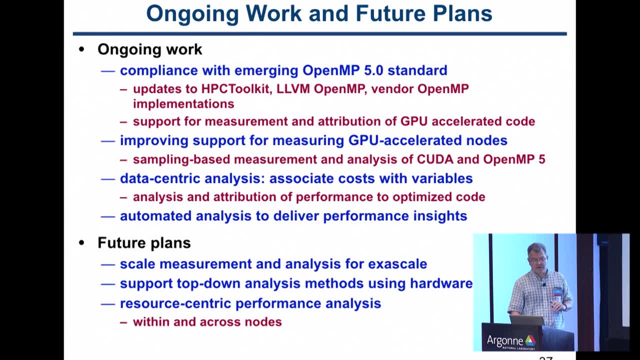 Is it similar to doing HBC view on the output of HBC prof. or is it So? what you do is when you say, When you run the code, you'll either say HBC, run your application, or you use the environment variables. 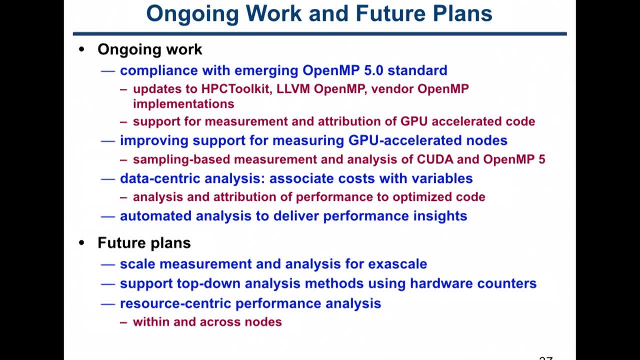 if you have a statically linked application, okay. And so when you Let's say, I wanted to sample using time, okay, So I could sample, say my event is real time, and then I say, dash T, collect a trace along with that. 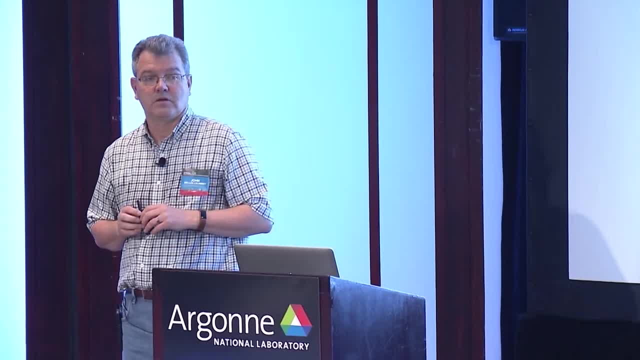 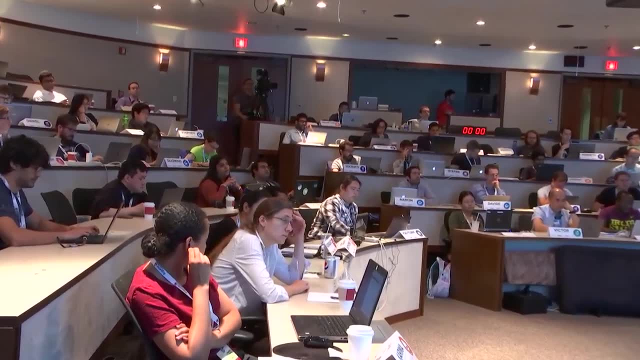 And so what we're collecting is a trace of samples, And you might think that this is a lot of data, but it's only about 12 bytes per sample, because what we're finding out is that at time T, we're at node 17 in this tree. 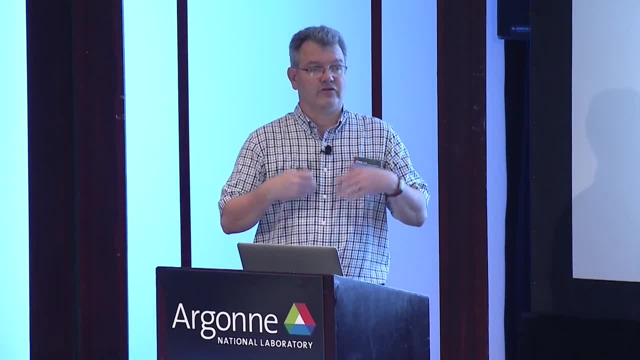 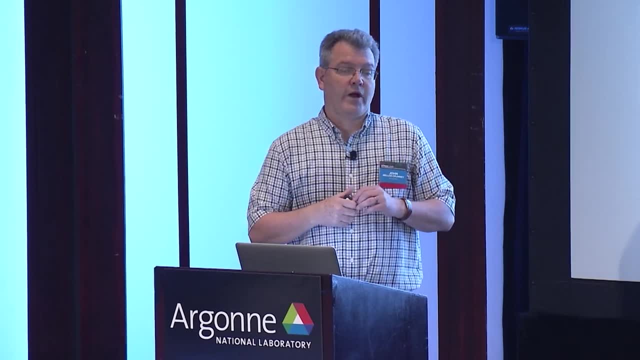 and that implies the whole path to root. So all we need is like the node number and the time, And so you get that by just saying dash T with whatever else you're measuring, and it will collect the trace automatically When you run HBCPROF MPI. 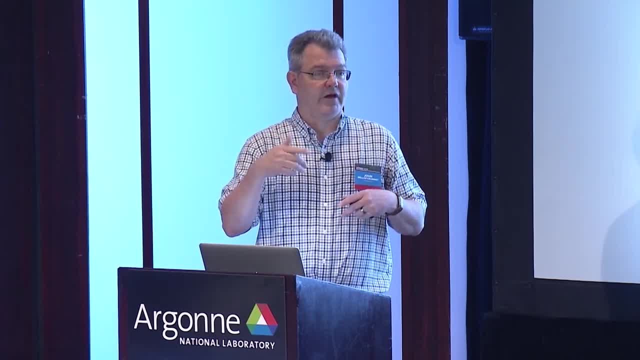 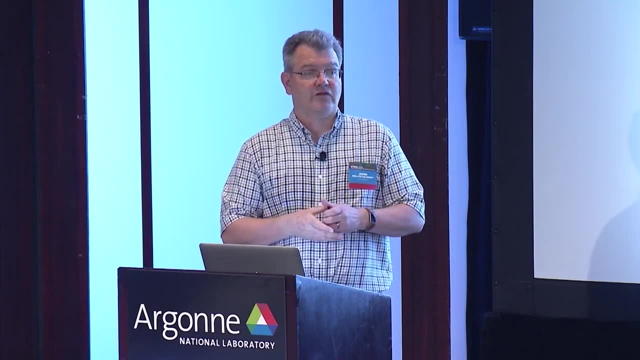 it will produce both the source code-oriented view and the trace-oriented view. okay, And then you just visualize that with HBCTraceViewer. Yes, I've seen that when I use HBCView, HBCPROF, I also get calls to the MPI calls in my code. 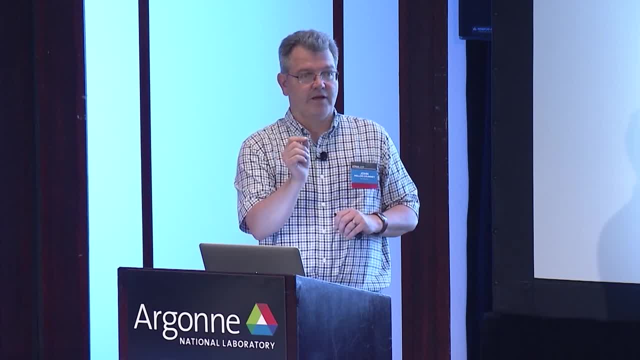 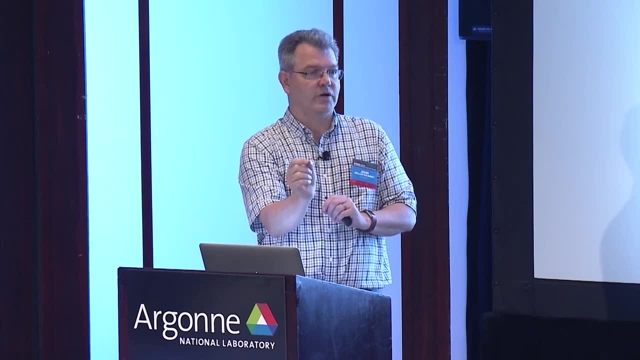 So what is the difference between HBCPROF and HBCPROF MPI? So the only thing, The only difference is HBCPROF is for analyzing small amounts of data. But if you run, If you run something on, say, theta. 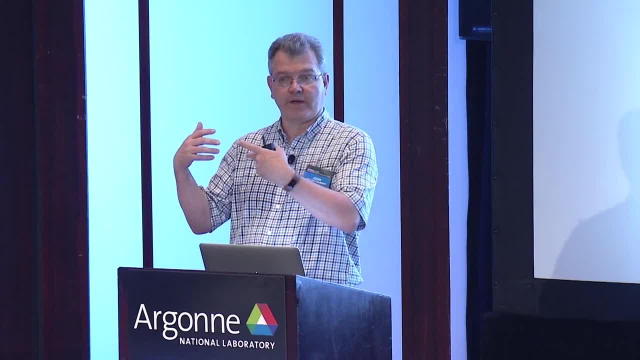 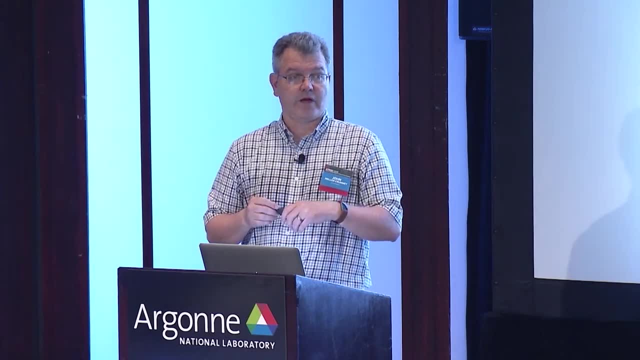 and you collect data on 100 nodes, on 20 threads. you don't want to analyze that all sequentially, So you launch HBCPROF MPI exactly the way you would launch HBCPROF, but you launch it using your MPI launcher. okay, 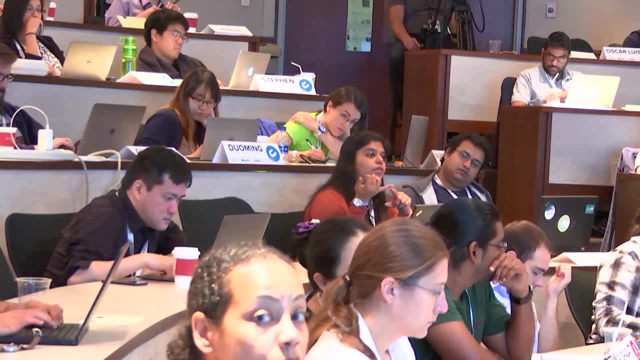 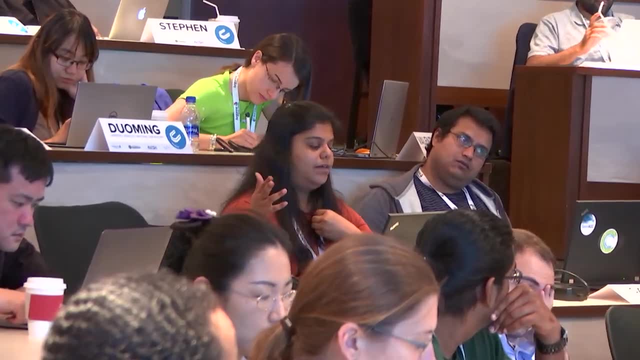 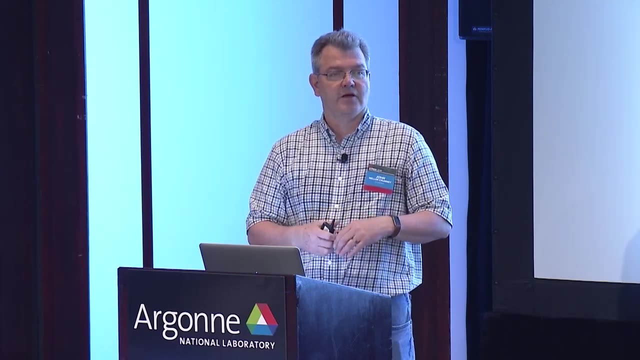 And then it's going to run on the compute nodes of the cluster and analyze all the performance data faster, Okay, Other questions: Yes. Do you have any tools to analyze data movement, like cache misses, So you can say: I want a sample based on cache misses? 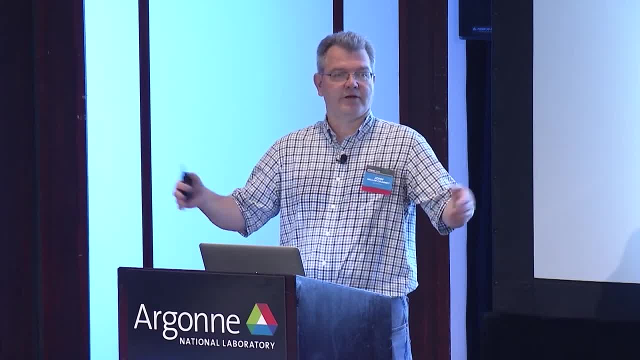 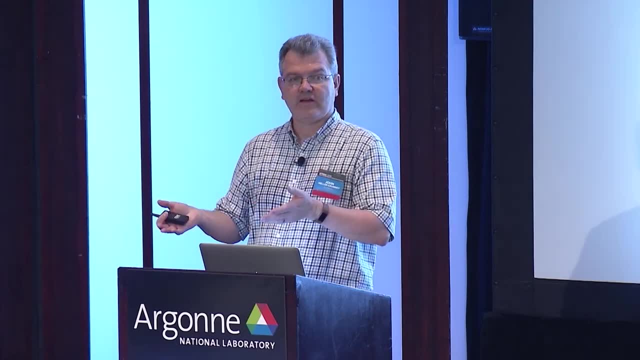 and that just comes up as one of the metric columns. So cache misses work the same way as time. Okay, Yes, I've encountered issues in the past using some debuggers where behavior of some MPI calls would change depending on where I put my breakpoints. 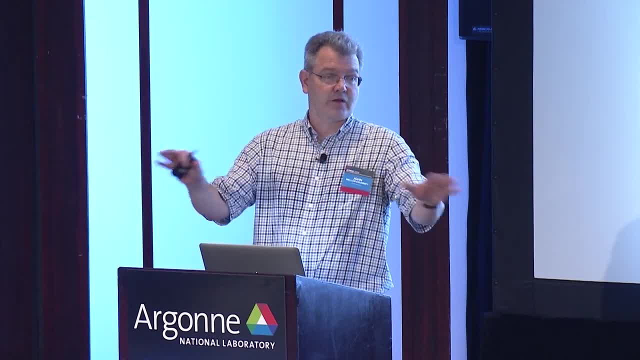 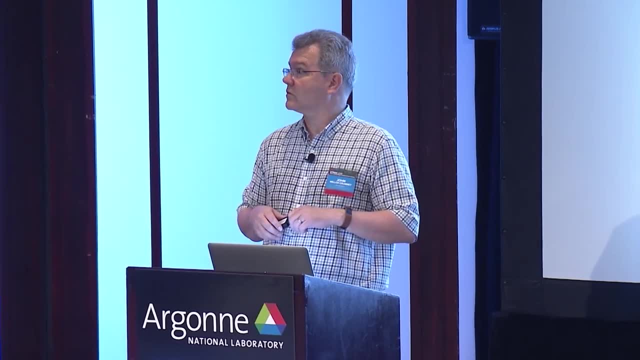 And I wonder, with these, With sampling, you know, in the middle of an execution, have you observed anything quite like that? or is that a risk at all, something I should be considering? So let's just say it's not supposed to happen. 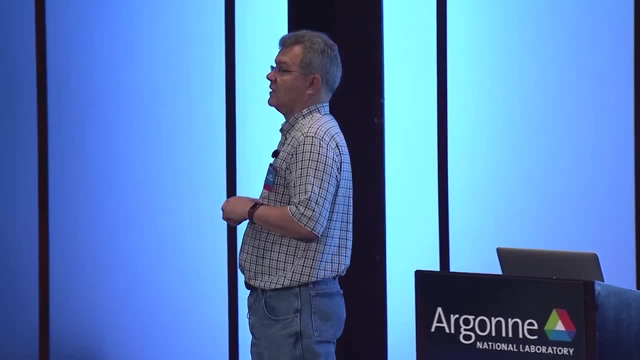 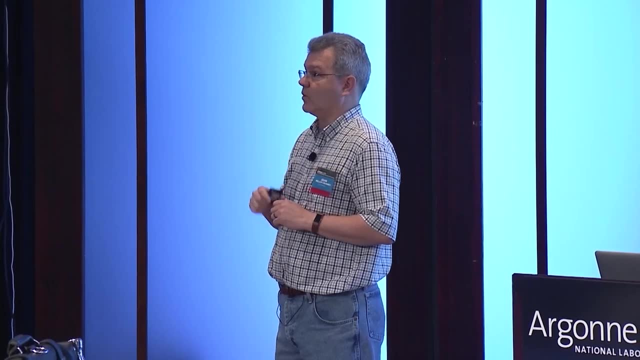 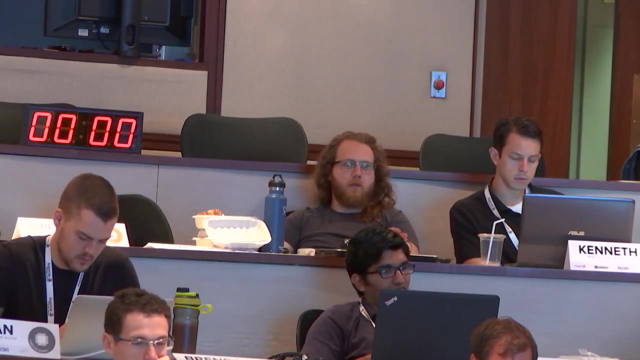 Okay, It's not supposed to be any different, However, for MIRA. when IBM delivered the software stack for MIRA, it turned out that they had race conditions in their PAMI MPI layer, And so anytime you were in PAMI multicast. 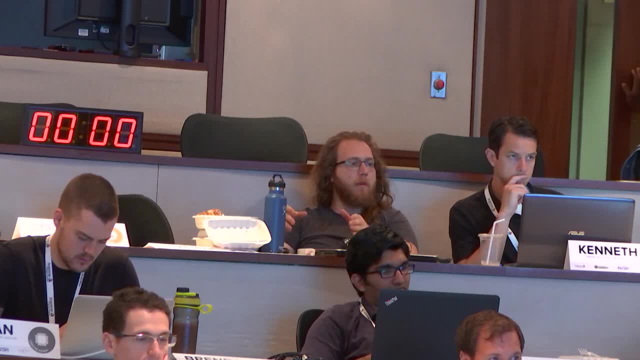 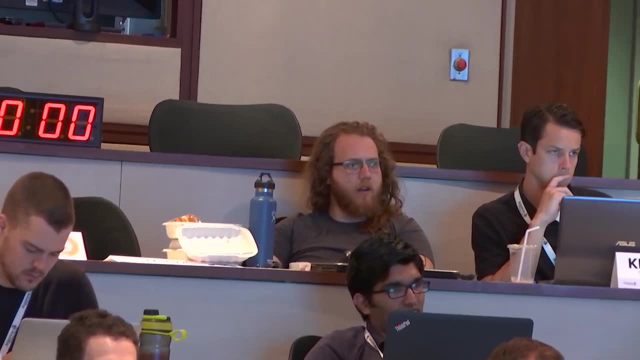 if we interrupted it with sampling we could disturb the race conditions and it would break. That's not supposed to happen. So we spent some time with IBM figuring out exactly what the problem was and we fixed it for PAMI multicast. It turns out there may be other problems in there. 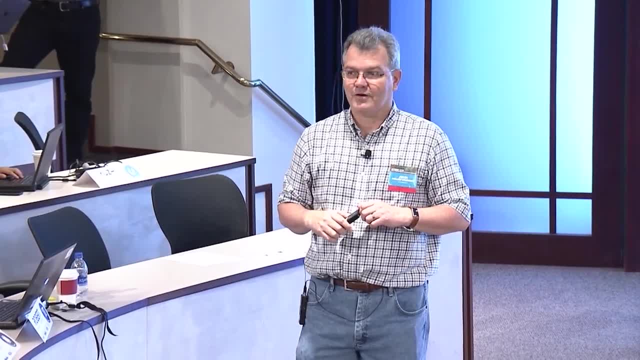 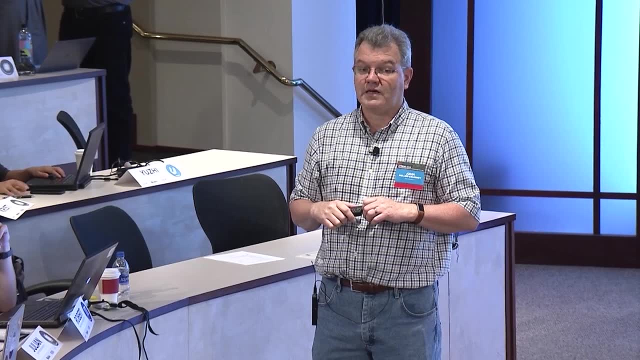 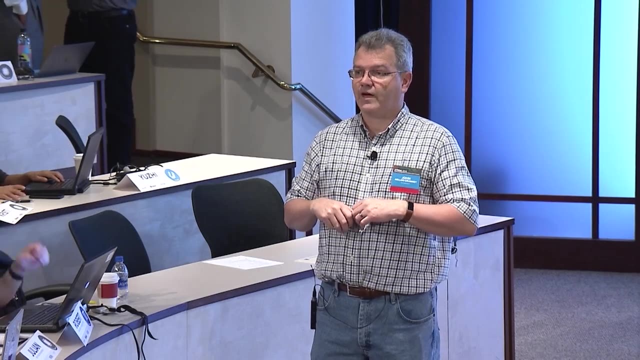 So one of the pieces of advice is you can turn off IBM's optimized but incorrect collectives using an environment variable that says: run the slower version because it's safe. So sampling is not supposed to make any changes to your program If your program is incorrect. 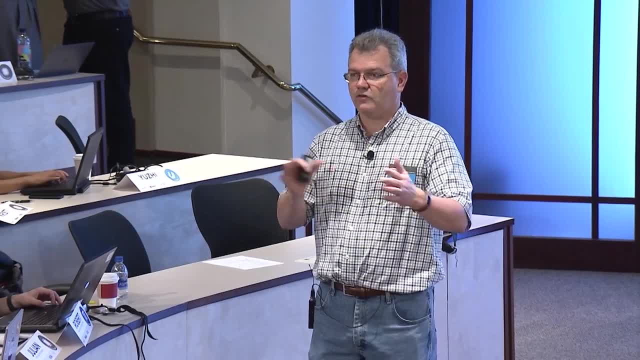 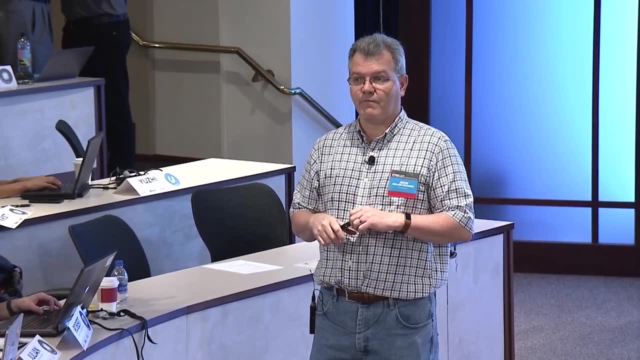 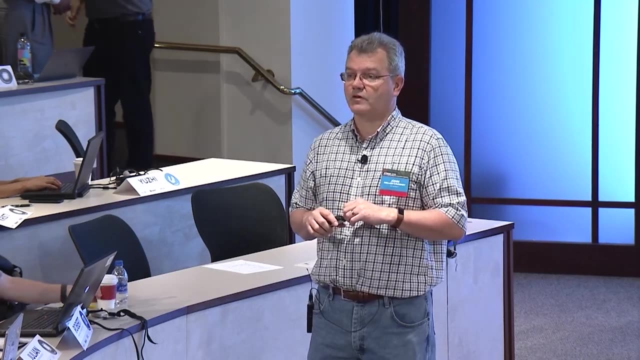 it can expose race conditions in it, and we've seen that with IBM's MPI. Okay, Yes, When you div the call trees to get, for example, at the parallel efficiency, do you deal with differences at the call trees somehow? Absolutely. 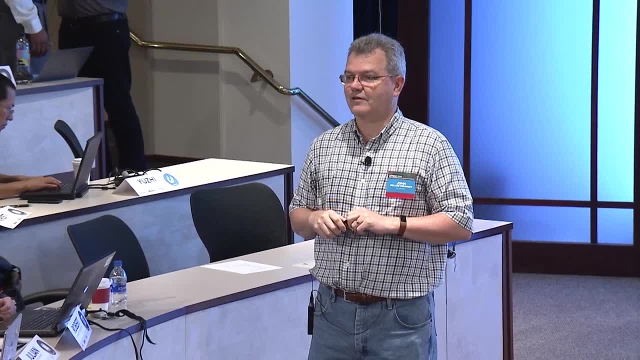 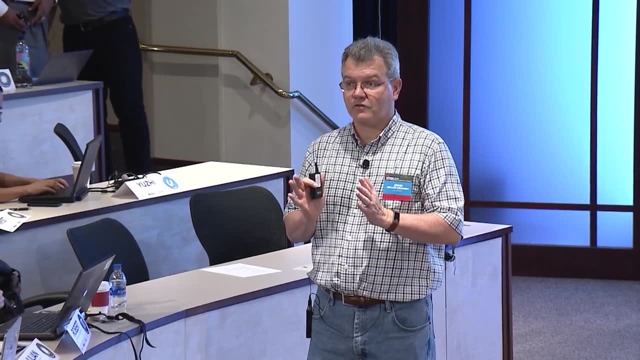 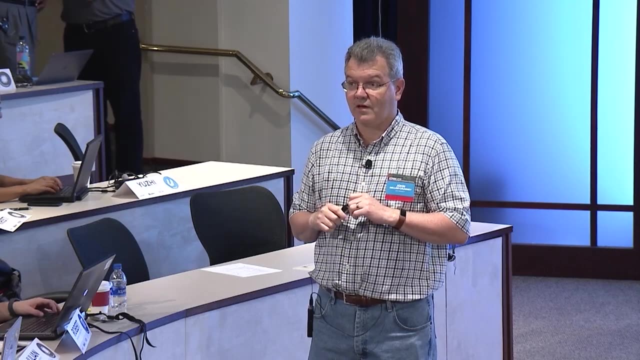 So, in fact, when you run on different problem sizes, in fact your call trees might be slightly different, because you may even have cases that says, well, if it's this problem size, maybe if my matrices are large enough, then I use some other strategy for solving them. 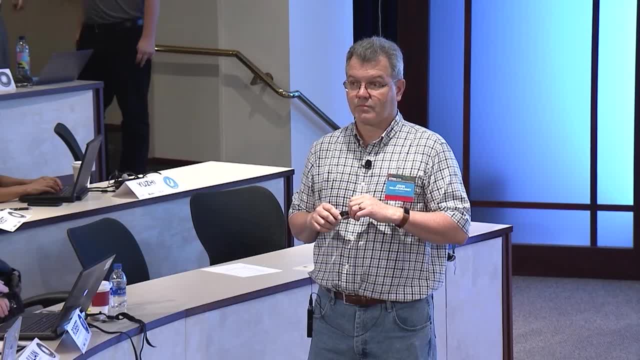 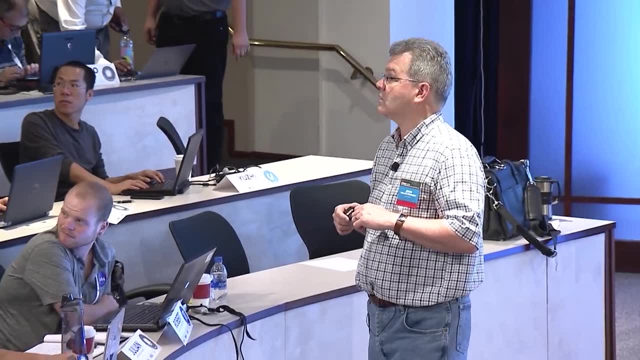 And so that will show up in the differences. but it's most useful if you're using the same algorithm for both, because otherwise it will show up as there was none of it in this tree and there was a lot of it in that tree.